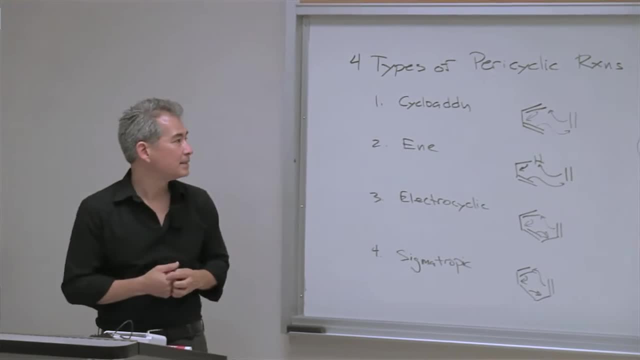 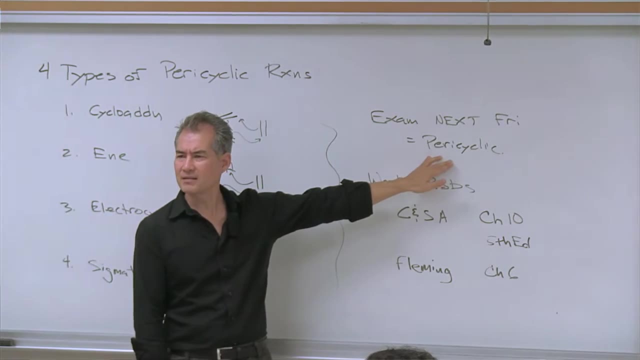 we have to have at least one sigma bond in the transition state that's participating. Our exam is next Friday. It's going to cover all paracyclic reactions, so we should be able to finish that on Friday. So we'll be done with that And let me encourage you to work. 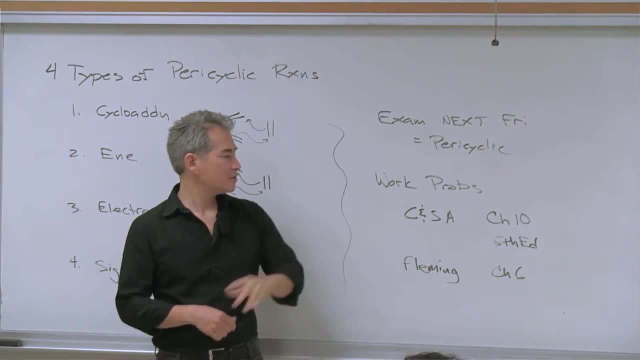 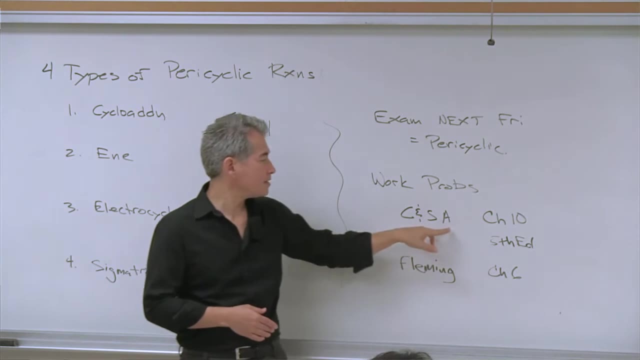 problems, not just the problems on the problem set, But there's two books. There's two books that are useful for this class. This Fleming book, Chapter 6, is all paracyclic reactions and there's bunches of problems in the back. Carrion-Sundberg Part. 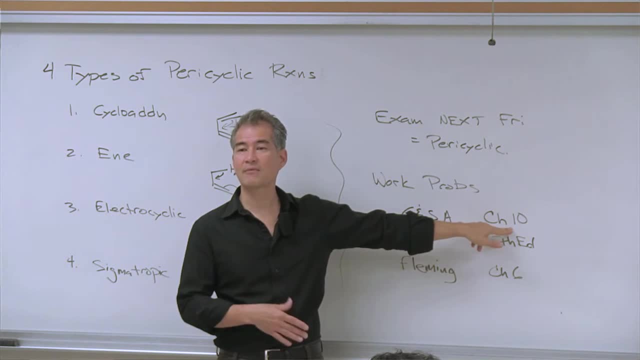 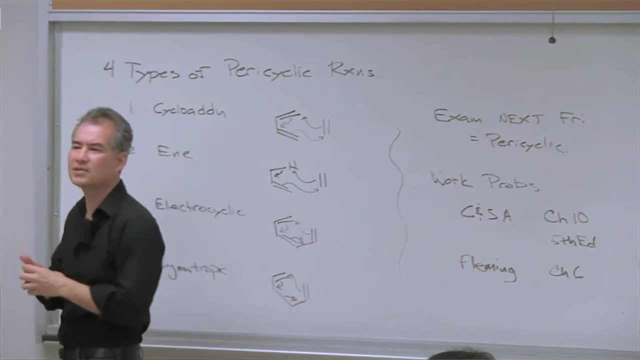 A. In the fifth edition, chapter 10 is all paracyclic reactions and the end of the chapter is full of problems. The fourth edition is online. Chapter 11 in the fourth edition is paracyclic reactions. So work those problems. Work as many problems as you can get your. 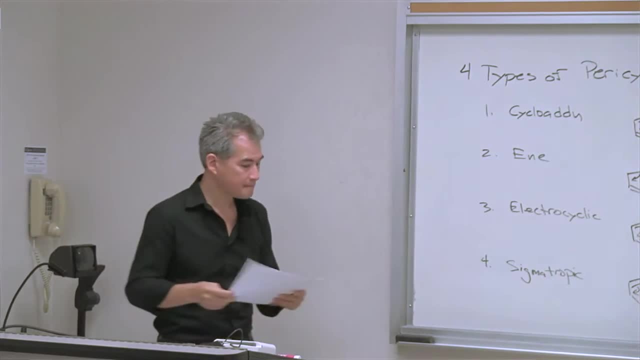 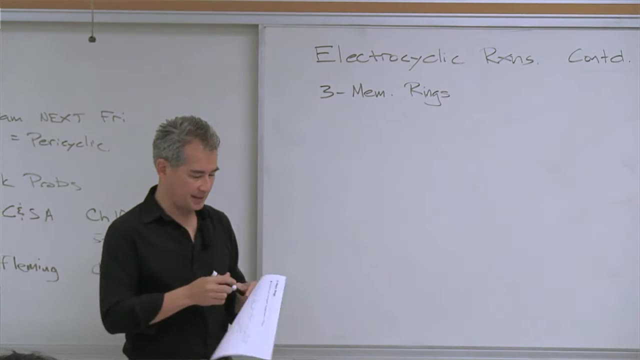 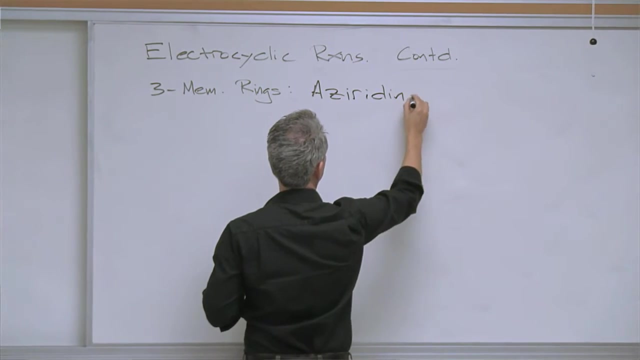 hands on, not just the problems, on the problem set. So let's keep talking about electrocyclic reactions And we'll talk about three-membered rings And in particular, we're going to talk about aziridines, Three-membered rings containing nitrogen, because there's a lone pair on the. 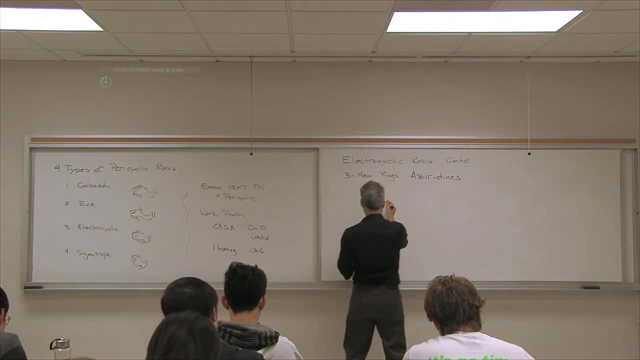 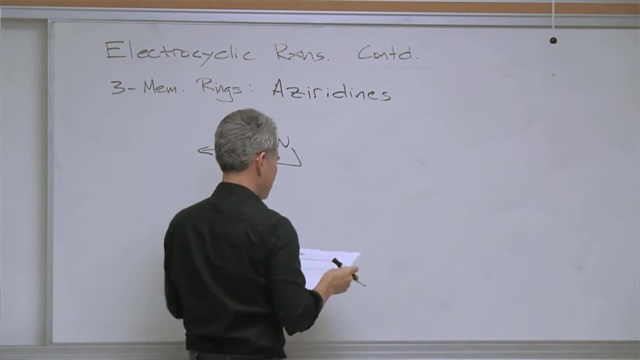 nitrogen atom that can participate. So I'm going to- I'll try to draw a structure of aziridine and I'll give it two choices going left and right here. So here's just a basic aziridine structure. Aziridine is: 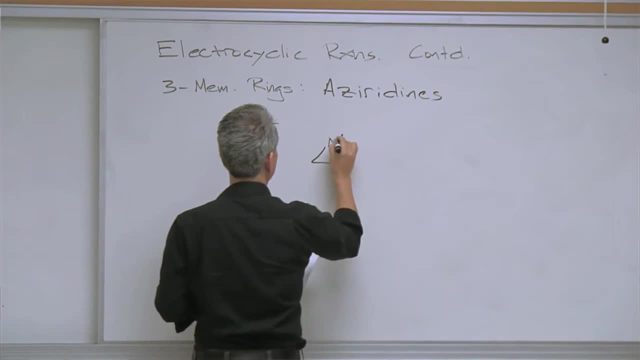 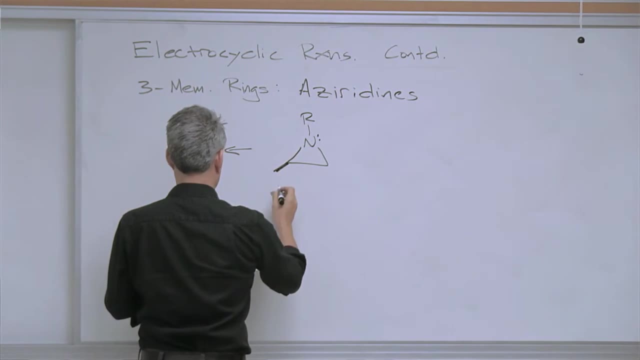 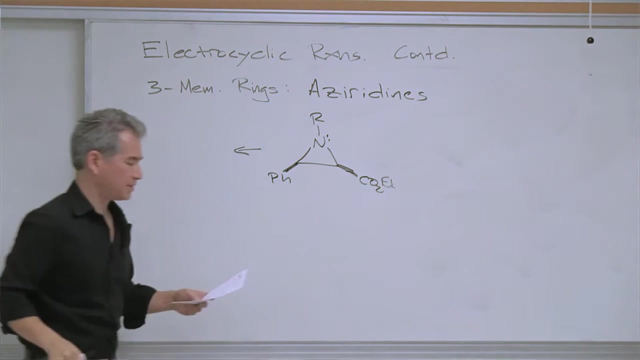 like an epoxide Good, And there's a lone pair here on nitrogen R group is not so important here And I'm going to put two substituents here on this aziridine ring: an arene and an ester. 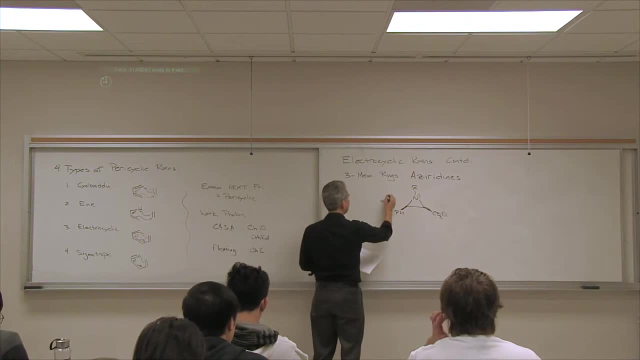 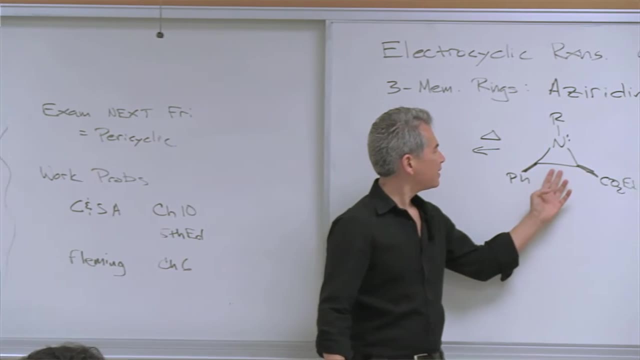 And we can track these choices here. So if we simply heat this, this can engage in an electrocyclic ring opening reaction. So we've got a sigma bond, And if we flatten this out, then this can be hybridized like a p-orbital. 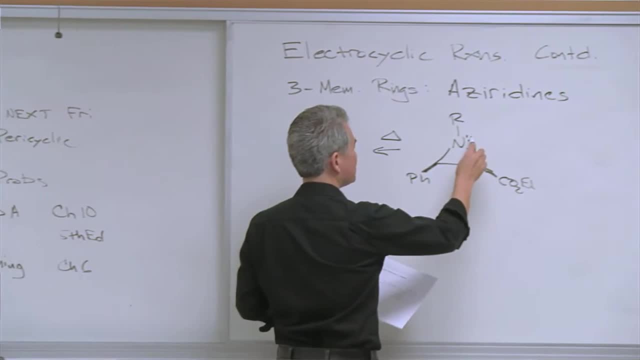 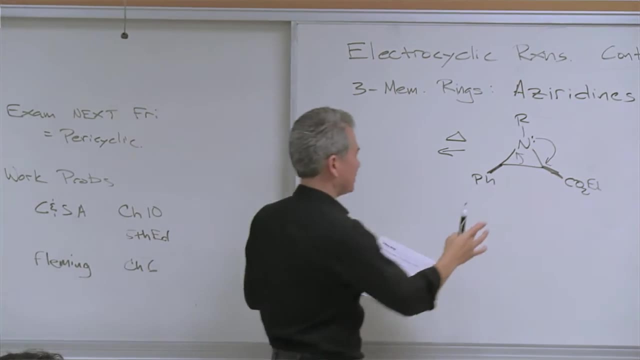 That can be like a pi system. So if we make this lone pair participate, it can donate into this antibonding orbital, weaken this bond And we can bring this over in order to make actually- let me push the arrows in another- the opposite way. 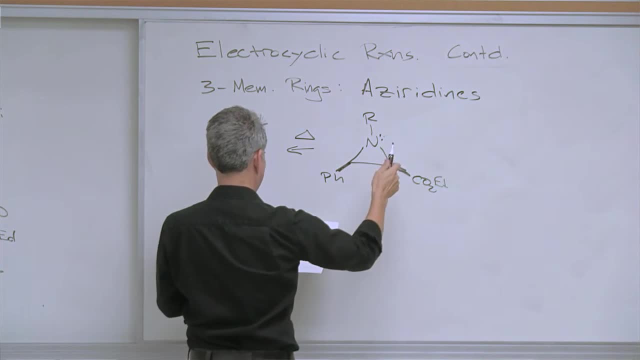 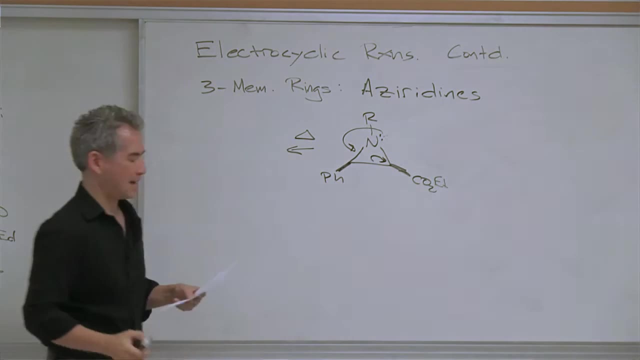 I apologize for that if you've already drawn that, Because I want to make it match my next structure. Let me push the arrows this way And I'll leave the electrocyclic And I'll leave the electrons here on this carbon atom. 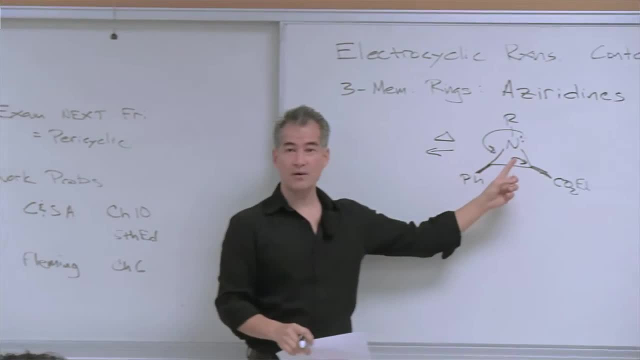 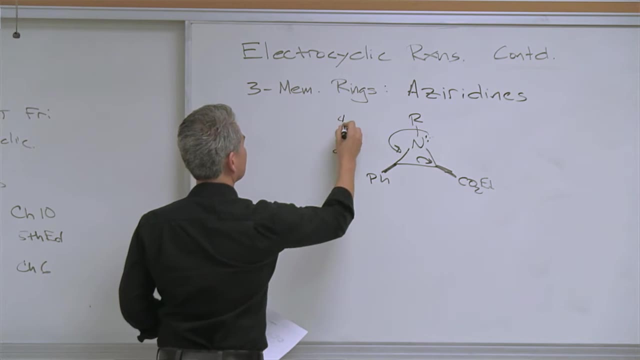 And that'll give me the resonance structures that I drew. So I've got two arrows. There's four electrons in the transition state, Two electrons per arrow. So if it's four electrons, is that conrotatory or disrotatory? It's conrotatory. 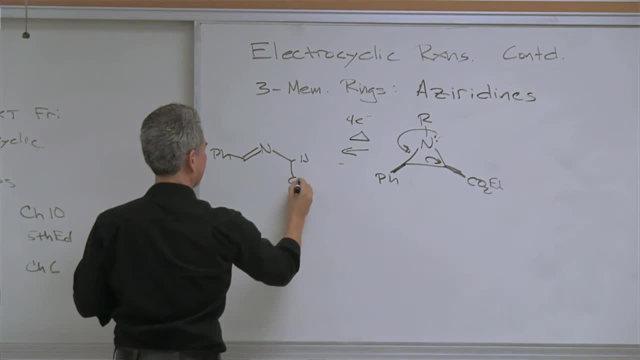 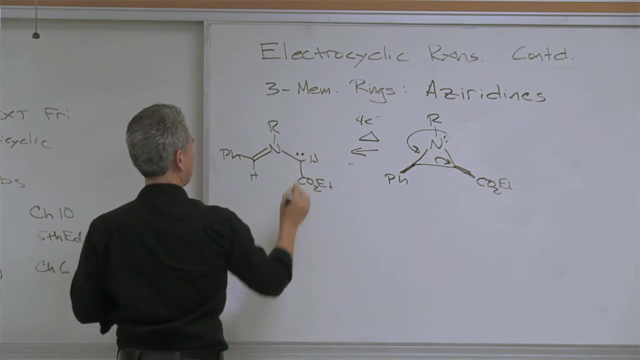 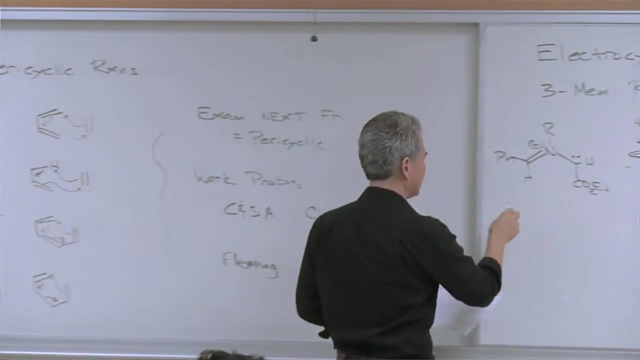 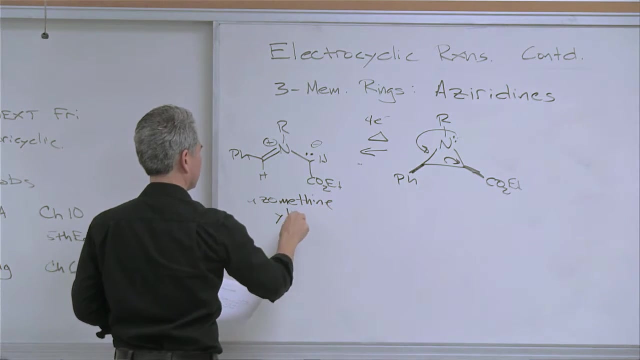 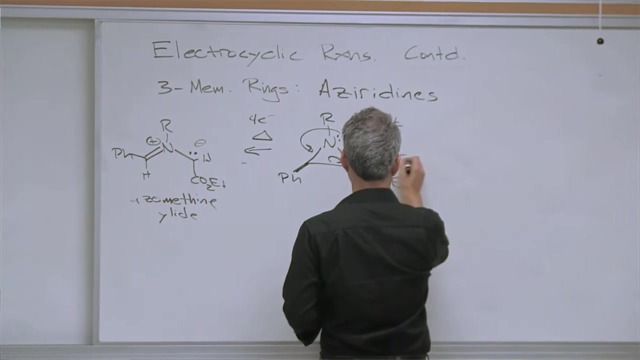 And I better make it conrotatory. It's metallic, And so you get this yIt structure. This is called an azomethyne, And azomethyne can do three plus two disposition reactions. You can also treat these with light. 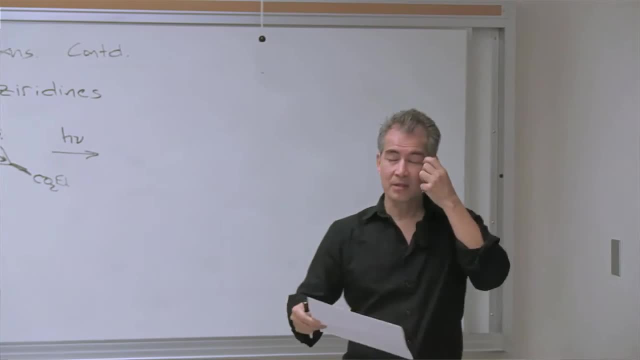 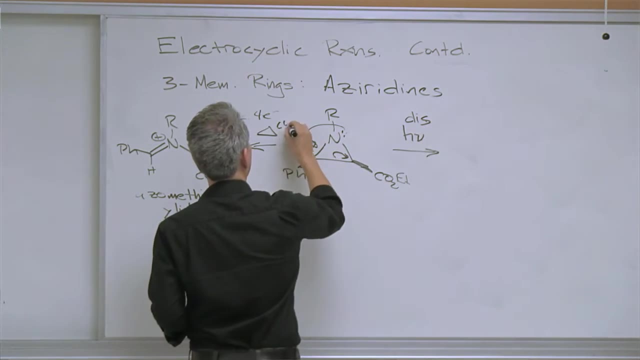 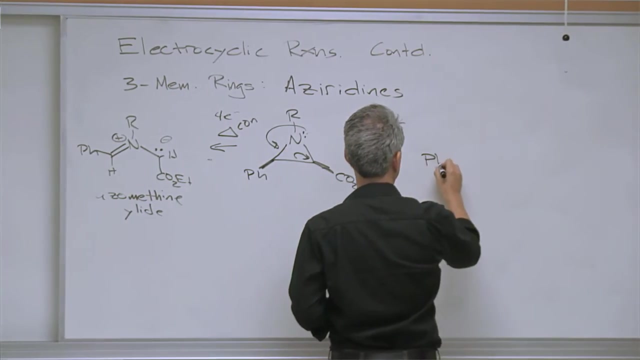 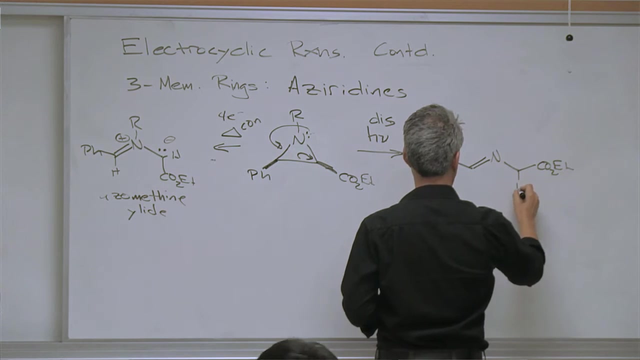 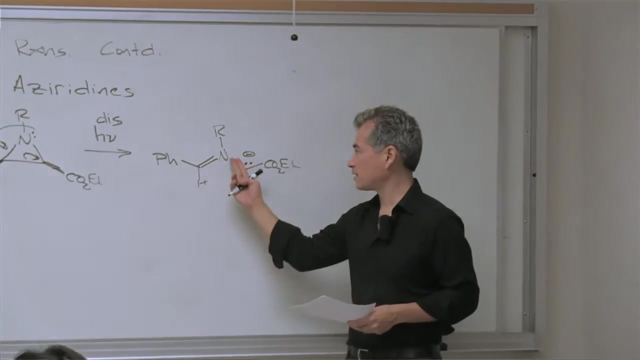 And you can reverse the paracyclic selection selection rules. so if heating it gives you con rotatory ring opening, I'll just write con here- then under photochemical conditions you would expect that this would give you dis rotatory ring opening, and so I I'm not going to draw the other resonance structure there, but there's. 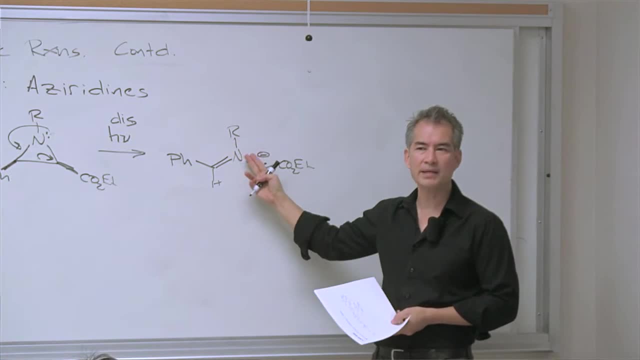 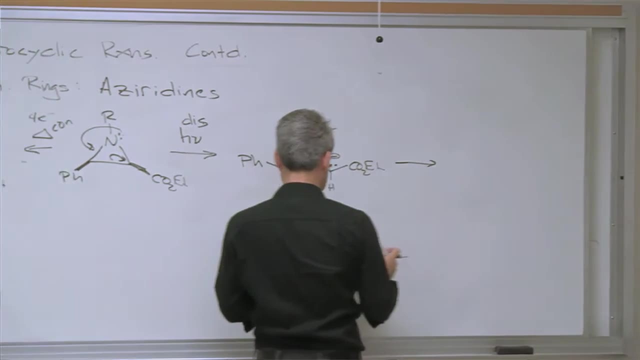 partial double bond character here between this carbon and nitrogen. that kind of gives you the equivalent of E and Z geometry. so in the presence of, I'll go ahead and draw down here if you put in some sort of a diagram. I'll go ahead and draw down here if you put in some sort of a diagram. 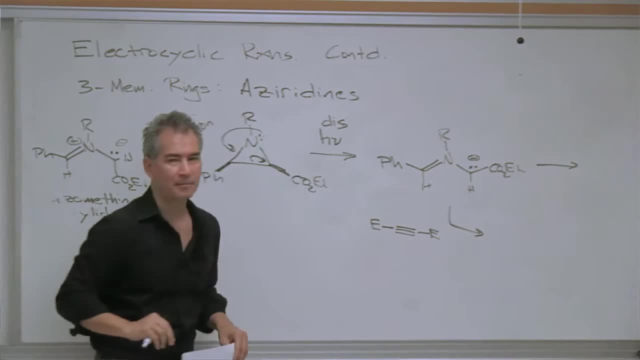 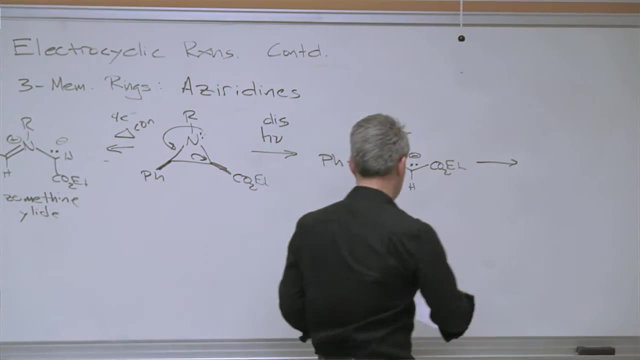 diagram: dipolarophile like dimethylacetylene to dicarboxylate, some sort of an activated. this is very nucleophilic. this azomethanolide, If I put in an electrophilic dipolarophile you can get 3 plus 2 cycloaddition. 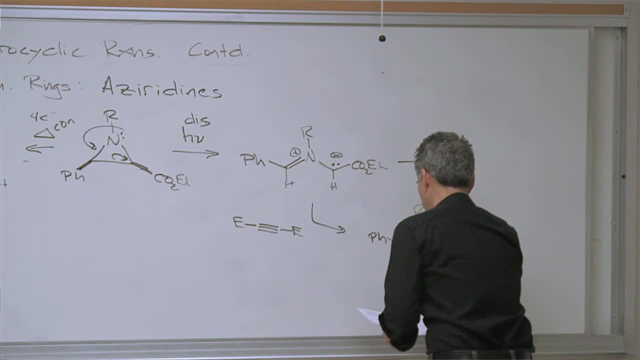 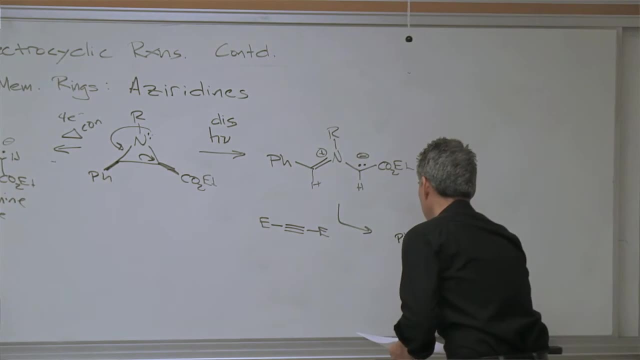 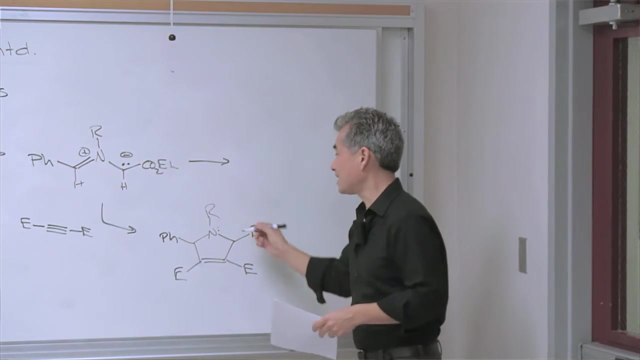 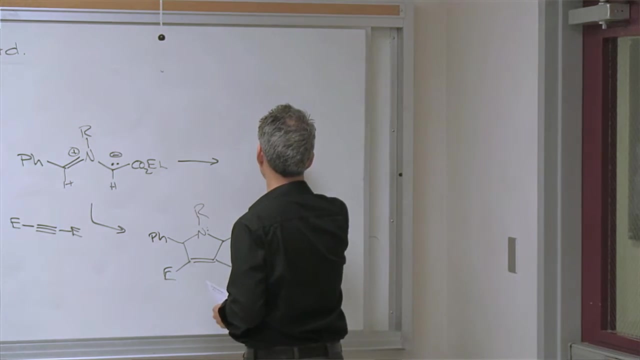 reactions to it. I'll just put E for ester here, And so you can generate five membered reactions, So two paracyclic reactions. This, it turns out, is not stable and it will tautomerize With all of these carbonyls. the double bond wants to be more in conjugation with the nitrogen. 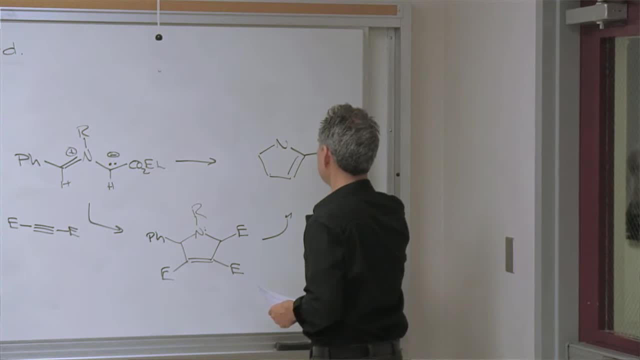 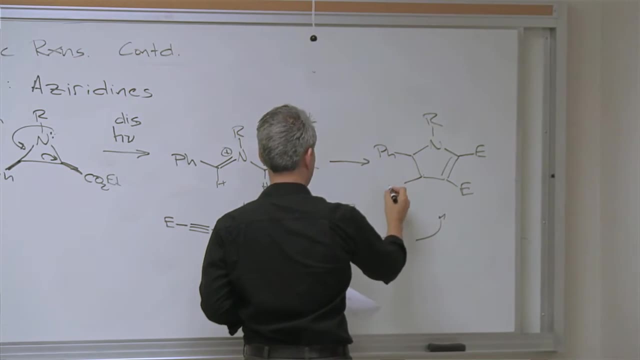 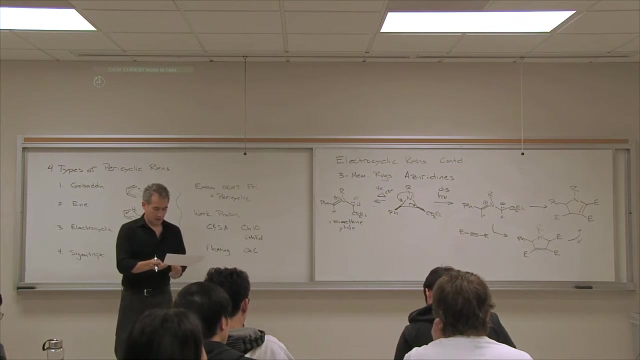 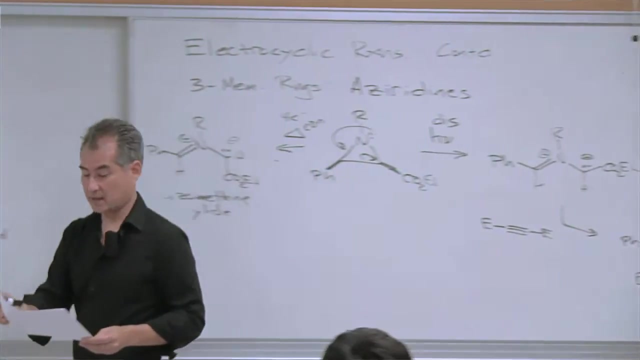 lone pair and a carbonyl, And so it's not really that interesting from the standpoint of paracyclic reactions. but this will tautomerize to an enamine. Oh, actually, I've got that tautomerization on the wrong side, Sorry Over here. So now even the benzene ring can. be part of that conjugated system. Okay, so three membered rings can ring open through paracyclic processes that are governed by orbital symmetry: disrotatory, conrotatory. Let's take a look at a carbocyclic ring, a cyclopropane ring, 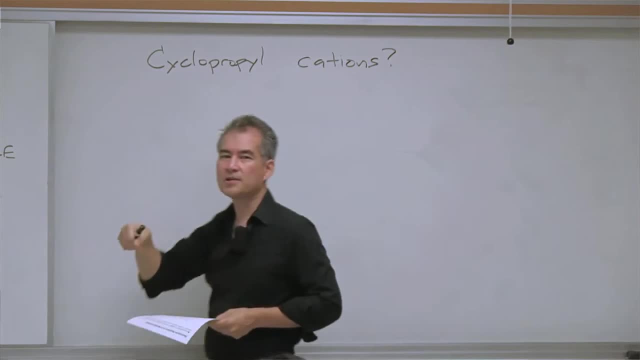 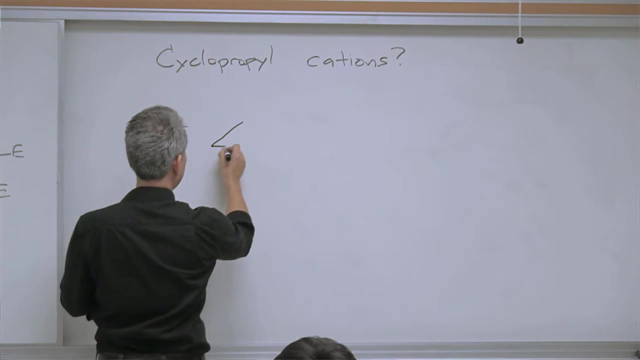 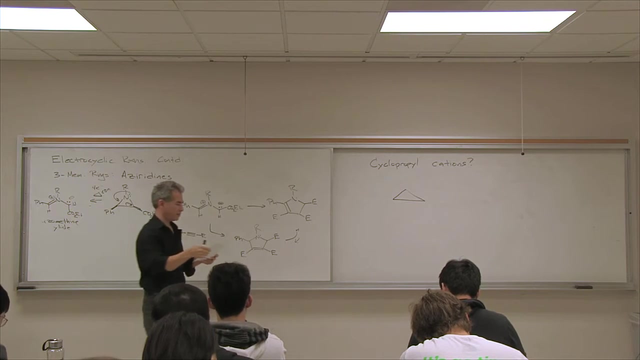 I'll put a question mark there next to cations. I'm going to start off by trying to draw a three membered ring kind of edge on, So we can kind of imagine that way. we can try to imagine substituents above and below the plane of the ring if I draw it in this distorted 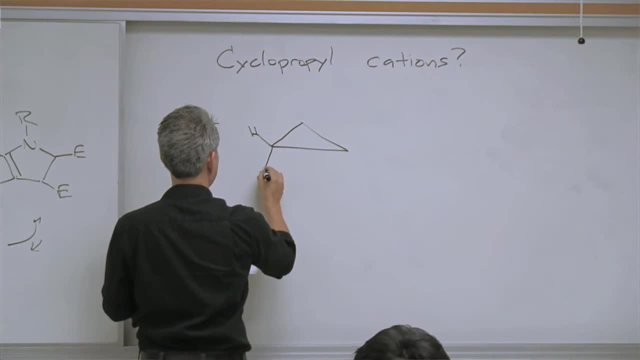 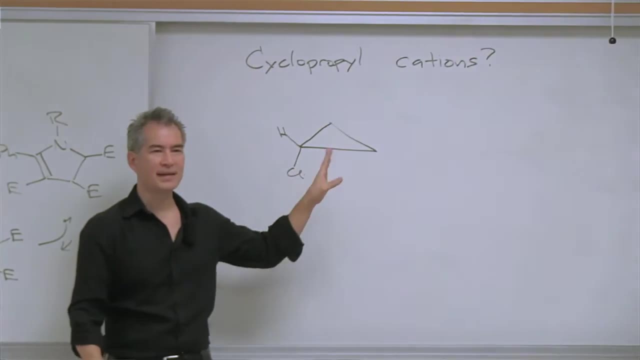 way, And I want to put a leaving group on here so we can imagine what will happen if that chloride pops out to give a cyclopropyl cation. This is not the kind of cyclopropane cation structure you're used to. You're used to carbocations next to cyclopropane rings. 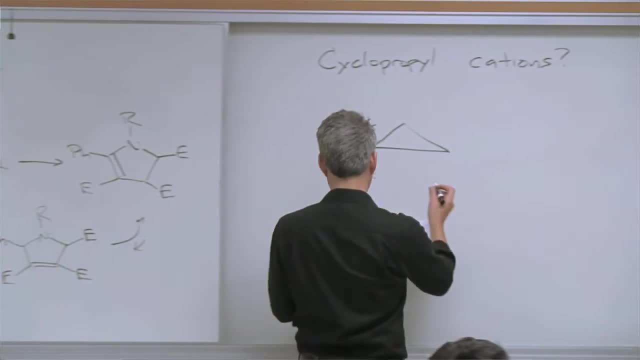 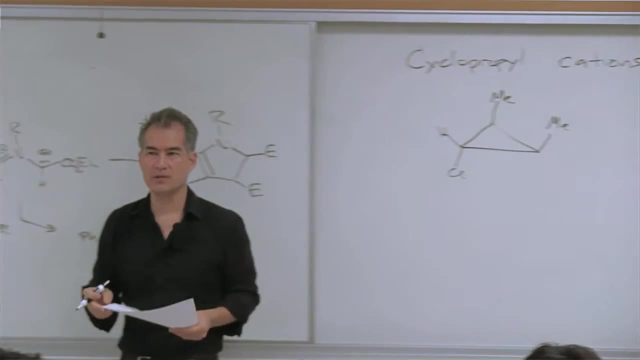 not inside of cyclopropane rings. So if you heat this enough, let me add some substituents. I'm going to add two substituents on the top face so that we can keep track of disrotatory and conrotatory stuff. So I'll put two methyl groups on the top face And then let me try. 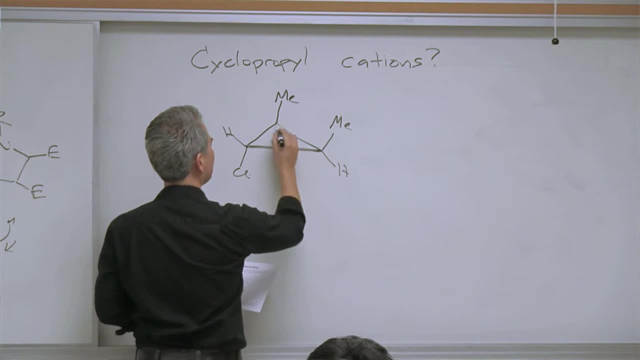 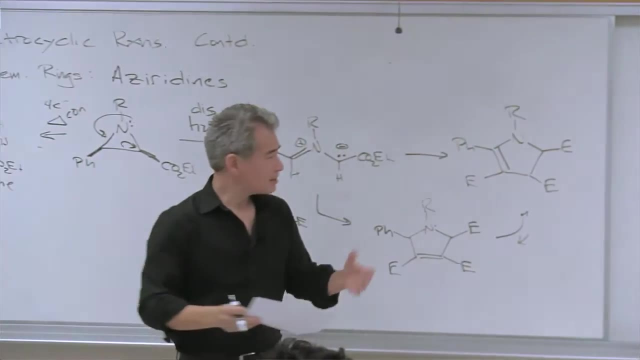 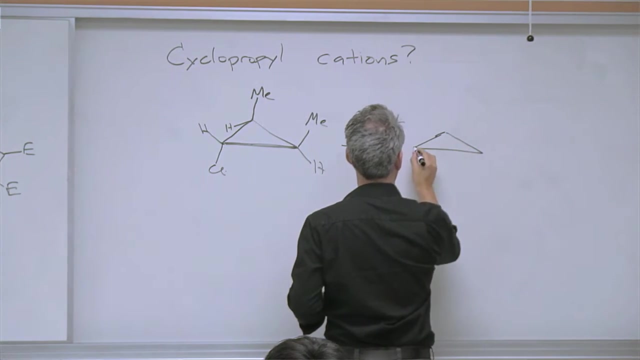 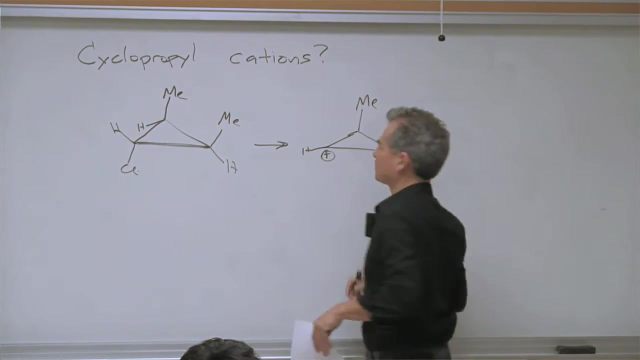 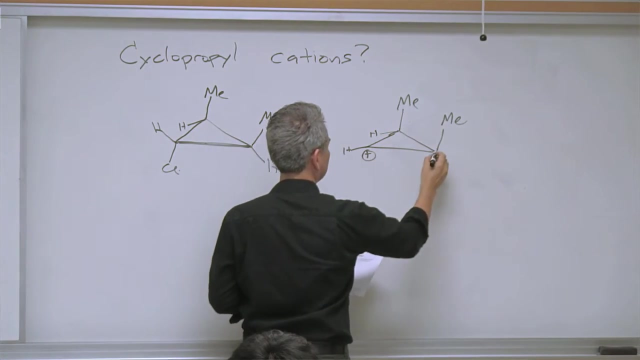 to make this look kind of three dimensional there, And then we'll put some H's on the bottom face of this cyclopropane. Okay, so let's imagine what happens if we ionize to give a carbocation. So now we have an empty p orbital there. And so now if I push the 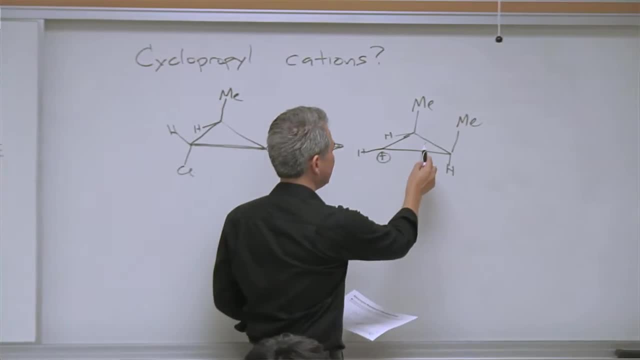 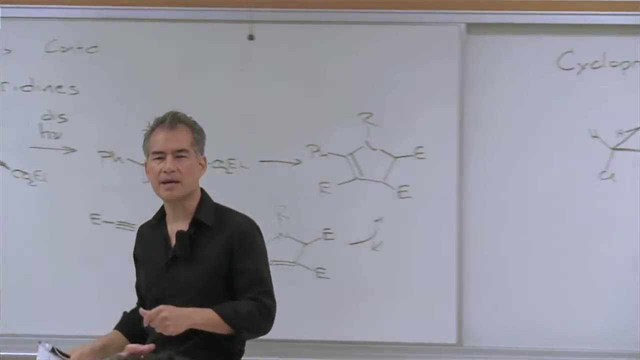 electrons and do some sort of a ring opening. really I've only got one pair of electrons And that's in this bond. It's kind of arbitrary which direction I push that arrow. So there's only two electrons. This is a two electron system. Is this disrotatory or conrotatory? 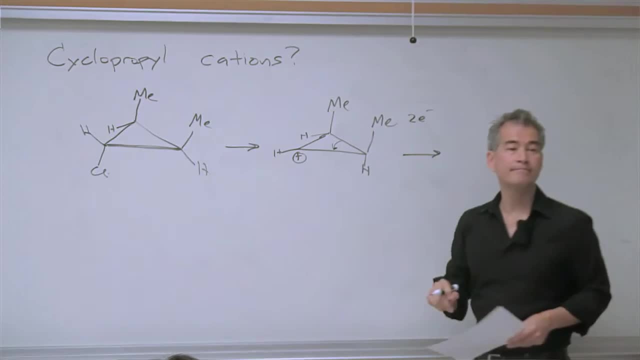 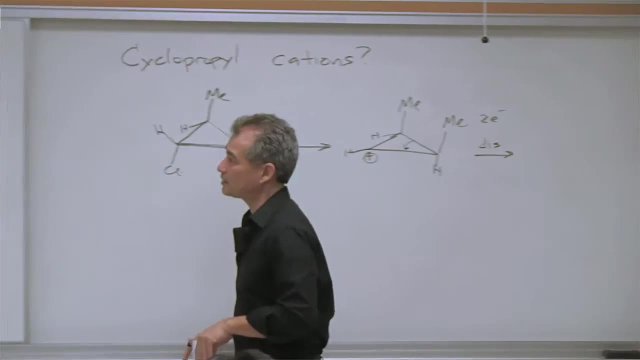 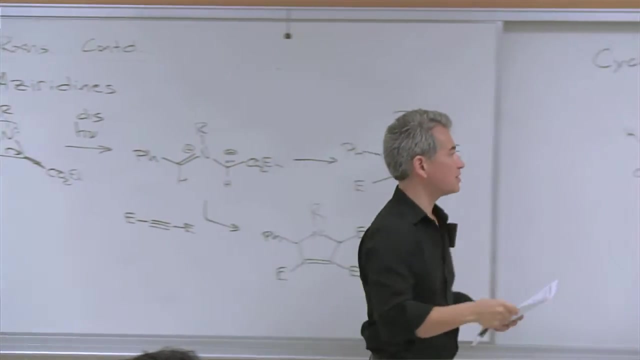 It needs to be disrotatory. So over here with this system, we had a pair of electrons in this orbital. This is a four electron ring opening. The cyclopropyl cation would be a two electron. Okay, This is a two electron system. So if you're simply heating this without light, then you'd 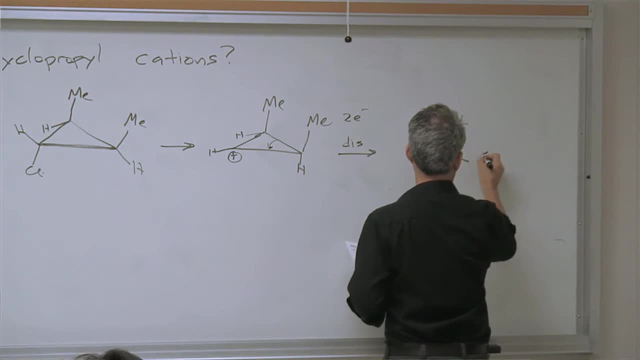 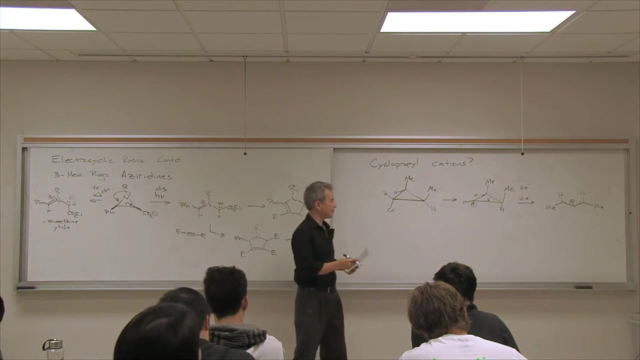 expect this to be disrotatory, And so the product that you get- in this case I'll draw the delocalized structure. It would look like this, which makes sense. That's sterically. that looks actually pretty good. I don't have any big steric issues. What's weird is that. 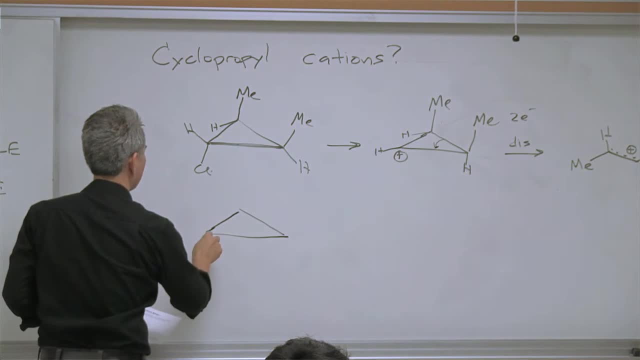 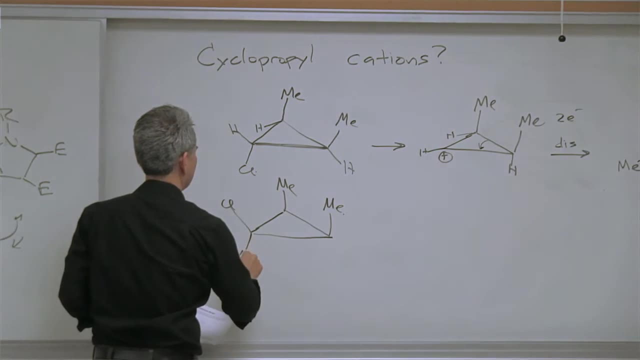 if you take this alternative isomer of this cyclopropane, where the chloride is up on the same face of the methyl groups, who would have thought that there'd be a difference here? right, If this is really the mechanism that I drew- and I'm going to imply that, maybe. 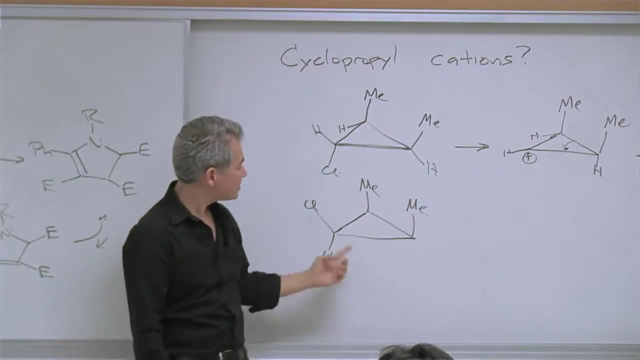 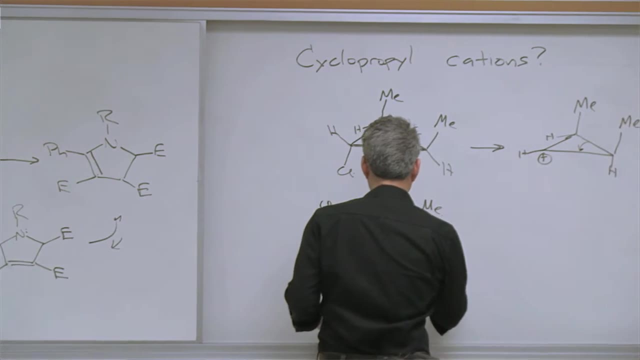 this is not the mechanism. but if this is really the mechanism, that it shouldn't matter which of these two chlorides I start with, because if they ionize, you'll end up with the same carbocation And I'm simply going to tell you I'll draw the product over here. 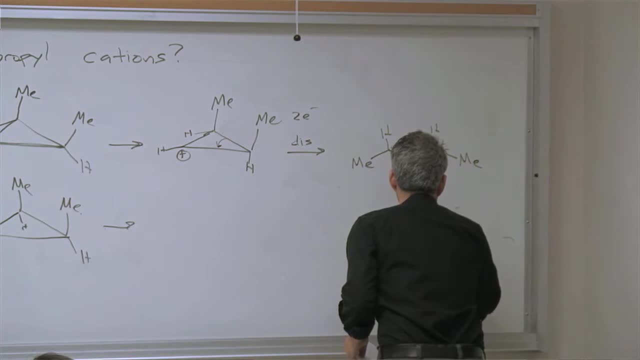 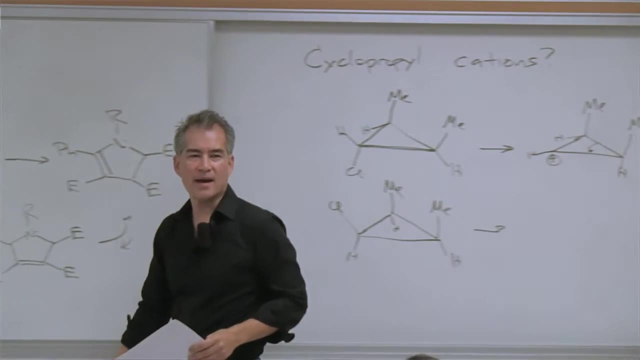 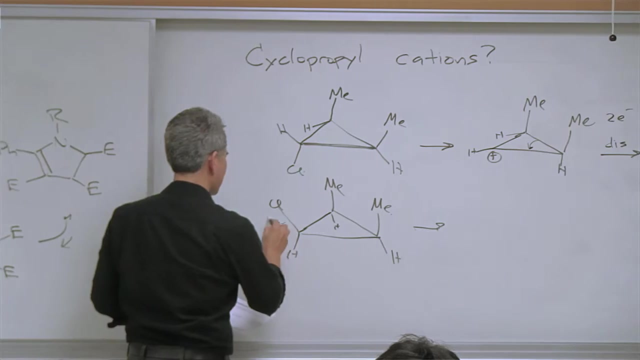 that, oddly, when you start with the other chloride, you get this other allylic carbocation. Why should it matter? It seems like you're generating the same chloride when this leaves. So in order to understand what's going on here, you need to draw out. 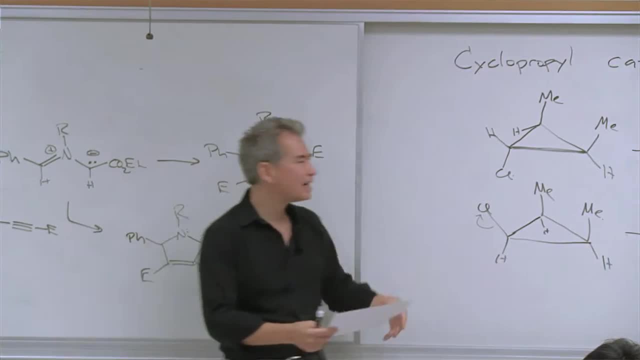 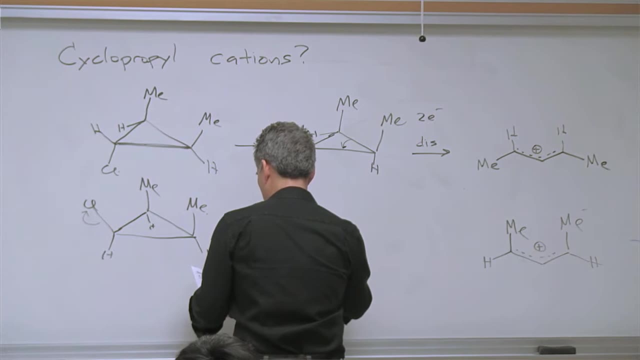 the anti-bonding orbital for this and ask: what is it that makes that chloride leave? So let me go ahead and redraw this structure, And what I'm going to try to do is try to draw this inside. This is some sort of a distorted way that can help me see the tilting of these methyl. 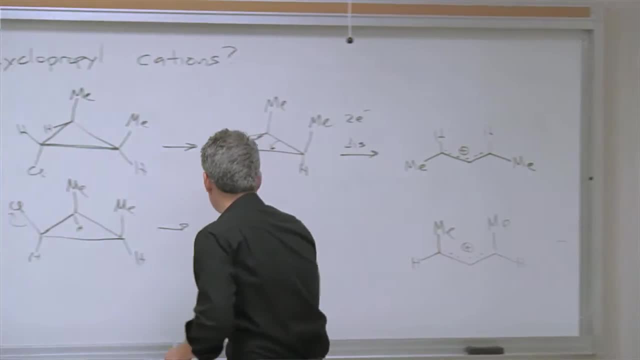 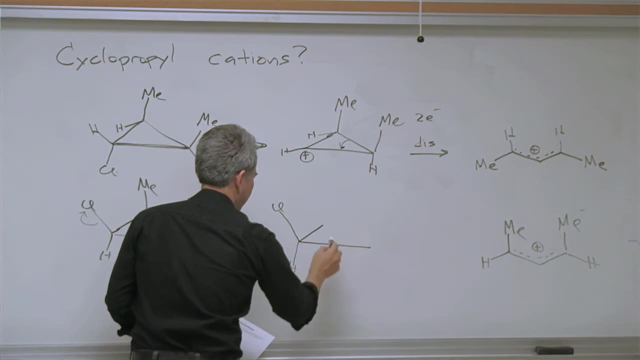 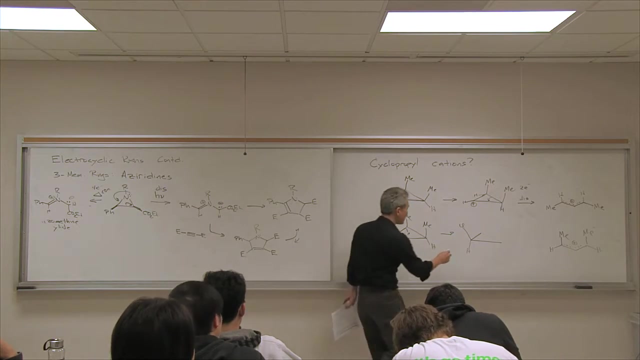 groups. And so let's draw why this chloride leaves. Let's draw this anti-bonding orbital for the carbon-chlorine bond And I'll just sort of lightly sketch in that bond. I want to draw the anti-bonding orbital for the carbon-chlorine bond. Any donation into this anti-bonding? 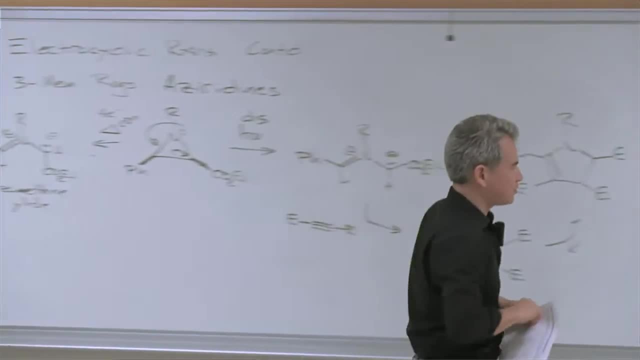 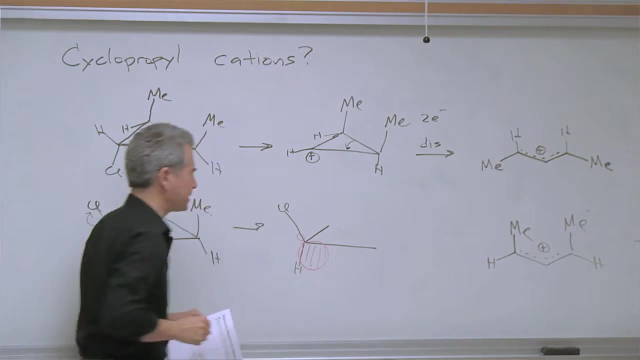 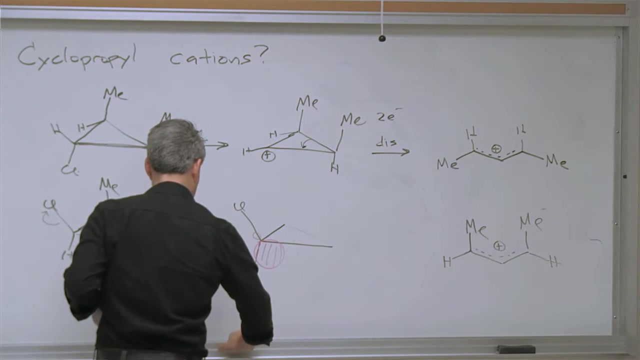 orbital and I'll draw that in brilliant red. Here's the anti-bonding orbital back here. That's my sort of sketch. Anything that donates into that anti-bonding orbital is going to make that carbon-chlorine actually leave with greater facility. So like this It turns out: 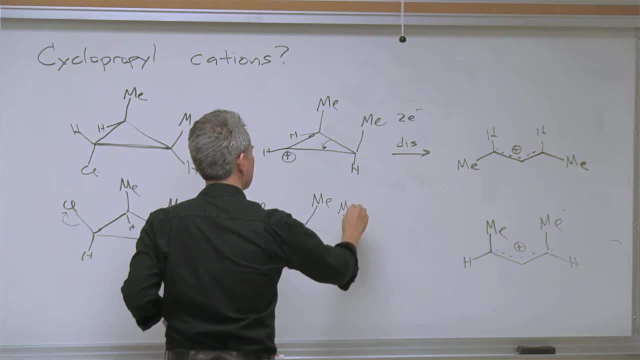 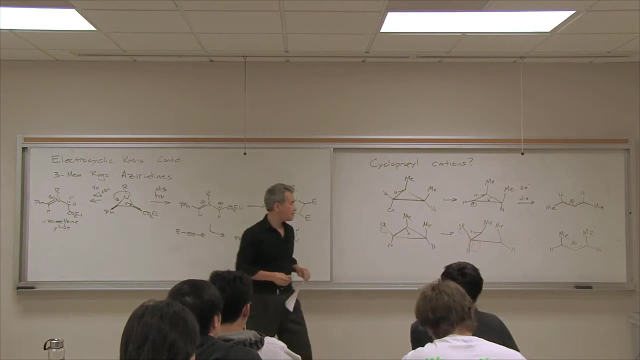 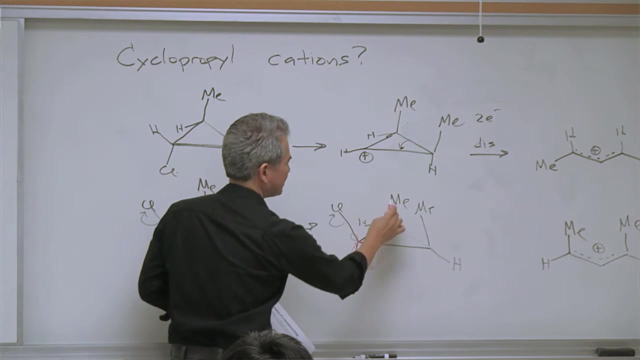 that if you torque these methyl groups inward- and I'm going to try to super distort this in some sort of a freakish way- what happens is this bond starts to torque And I'll try to draw. normally this bond is poking in between these two carbon atoms, but if you distort, 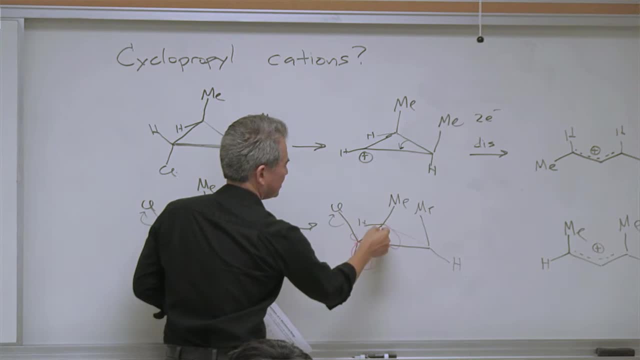 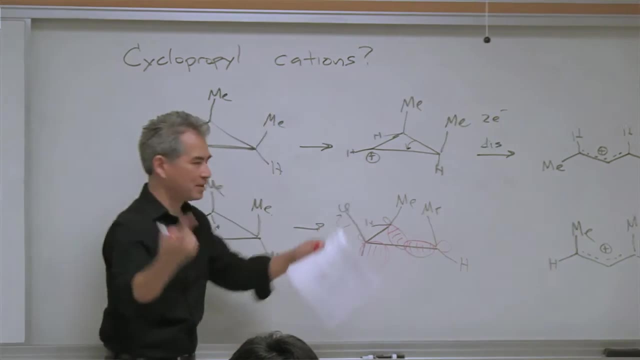 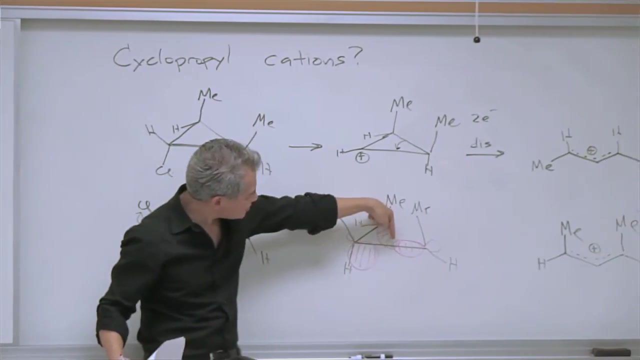 this molecule to twist those methyls inwards, then the orbitals that contribute to formation of that sigma bond will now start to bend downward. So if you twist these methyls inward, this sigma bond will sort of distort downward And that allows the electron density in this. 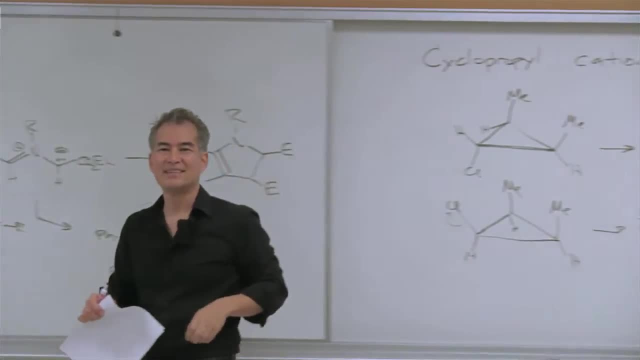 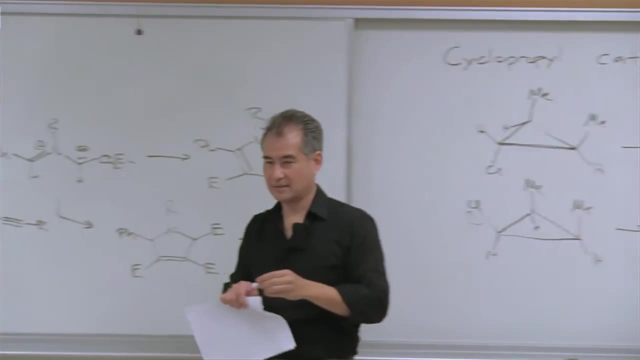 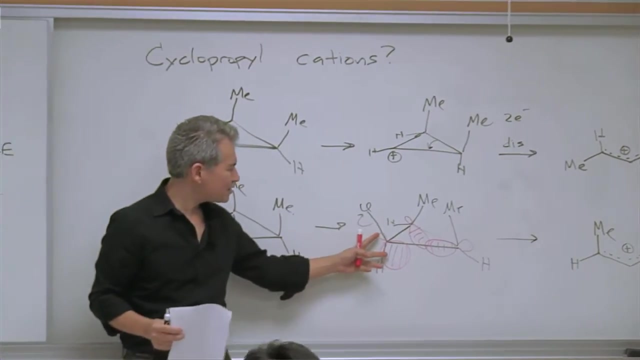 bond to overlap with the anti-bonding orbital Subtitles by the Amaraorg community. In other words, this chloride will leave faster if you're torquing these methyl groups inward, And so the point here is that you could still consider this paracyclic. This isn't a p-orbital. 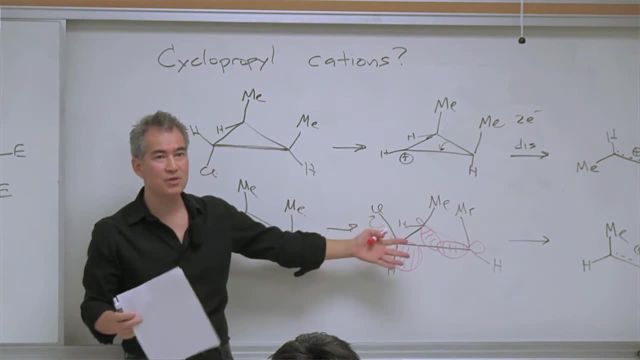 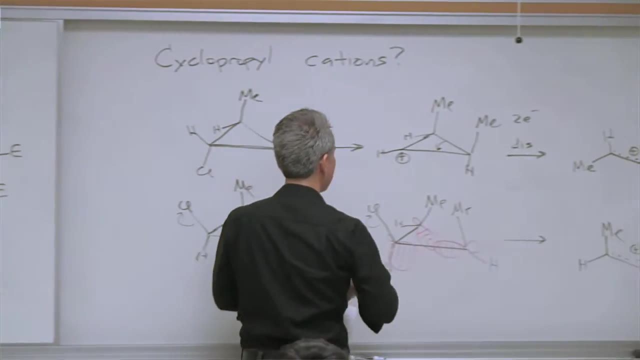 it's an anti-bonding orbital, But the anti-bonding orbital has the same symmetry- pi-like symmetry- as a carbocation p-orbital. It's got the same symmetry as this carbocation here. So if you look at this, there's orbital phasing above and below the plane. You could draw out the. 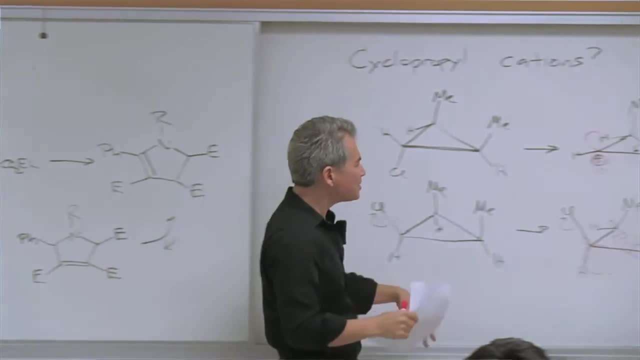 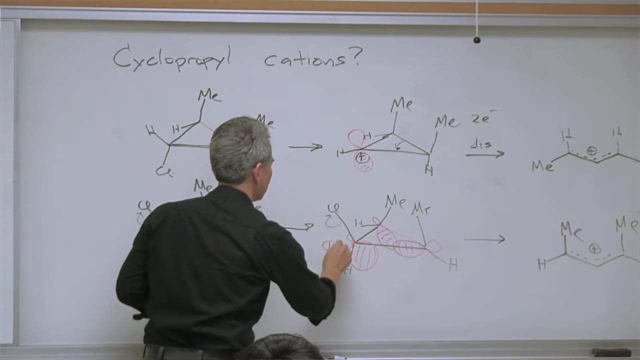 phasing there, So you can't use carbocannines to explain this result over here. You have to invoke a sigma star anti-bonding orbital instead of an MTP orbital, But you would still consider that to be a paracyclic process because it obeys these properties of orbital. 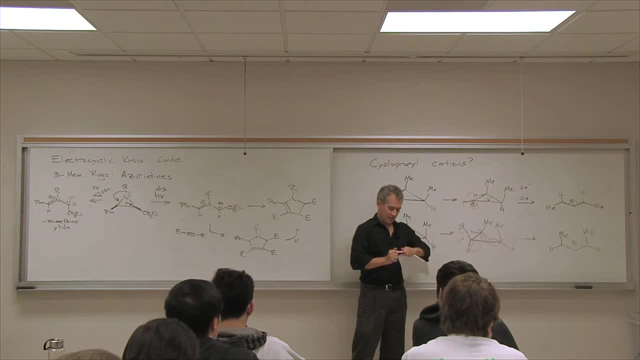 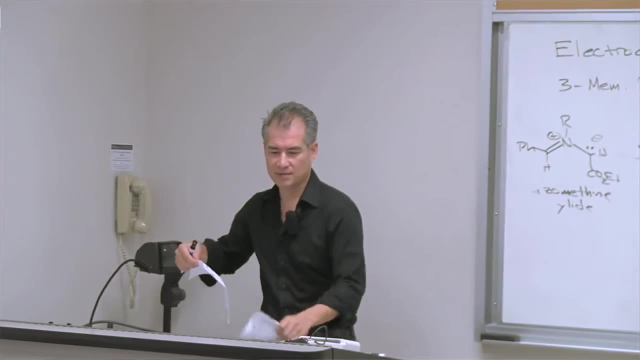 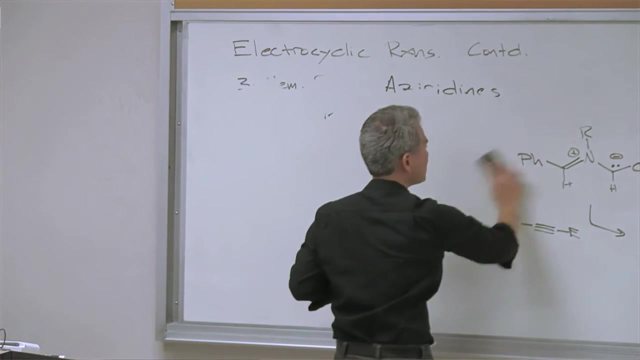 symmetry. Okay, I want to come back to one last question here, And that is what happens, something that prevents paracyclic processes from occurring. If you heat up molecules enough, they'll react in some way, And that doesn't always prove that it's a paracyclic process. 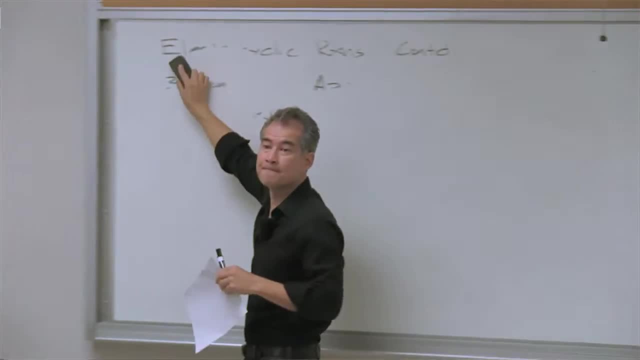 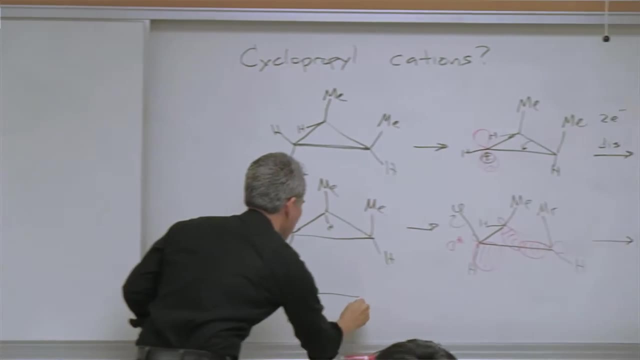 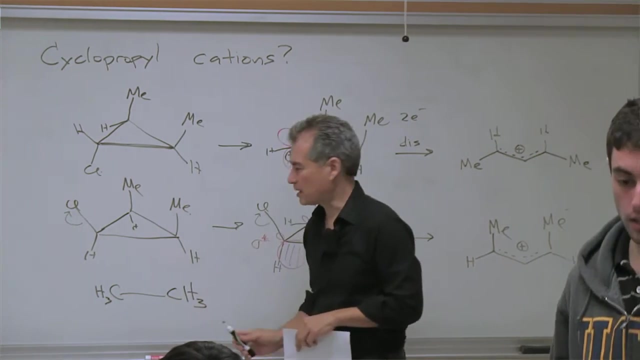 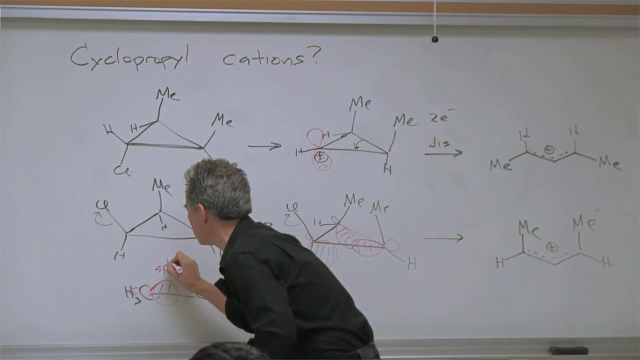 Yeah, Could you clarify what sigma orbitals are going into that sigma star scale? So if I take a carbon-carbon bond, let's make it methane here. So if I take a carbon-carbon bond, you can imagine that this carbon-carbon bond arises from the interaction of two sp3-like. 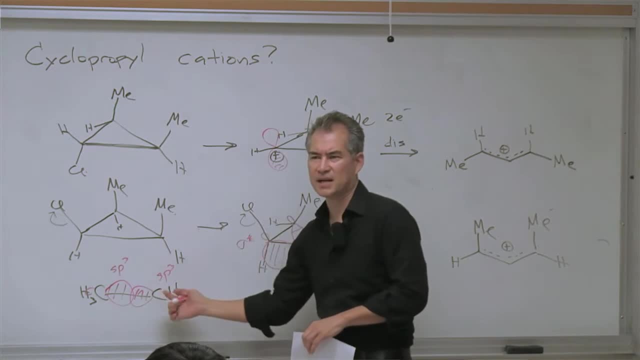 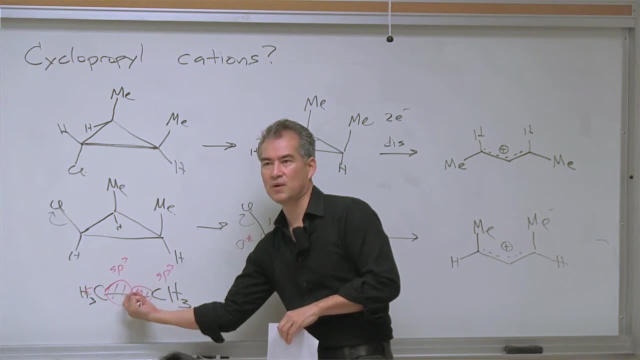 hybrid orbitals combining together. You make carbon-carbon bonds by combining two sp. If you think about orbitals as tinker toys. this bond is composed of two sp3-like orbitals that combine in a like phasing manner. And so if I distort these, if I take one of these, 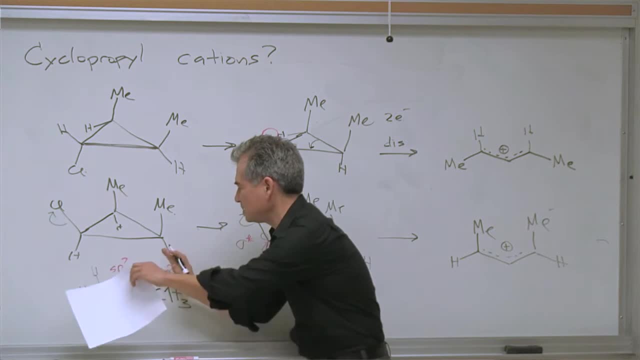 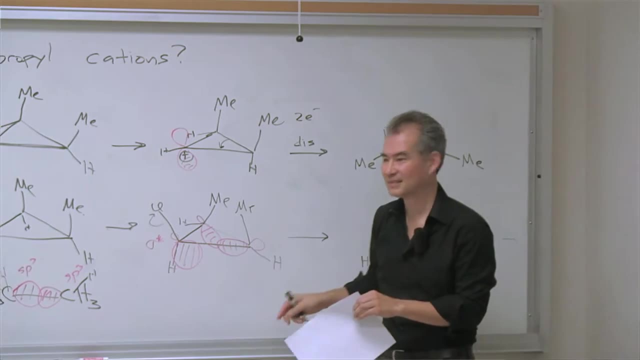 H's Or any or any substituent, and I and I torque these up. these have to bend down, And so that's why I torque this in. these have to bend downward in response to that, So it's. 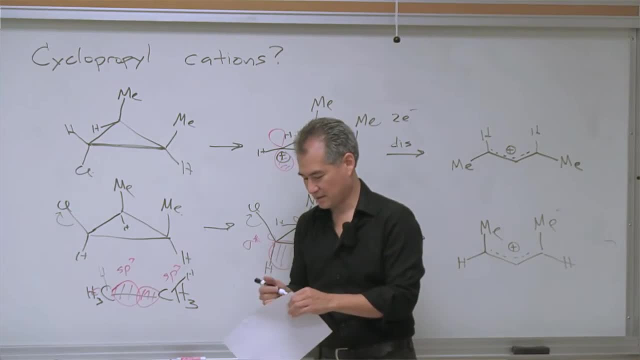 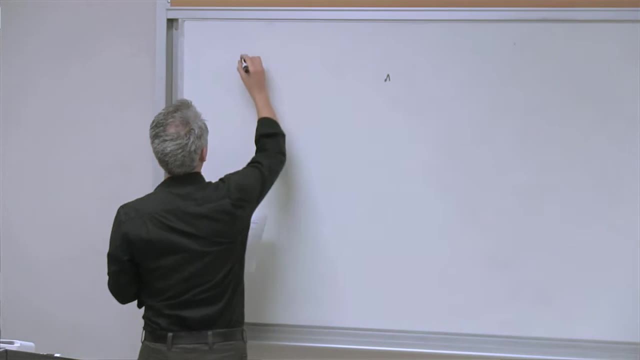 that kind of torquing here, that's, that's bending that downward. Okay so, and what I'm talking about here is general, It's not just electrocyclic reactions, And what I'm talking about here is general, It's not just electro-cyclic reactions. 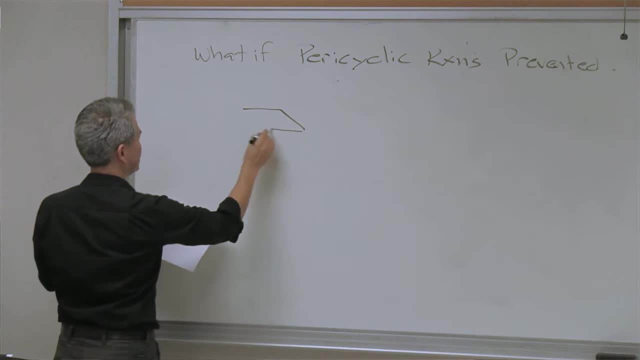 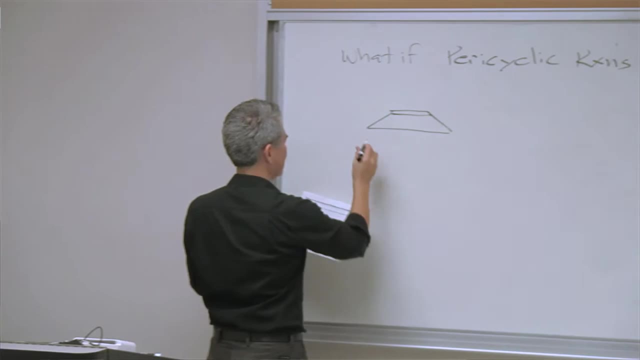 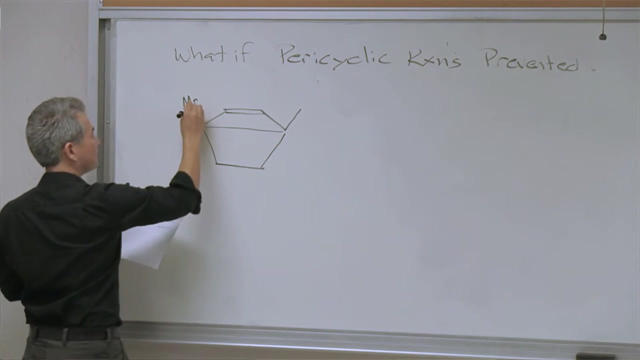 I'm going to try to draw this molecule here called dewar benzene, And I'm going to start by drawing a cyclobutene ring kind of edge on, because I want to try to imagine these two substituents here. They can be methyl groups. 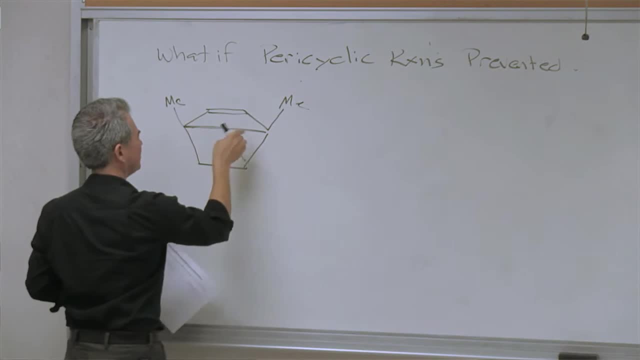 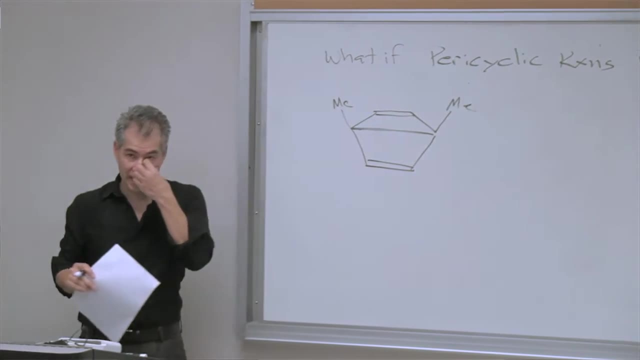 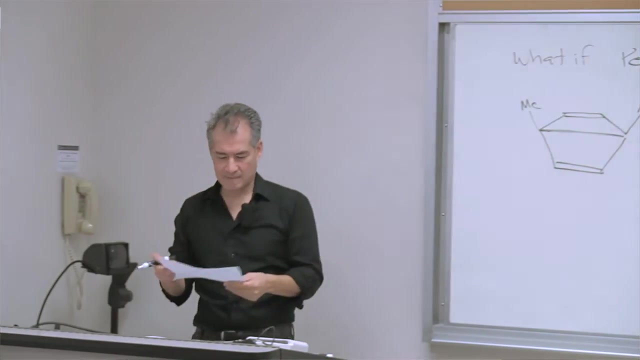 It doesn't matter, Above the plane of the ring And I'll draw the rest of this other ethylene bridge, ethene bridge, below the plane of the ring. So it's kind of like a benzene ring if you kind of just look at the six atoms in the middle. 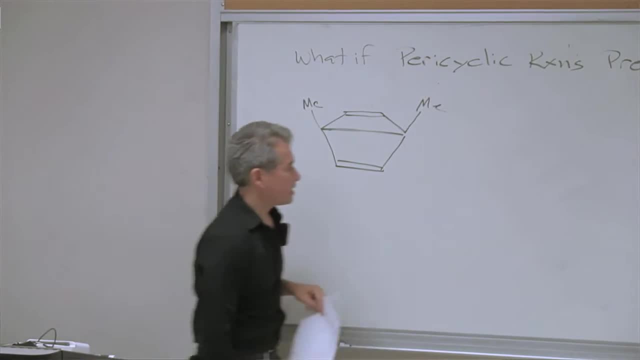 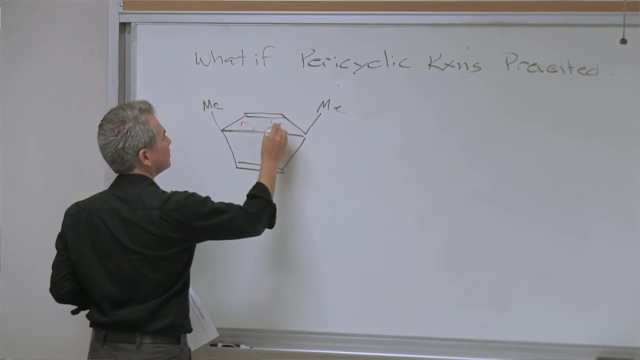 And in theory, all you have to do if I get my red pen out, OK. OK, So the solution out here is doing electro-cyclic ring opening And then you can make benzene. So you can imagine there is a huge driving force. 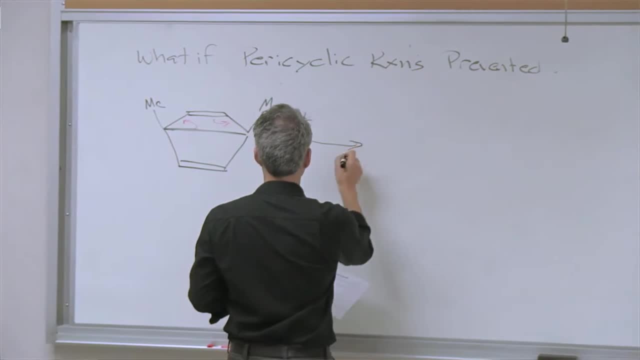 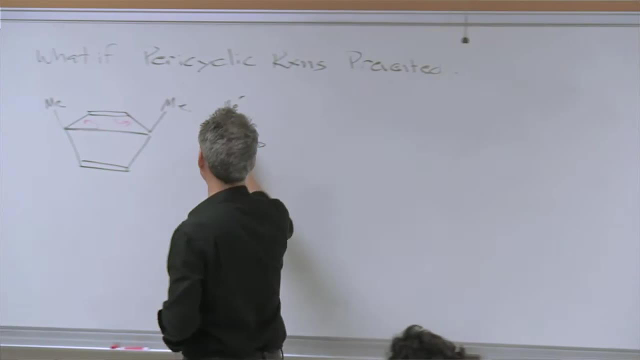 aromaticity for ring opening to form benzene. The problem is, this is a four-electron process, And if it's a four-electron process it has to be conrotatory, And conrotatory means, if I spin this group out- 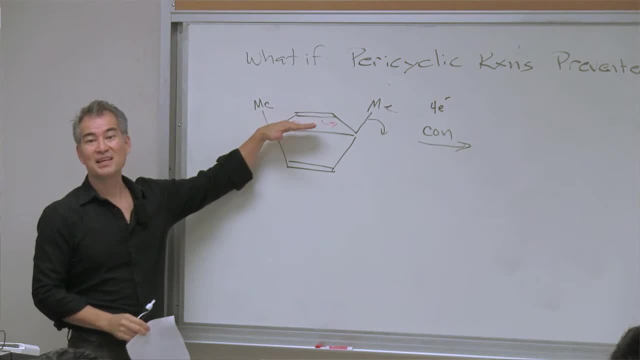 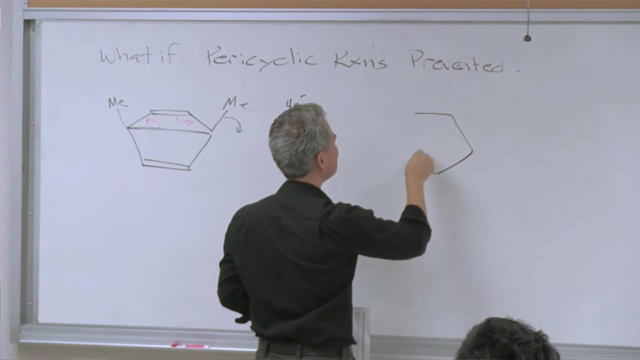 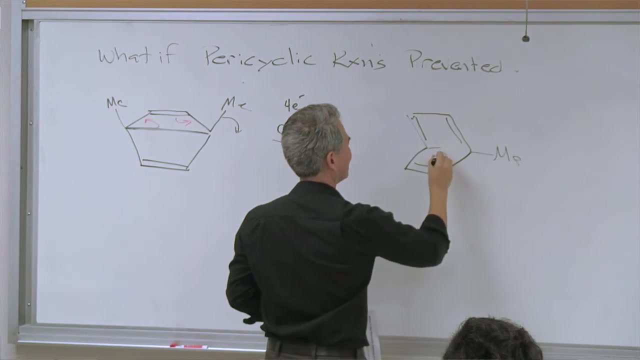 of the benzene ring. this other group, other group also has to spin inward. There's no escaping that. And I promise you you're not going to generate a benzene ring where one of the substituents is pointed inside the ring. I don't even know how to draw this. It's killing me here, So I'll just put that. 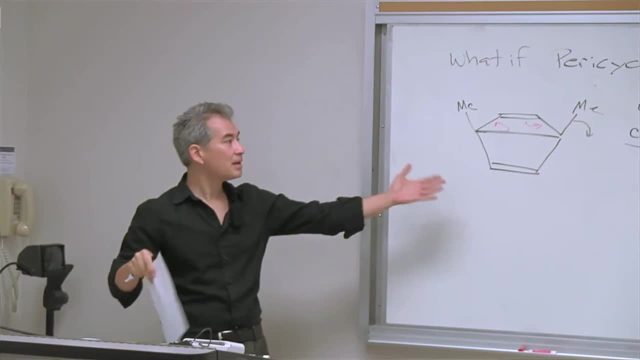 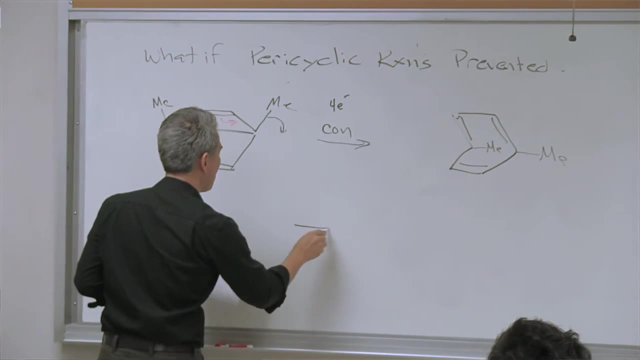 methyl group somehow inside there, Right, there's no way you can do this. But that's not to say that this can't ring open. In fact it doesn't take a lot, but it's very easy to open Dewar benzenes If you take Dewar benzene and you simply heat it briefly at. 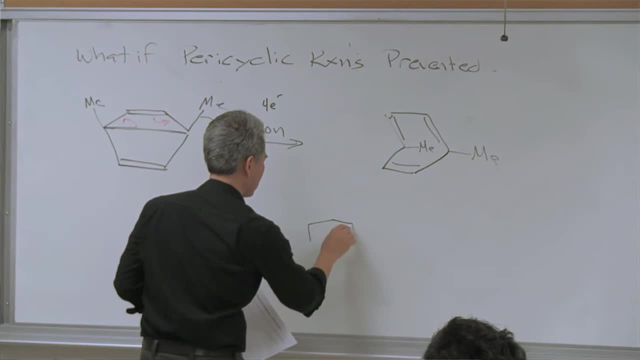 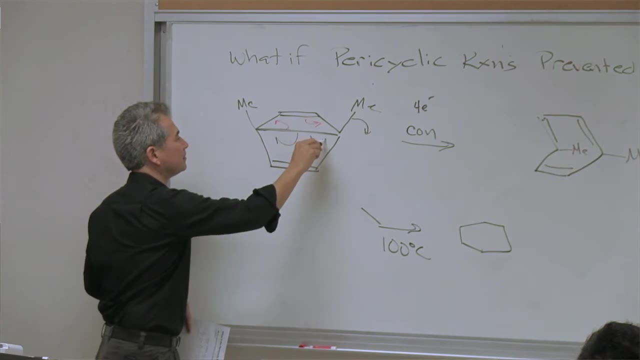 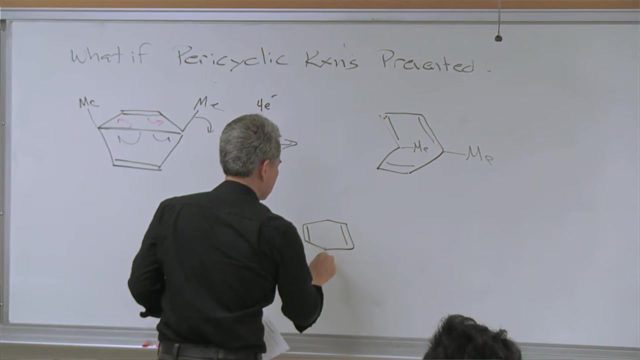 100 degrees it will form benzene or an airing ring, but it does it through radical reactions. So what's happening here is it's popping open to give two radicals, And so this is a general feature of reactions. If you somehow prevent the orbital symmetry allowed, process you. 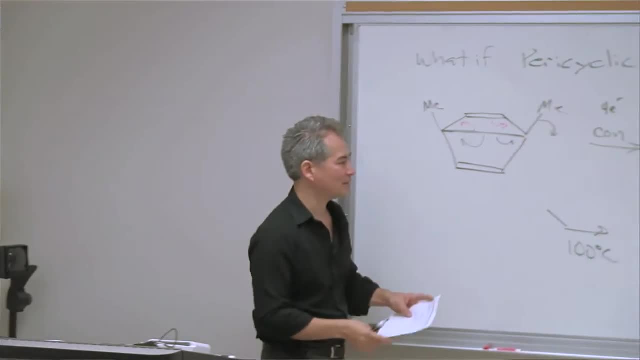 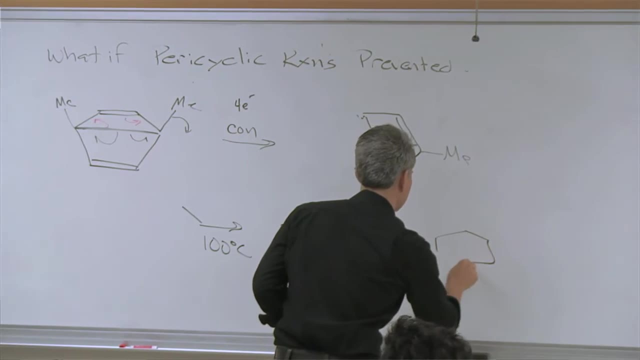 can still generate a benzene ring, You can still generate products, but it's usually through some sort of a diradical. And so now- and there's initially a spin- I'm not going to, we're not going to talk about spin unless we can get to photochemistry in this class. But eventually this can reform. 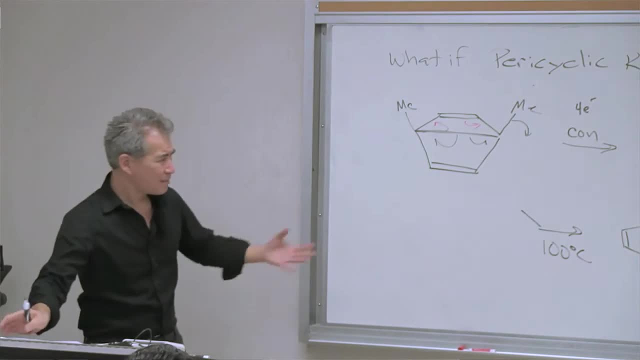 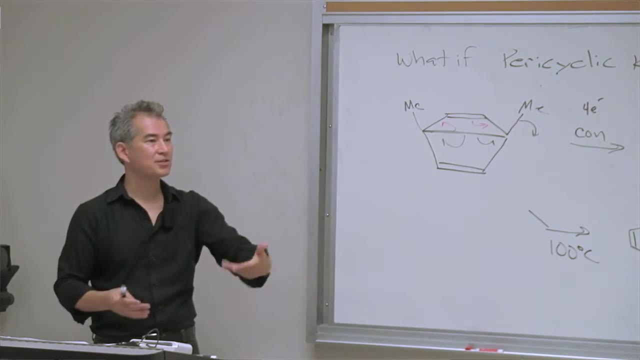 a benzene ring. Okay. so if there's some orbital symmetry problem that prevents pericyclic reactions, Diels-Alder reactions, sigmatropic reactions, ene-like reactions, oftentimes you'll have radical diradical reactions. 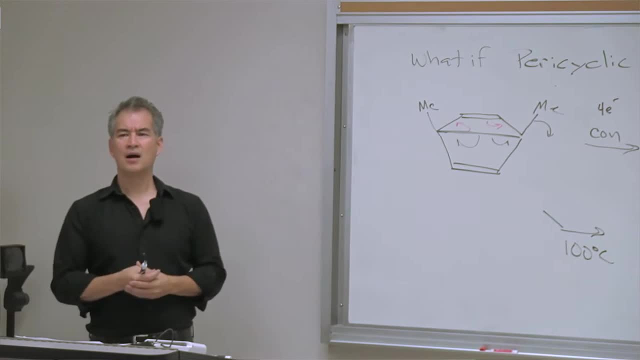 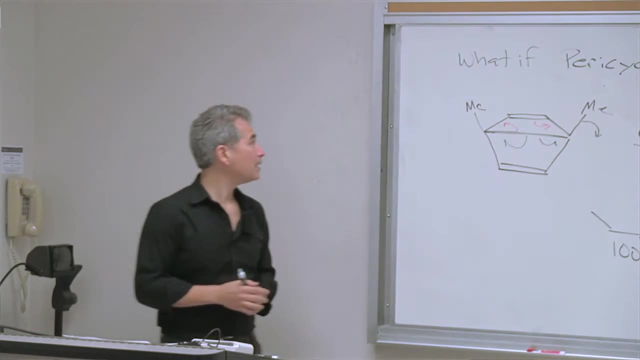 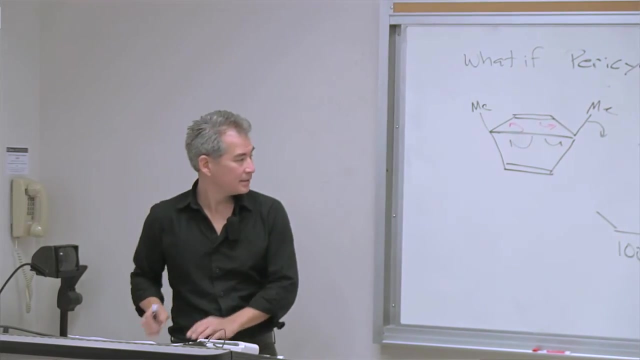 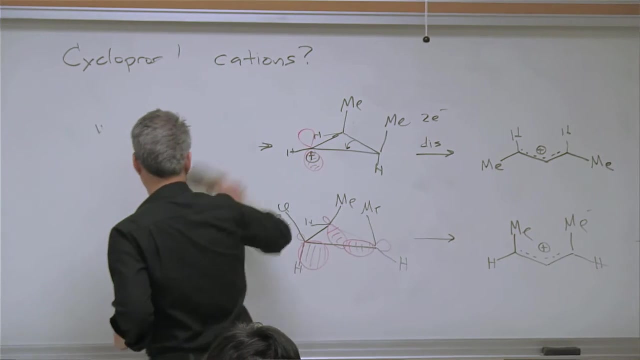 Or if you've got the right substituents that stabilize ions: ionic reactions, carbocations and carbanions. Okay. so that's it for electrocyclic reactions. So let's totally switch gears now and let's talk about sigmatropic reactions. 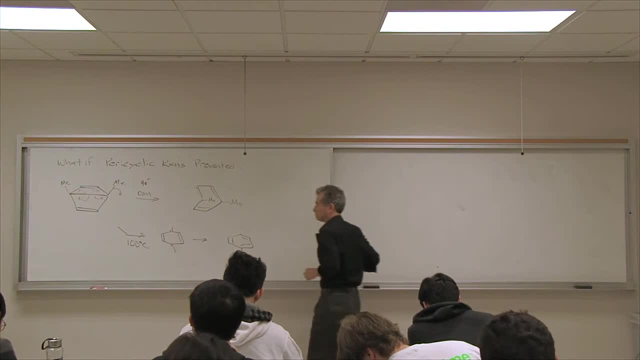 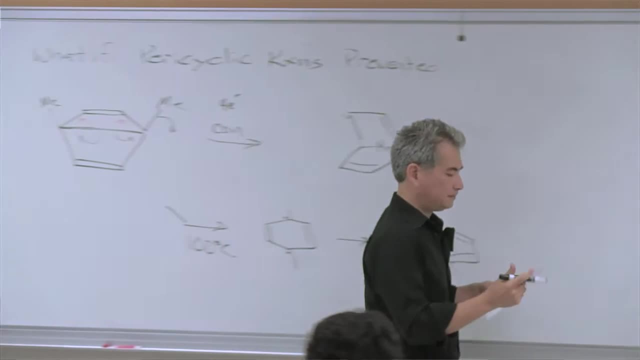 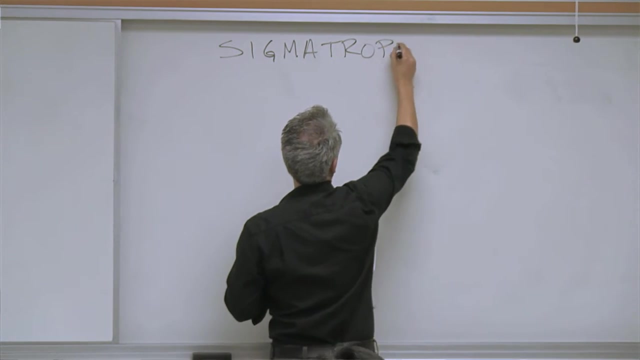 Patients are generically dropped for radiation when they suffer through oral ninety- güç applications, that which can cause complications such as personality, hemoglobin, osteoocene, pta, così as bandeja viso, Penicillin, and pharyngeal tightness of the gums. 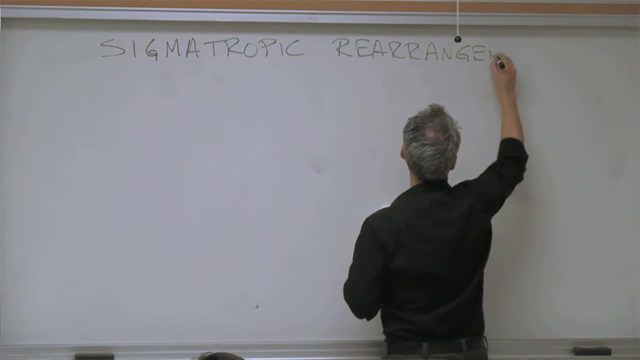 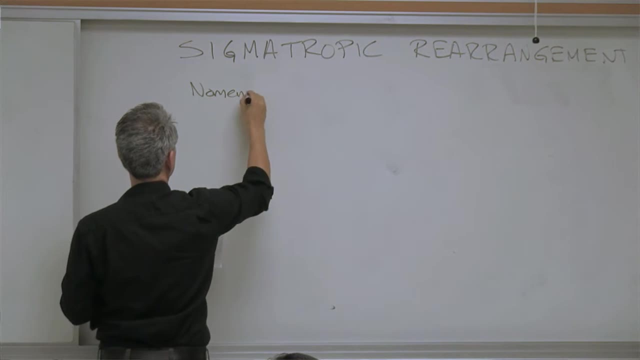 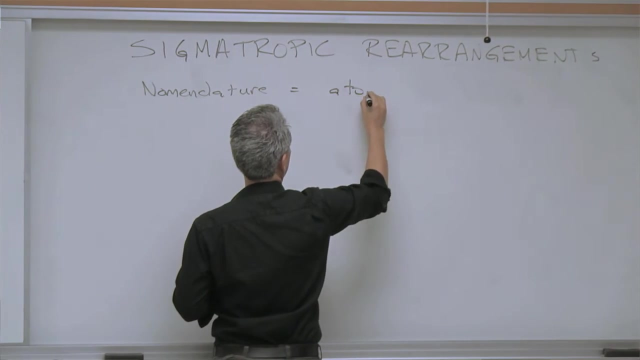 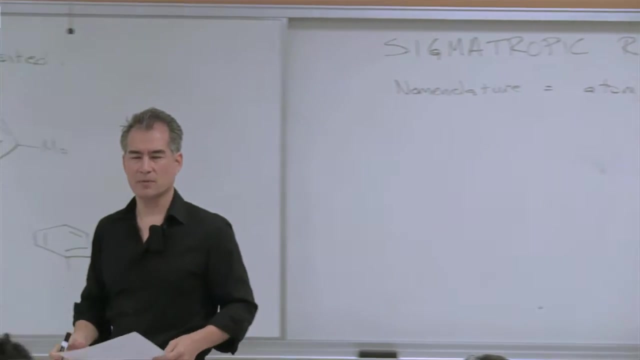 Organic reactions. Reaction قال: angiavors нять. parasympathetic reactions, virulent vasculature. Okay, the nomenclature that we're going to use, and that is commonly used for sigmatropic reactions, is based on atom fragments. 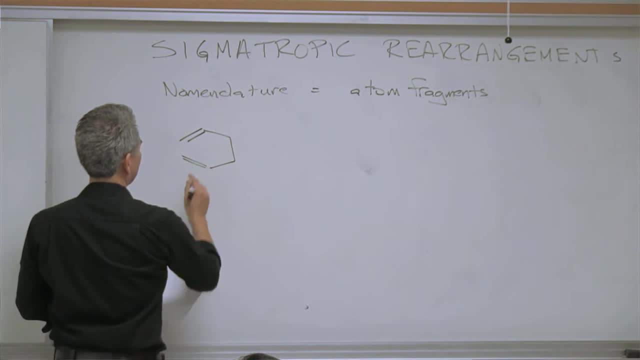 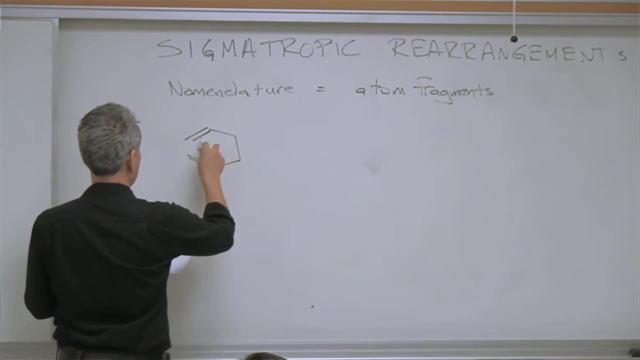 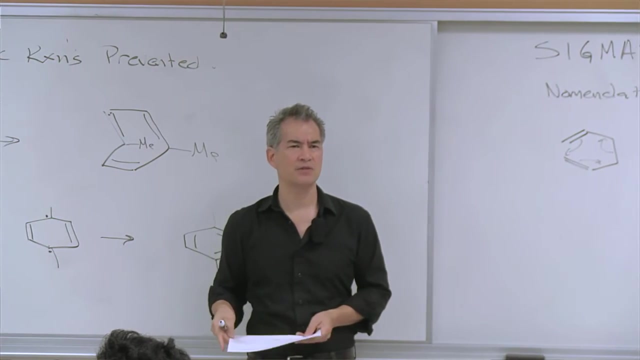 So I'm going to start off with this canonical sigmatropic rearrangement that involves a six-membered ring. It's called a Cope rearrangement And one way to think about this that will help you analyze anterofacial versus superfacial. 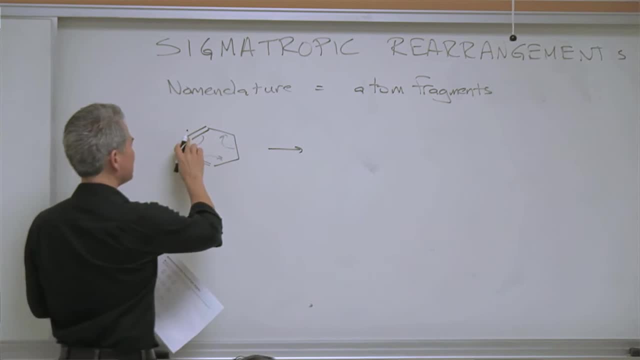 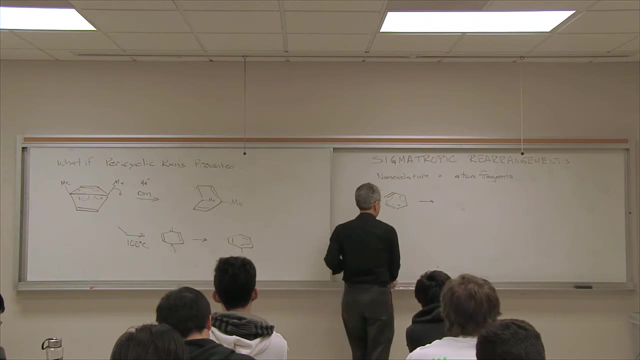 stereochemical issues is to think about this as involving two three-atom fragments, And let me add some numbering here so we can see what those two three-atom fragments are going to be. So when I draw the product of this and you can do the arrow pushing in the reverse, 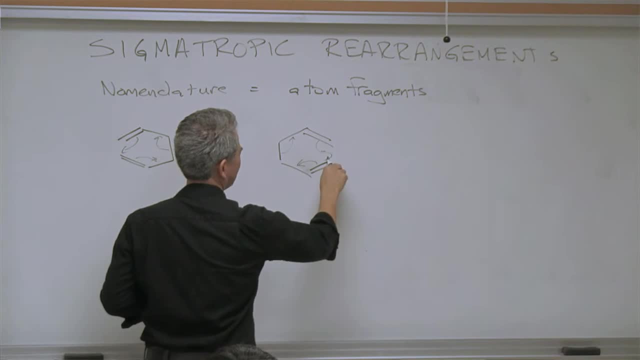 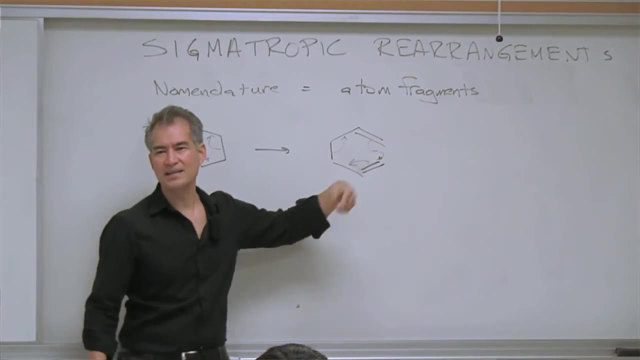 Direction. I want to make sure this arrow ends on that carbon. I want to be really picky about that. I don't want you guys to make the arrows just end in open space, because that doesn't represent some sort of an anti-bonding orbital. 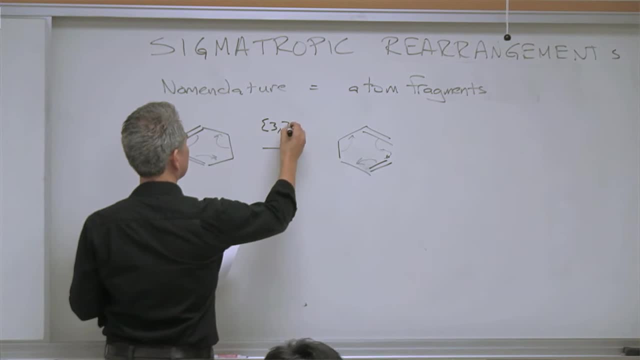 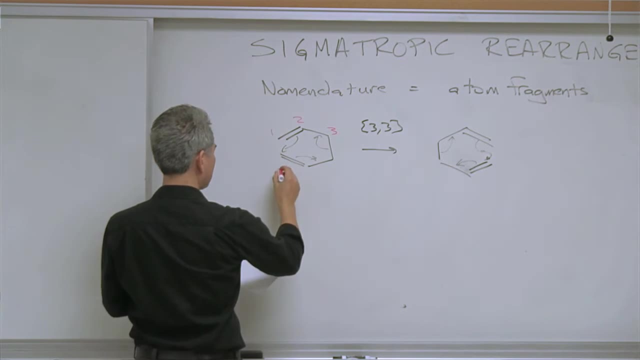 Okay, so this would be called a 3-3 sigmatropic rearrangement, And the way to think about this is that this is composed of two three-atom fragments. The numbering here- you know what's one, two and three- is arbitrary. 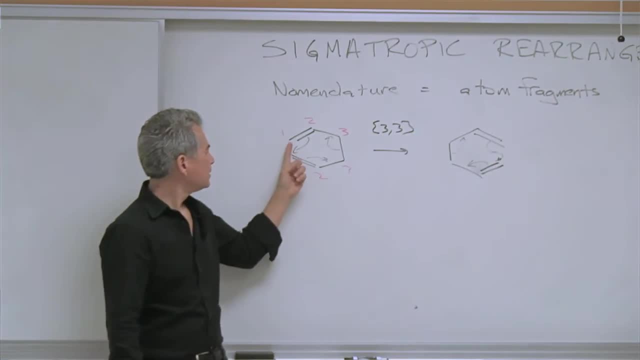 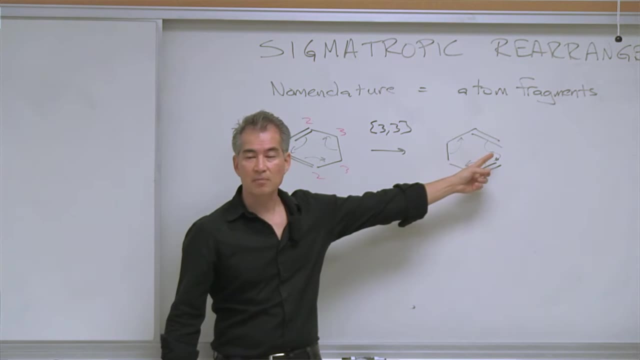 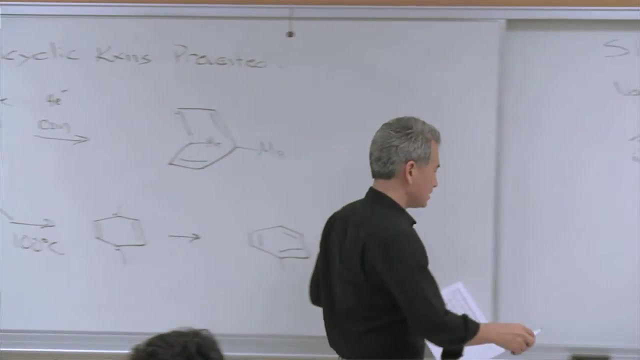 The point is I've got two fragments, each composed of three atoms. In the beginning there's no bond here. In the beginning there's a bond there, And then that's reversed in the product And the point is that in the transition state you have partial bonds between those two fragments. 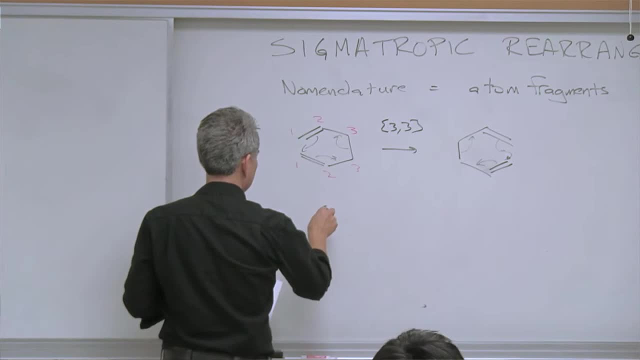 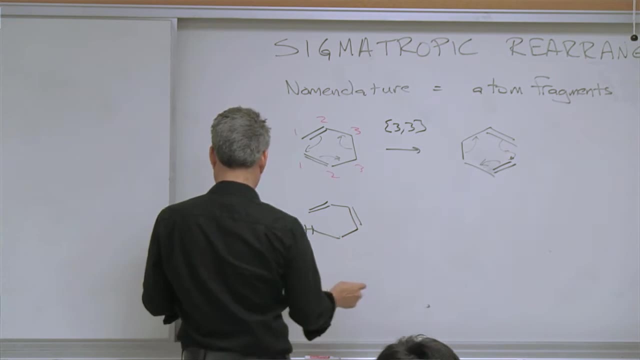 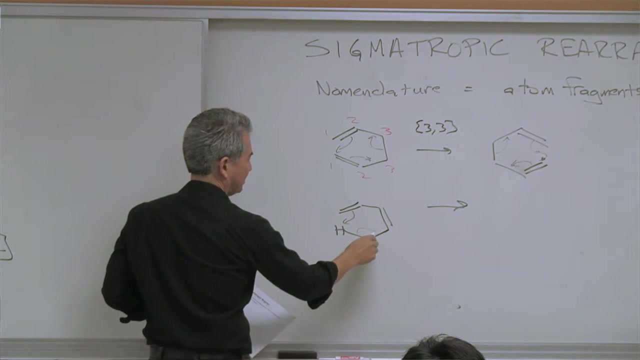 Let's take a look at a slightly different version of a sigmatropic rearrangement. that involves also a six-membered ring, And what I need to imagine is I'm plucking off this proton and then giving those electrons back to this carbon system here. 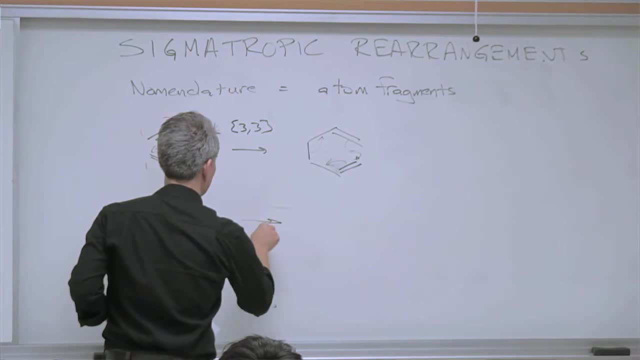 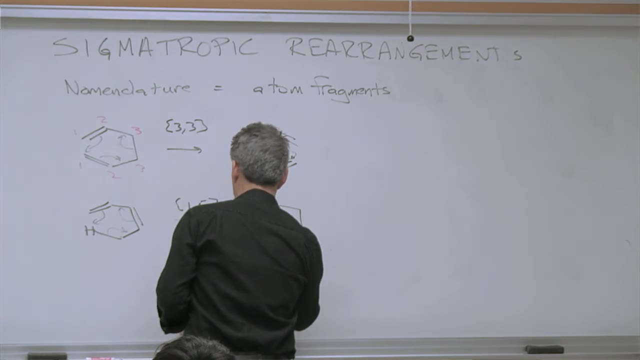 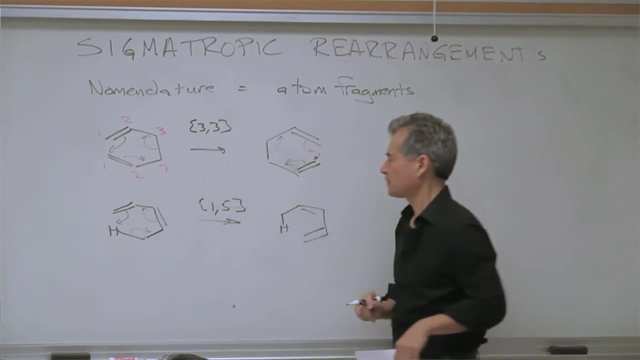 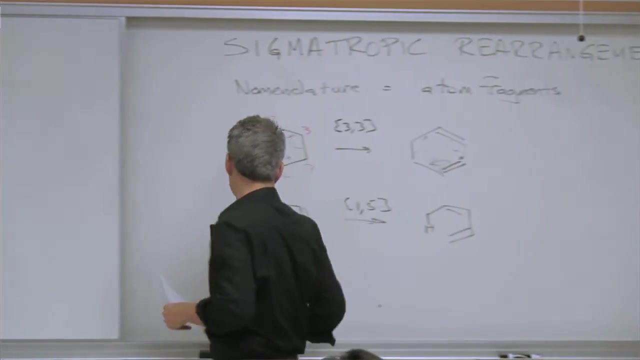 And we would call this a 1-5 sigmatropic rearrangement. And if I follow my arrow pushing, it should look like that: Now the H is attached to that upper carbon instead of the lower carbon, And let's count the atom fragments. 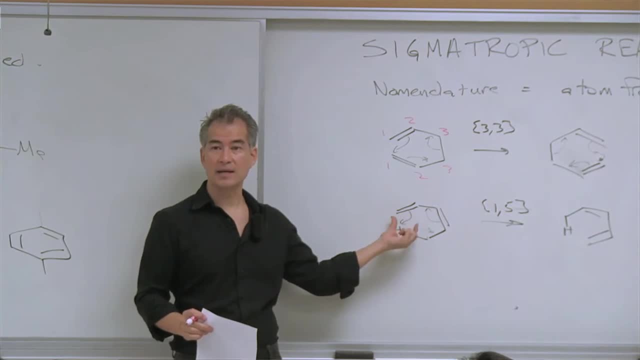 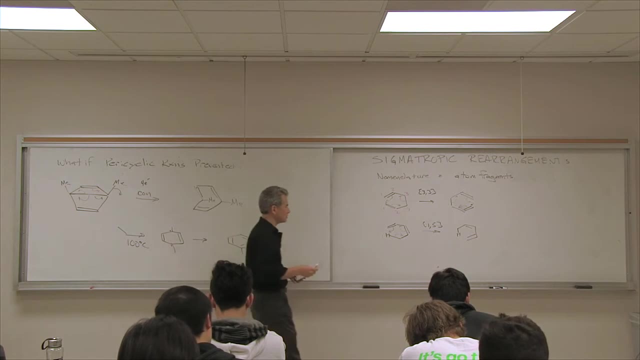 So there's a proton. In the transition state there's partial bonding to the proton, So this proton is really just a one-atom fragment. In the transition state there's partial bonds to the proton. The other fragment is composed of five carbons that stay bonded throughout the entire course. 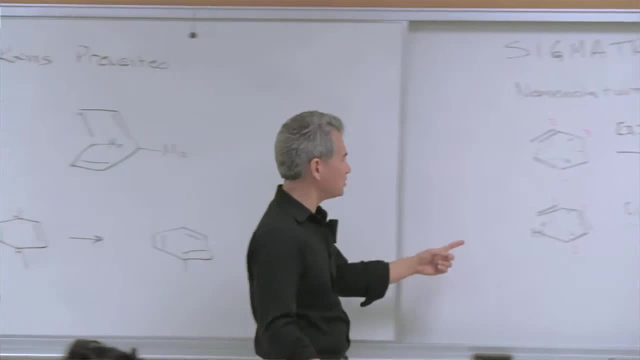 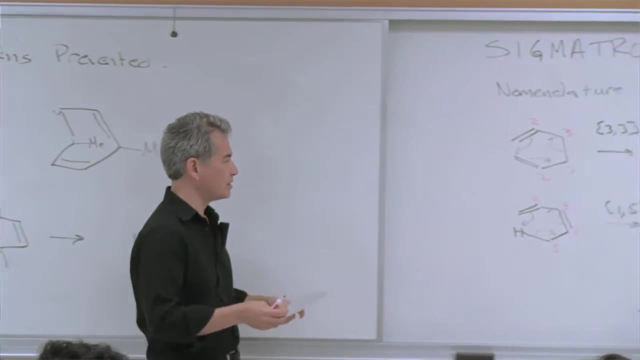 of this rearrangement? At no point, do you. There's at least some kind of bond between all five, All five of these carbon atoms. So this is a 1-5 sigmatropic rearrangement, And I could draw the reverse arrows. 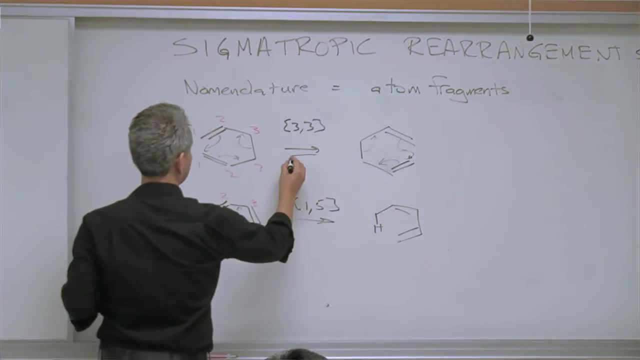 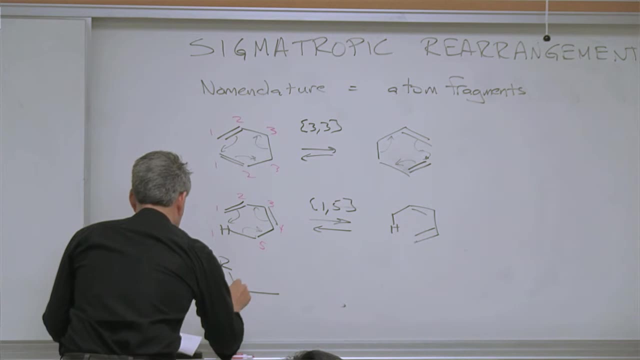 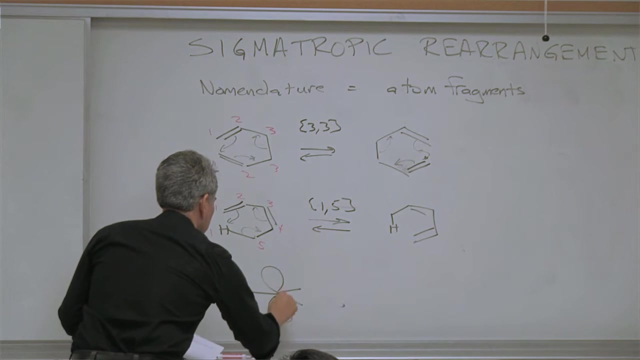 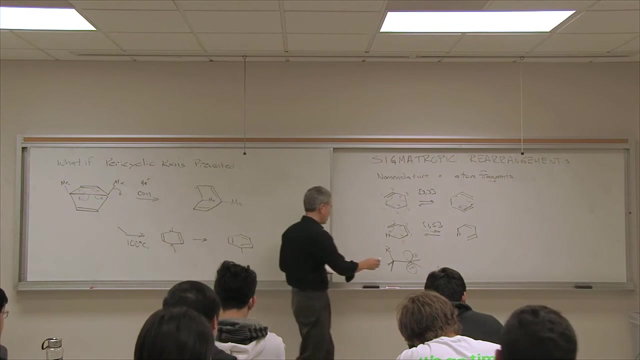 I'm not going to for the backward reaction. I'm not going to do that. I'll just indicate that these are all reversible. Here's a very common rearrangement that I think you saw a lot of last quarter, And that's carbocation shifts or hydride shifts. 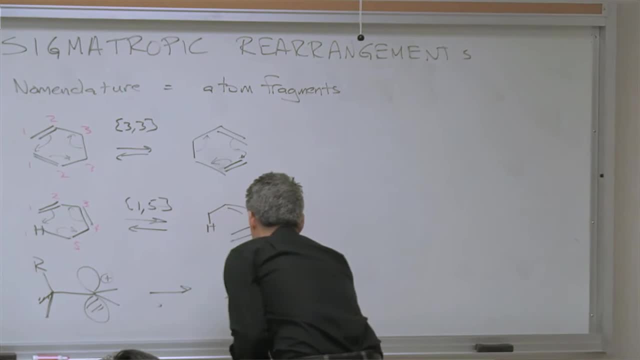 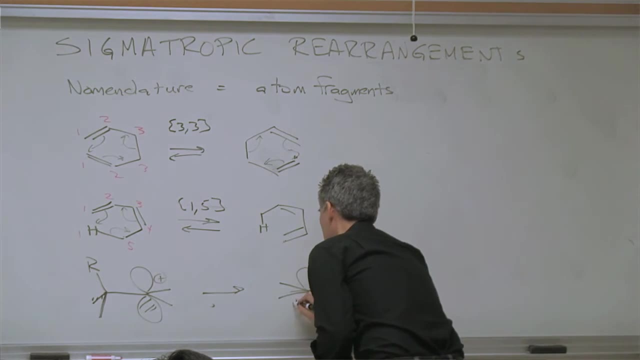 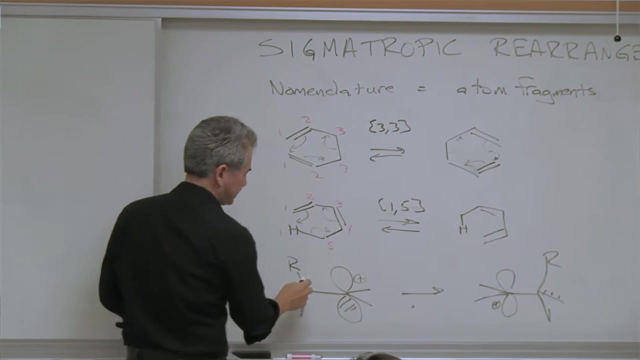 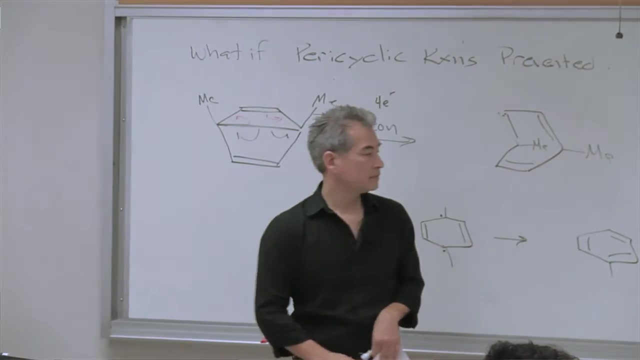 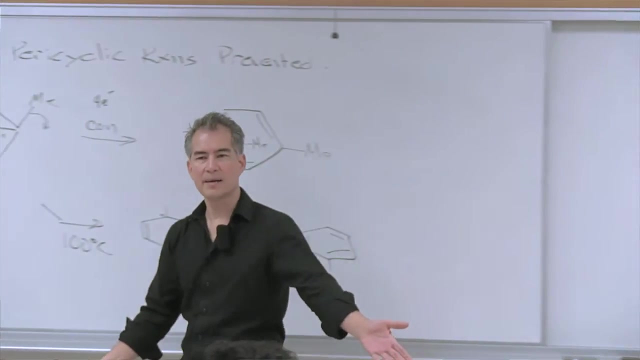 And so if I draw the arrow pushing here, I simply take the electrons- There's two electrons in this carbon-carbon bond- And I donate those in the empty orbital. And if I number my fragments here, This two-atom fragment on the bottom stays bonded the whole time. 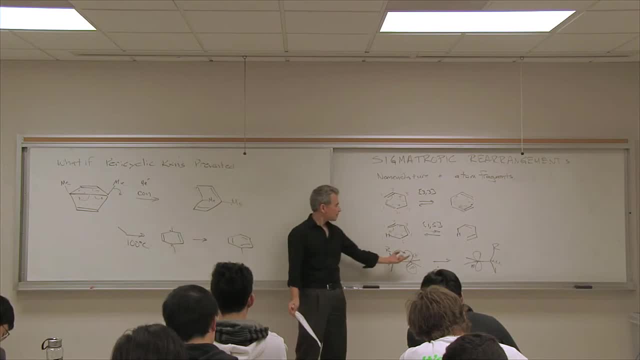 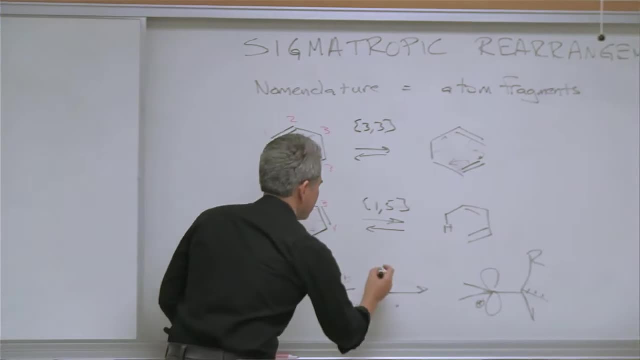 There's always a bond between one and two, going from starting material to product, Whereas this R group is my other one-atom fragment. So this is a 1-2 sigmatrope, This is a 1-2 sigmatropic rearrangement. 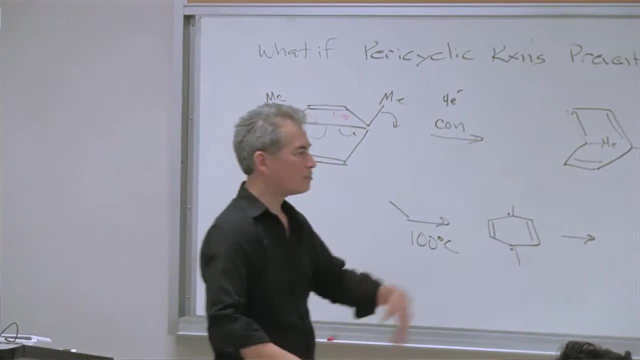 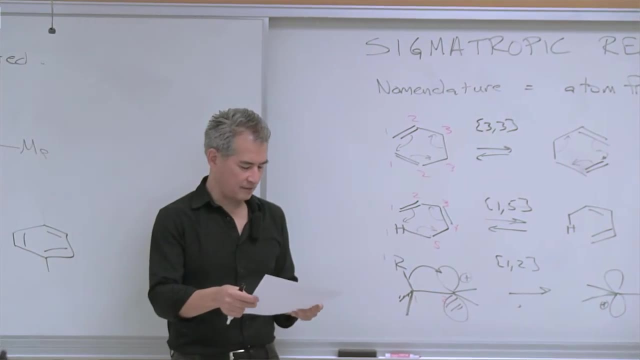 You probably call it a 1-2 shift, but that's a sigmatropic reaction. It obeys all of the paracyclic selection rules based on orbital symmetry that all of these other sigmatropic reactions have to follow. Okay, there's another. 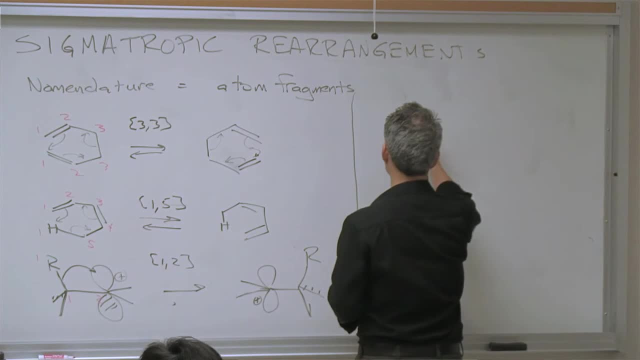 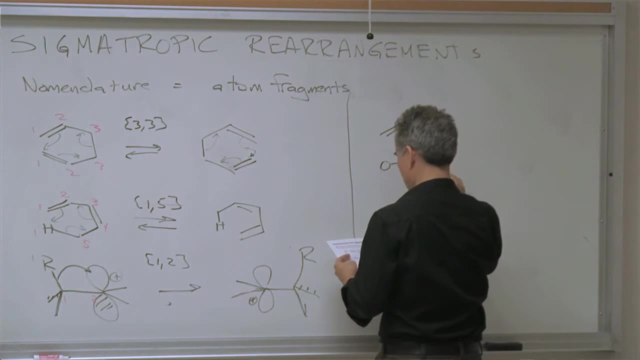 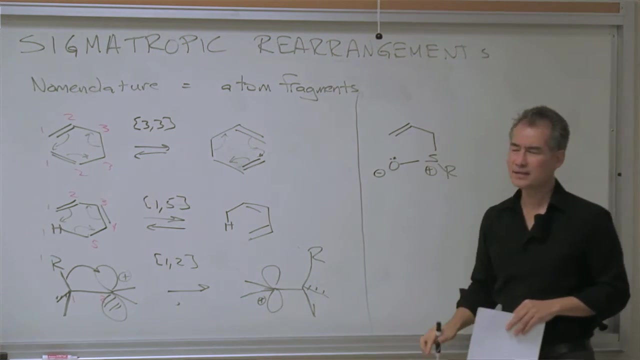 There's one more class of rearrangement reactions And there's still. It's not always clear what's going on in these reactions. I'll show you one of the most common examples of this. This is a sulfoxide. So we've talked a lot about sulfoxides or sulfur chemistry. 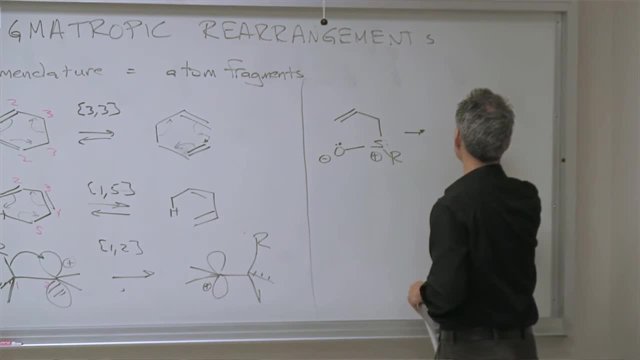 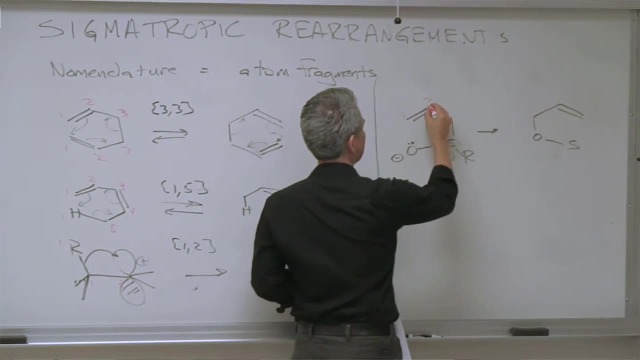 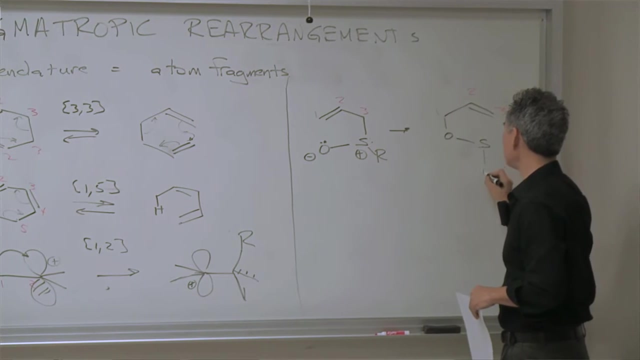 And this can undergo rearrangements quite fast. Okay, There's also some more classile rearrangements in which these atom fragments look like this: So there's an allylic fragment, And then there's this sulfoxide, sulfenate, sulfenic ester fragment here. 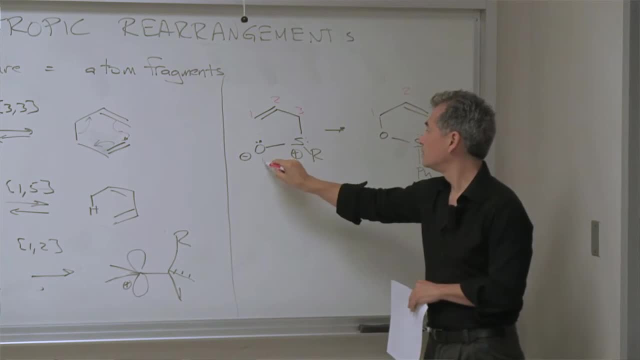 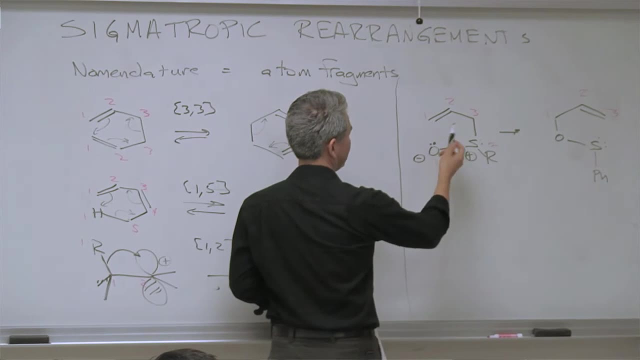 So there's always a sulfur-oxygen bond from beginning to end And there's always all the carbon. All the carbons in the allofragment remain bonded, Remain bonded from beginning to end, So you can draw an arrow-pushing reaction that looks like this: 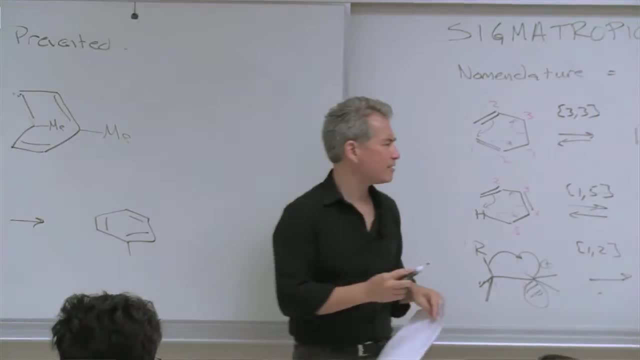 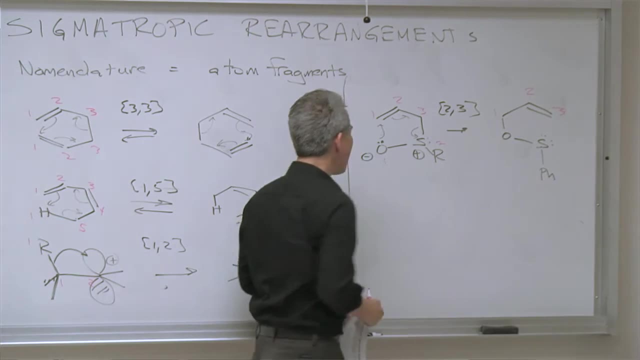 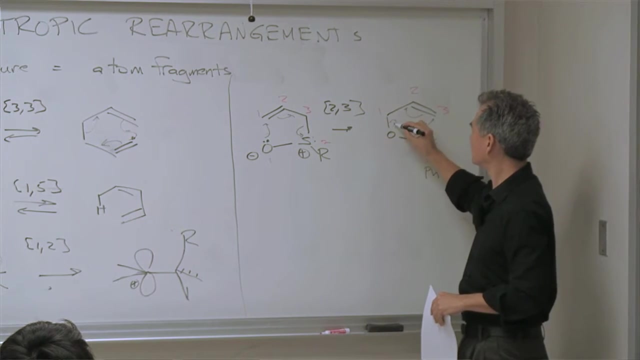 The problem with this? This is called a 2-3 rearrangement. The problem with this is nowhere in my mechanism. regardless of whether I push forward or backwards with my arrows, nowhere in my mechanism am I affecting the bonding between the oxygen and the sulfur. 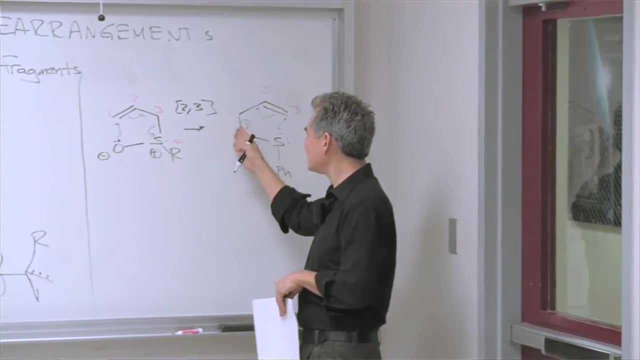 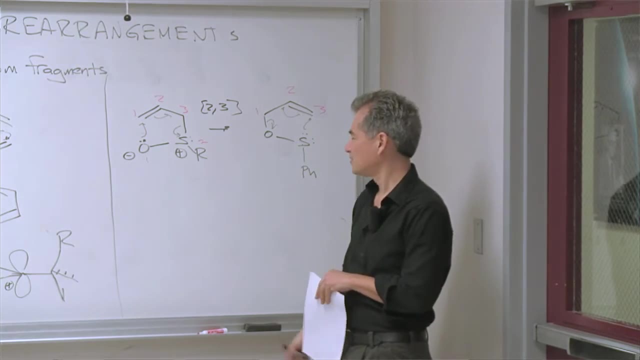 And if there's no interaction between the electrons on the oxygen and the electrons in the sulfur, then how can this be paracyclic? How can it involve a cyclic array of electrons? So there's some debate as to whether these are paracyclic. 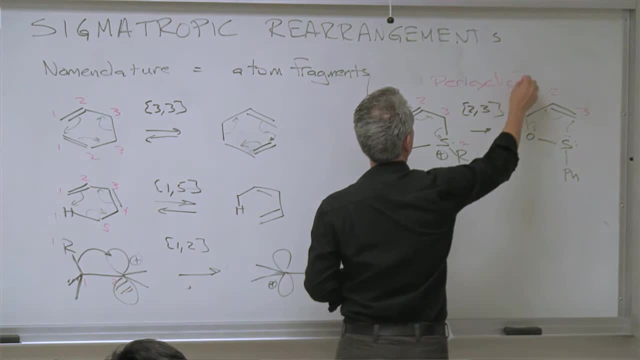 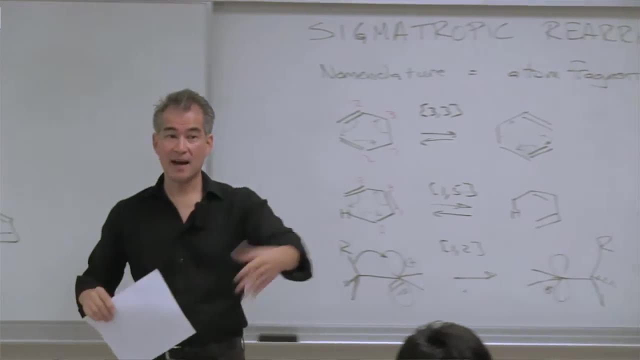 So I'll just write paracyclic, And in fact if you do the carbanion version of these, you can't find a paracyclic transition state unless you include a sixth atom somewhere. So I'll just leave this as a question. 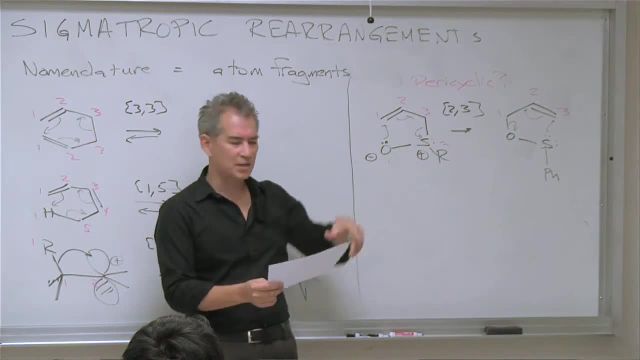 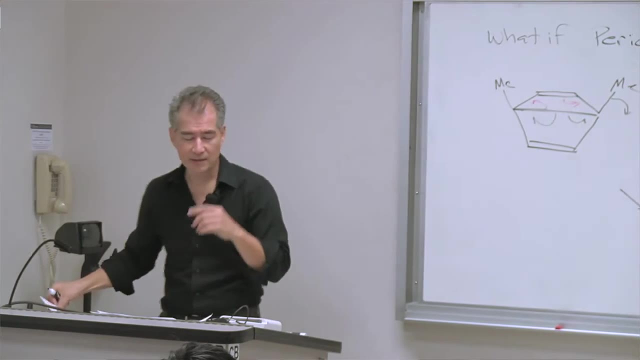 Mark as to whether this, Even though we will call it a 2-3 rearrangement, it's ambiguous as to whether that's a paracyclic process. OK, So let's take a look at the simplest and most common version of a sigmatropic rearrangement. 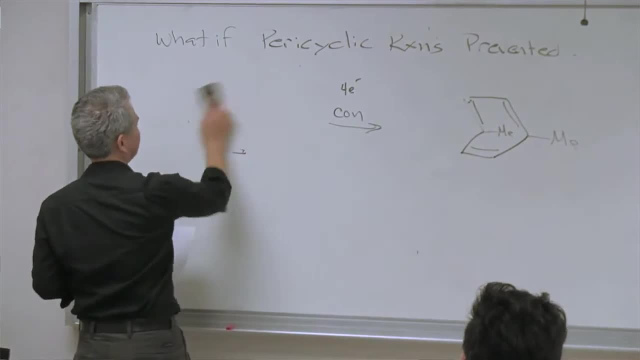 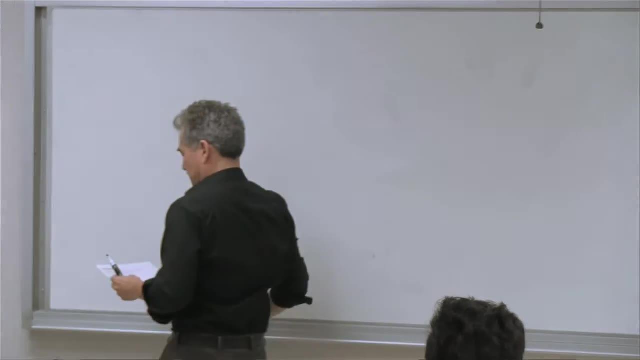 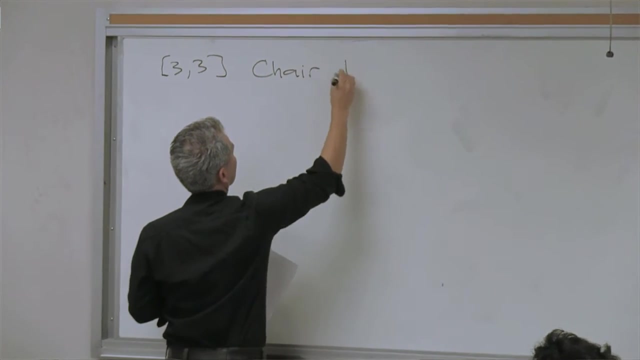 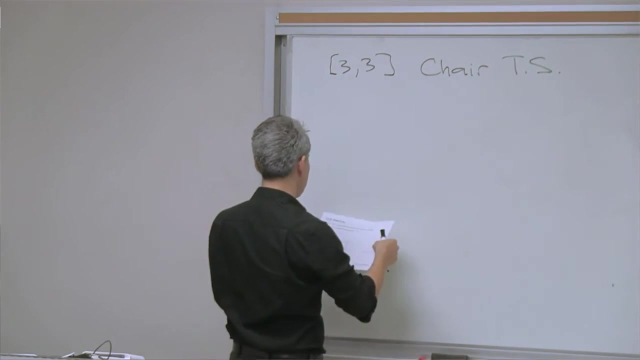 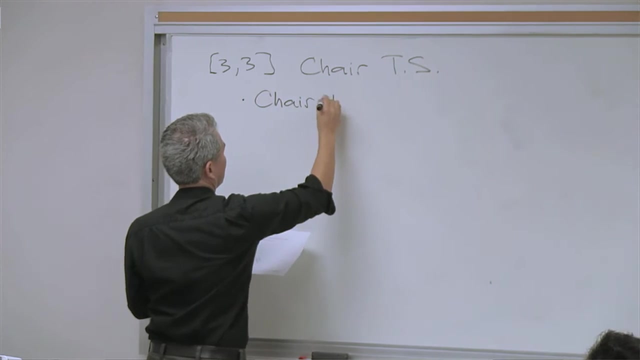 And that's the all-carbon system with a six-membered transition state, And this will give us a chance to talk about stereochemistry. So 3-3 rearrangements, 3-3 sigmatropic rearrangements, prefer chair transition states. 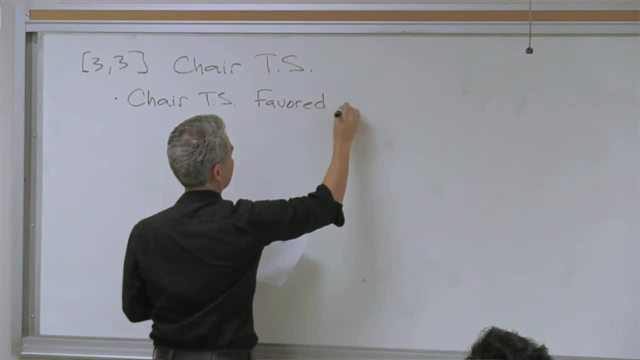 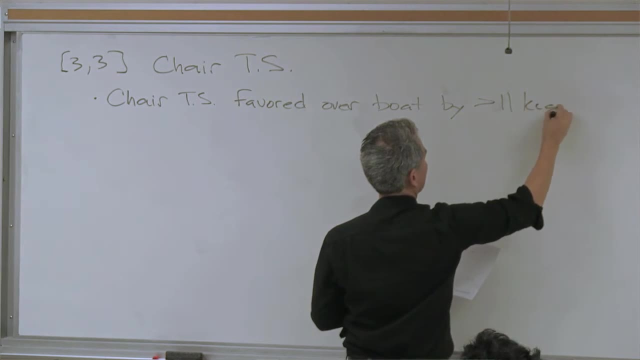 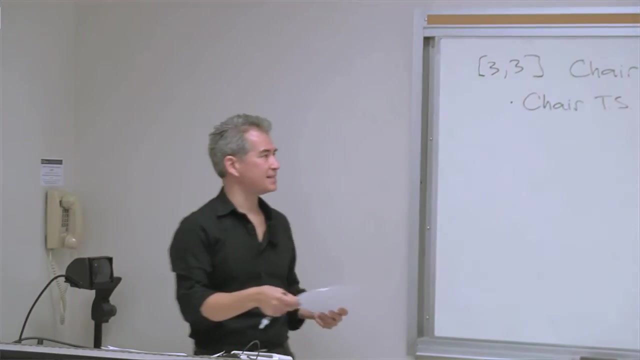 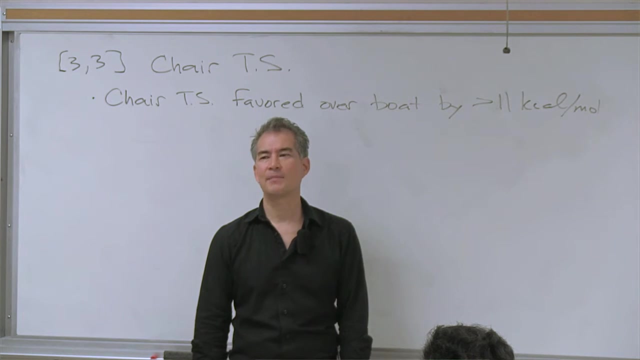 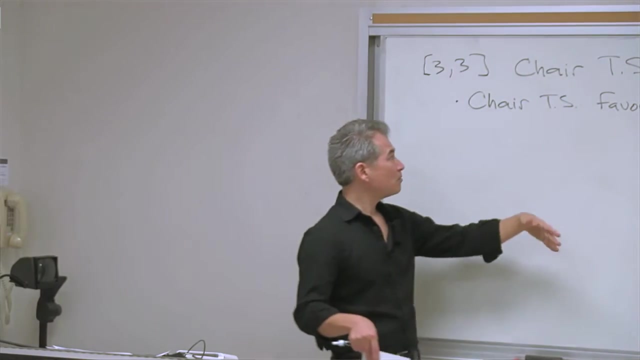 OK, Cool, Thanks. over 11 kcals per mole. How many factors of 10? is that? 1.4 kcals per mole is a factor of 10.. I'm not that good at math, but you guys are good at that. 7. 10 to the 7th, So chair. 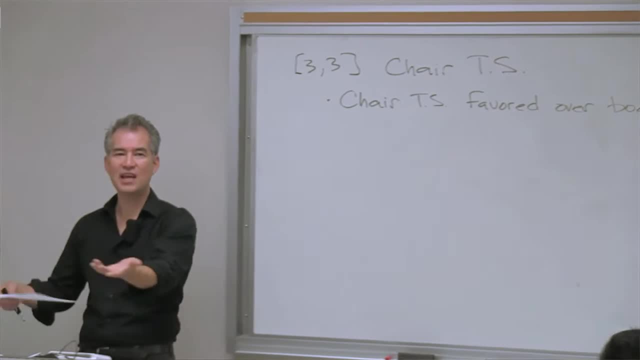 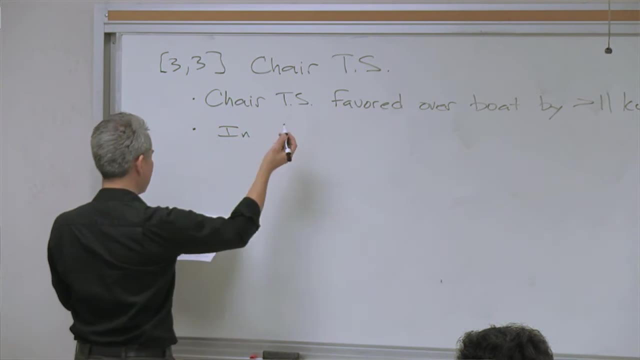 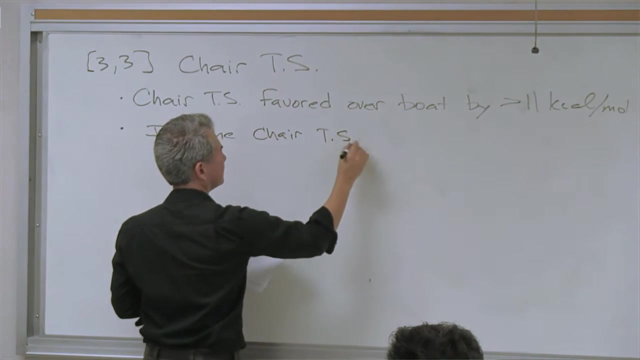 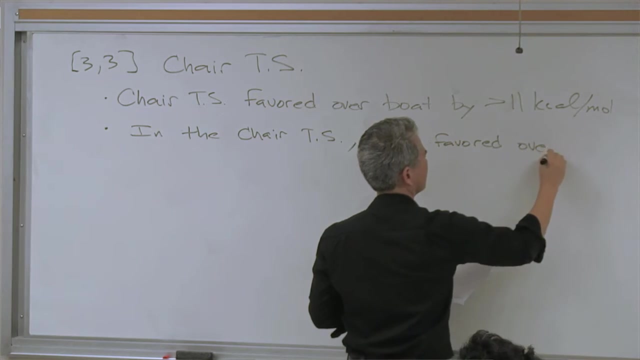 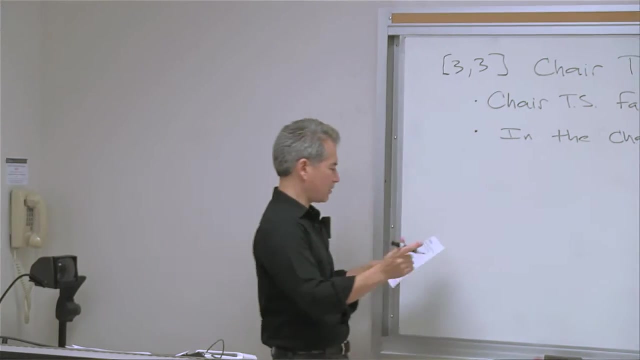 transition states ought to be faster than boat transition states by 7 orders of magnitude. So you should expect huge selectivity for chair, like transition states. And then the next thing is kind of obvious: You want your substituents to be in equatorial over axial. 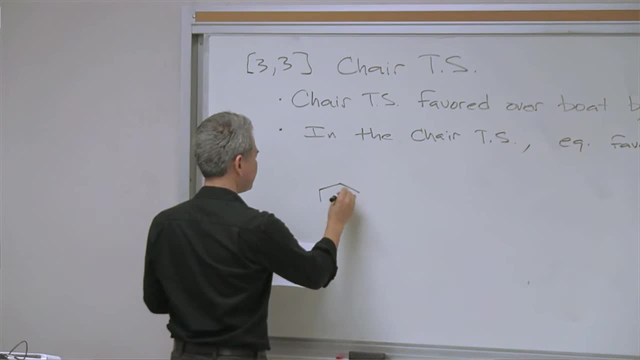 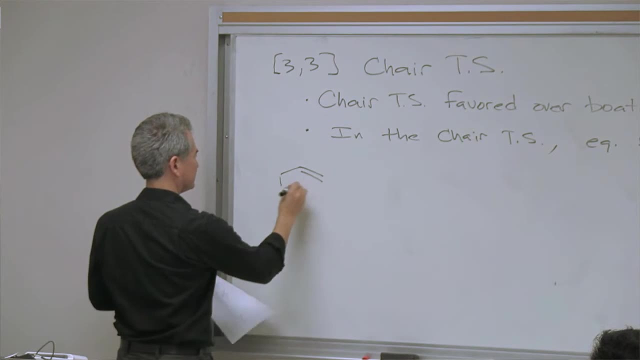 like orientations, So let's start off by: I hope I'm going to have room here, so let me make sure I leave some room. I'm going to draw three structures over here for products on the board, So this would be an example. 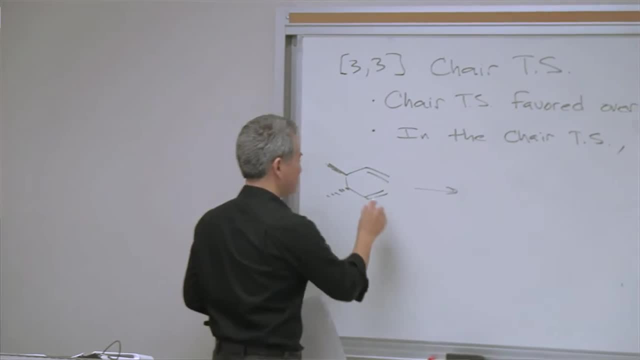 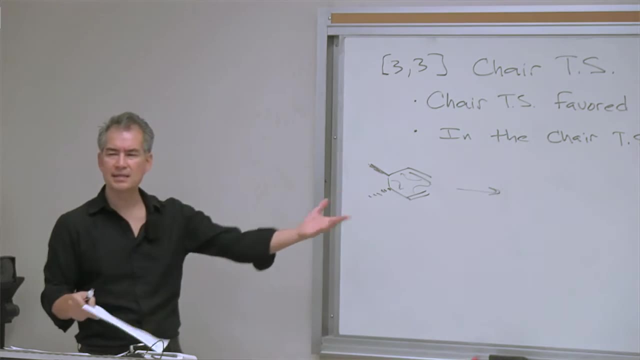 of a substrate for a 3-3 sigmatropic rearrangement. You could push the arrows like this. That's not really the important aspect here. The important aspect is the transition state that leads to these three products. Maybe I should say two products. one of them you really don't see, So here's one product. 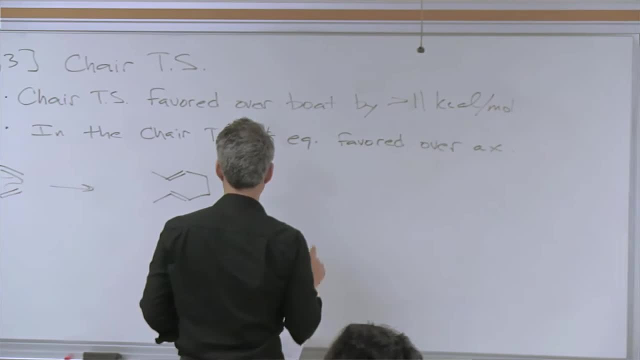 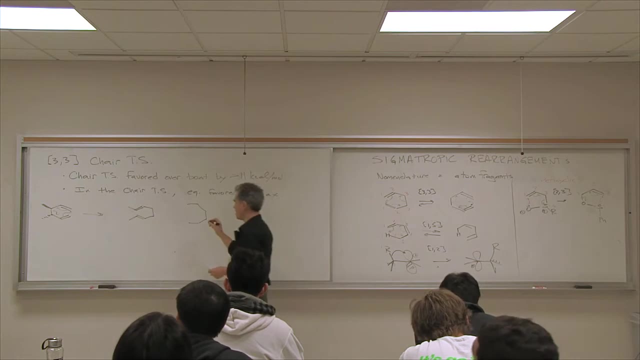 that you can generate. and here's a different product that you can generate. I think it's easier if I try to start to draw an eight membered ring. then you'll see why It's not an eight membered ring. I just wanted it to look. this makes it more easy to see. 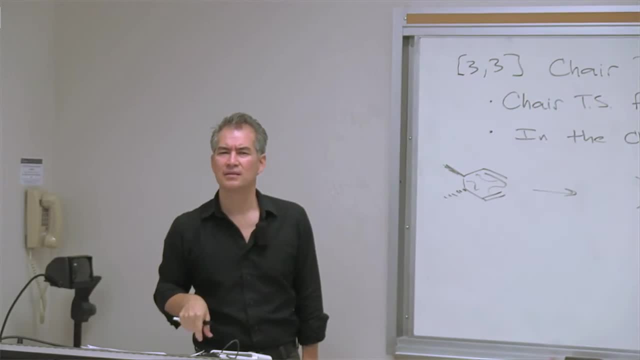 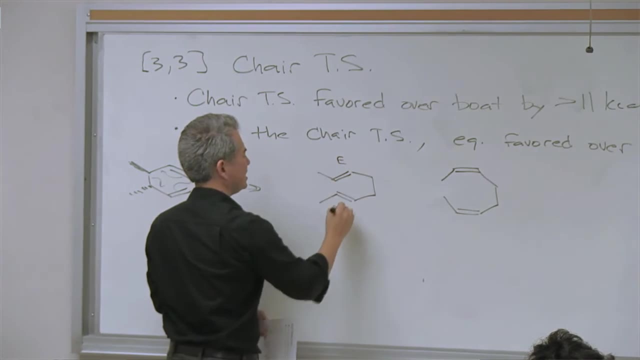 that the alternative product has two cis double bonds instead of two trans double bonds. No, this: these have the same atom connected to it. It's just an issue of two of these. It's just an issue of trans E versus cis, which is the Z geometry, and you can open. 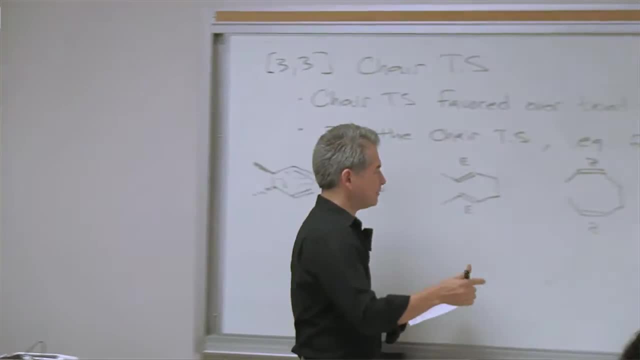 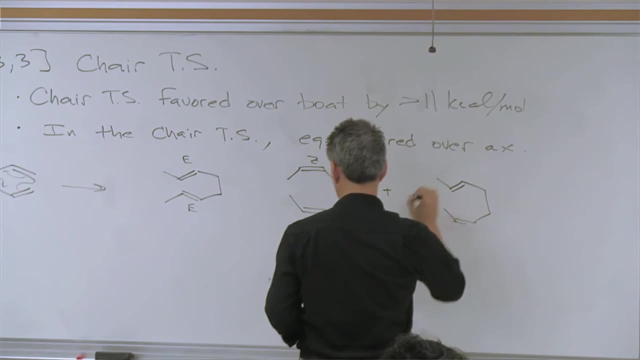 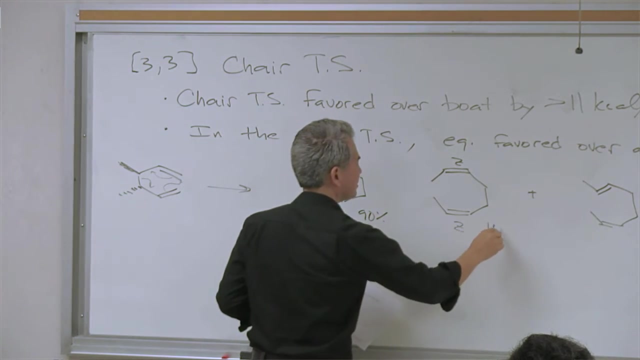 to give either one or rearrange to give either one of those. and there's a third product here that you really don't see and that would be the mixture of the cis and the trans. So the actual ratios, if you run this reaction to low conversion before it has a chance to 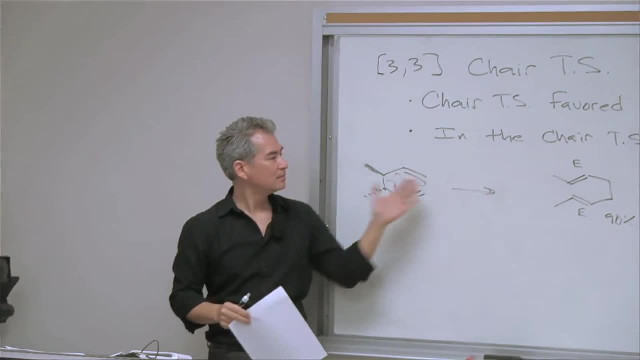 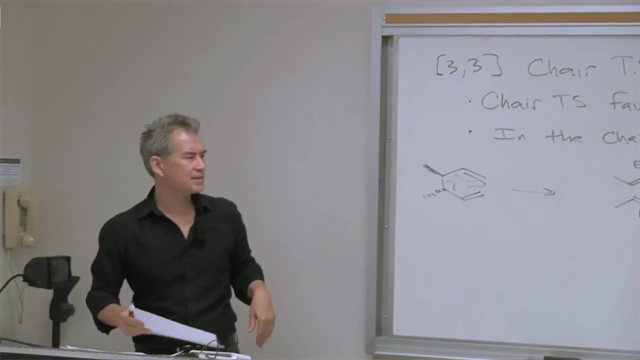 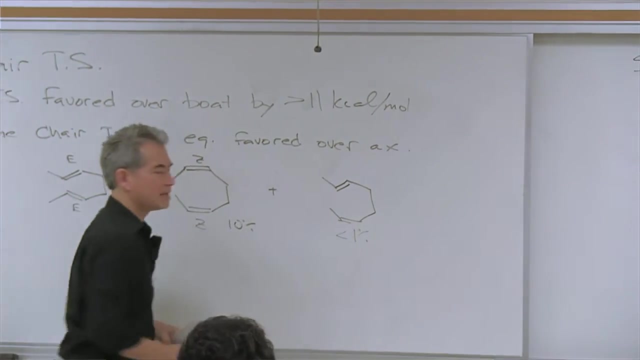 go backwards, right, this is an equilibrium reaction. What you'll find is that, kinetically, you'll get a 90 to 10 ratio of the trans product versus the double cis product, and you get none of this, or at least non-detectable. 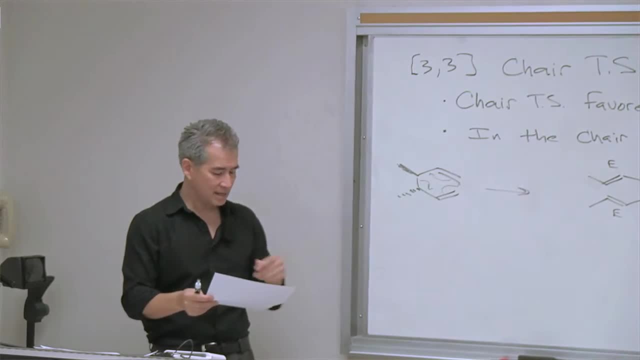 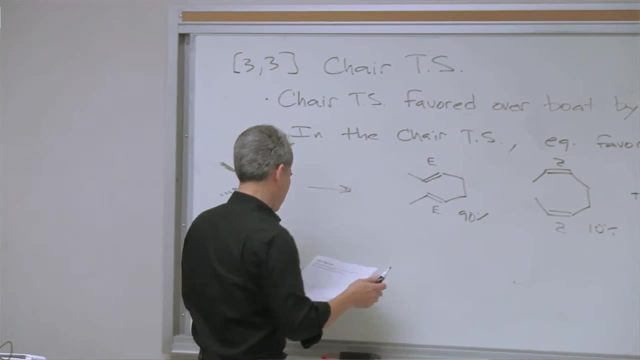 less than 1% of this mixed one where it's E and Z. So let's take a look at the transition states. I'm going to draw some chair and boat-like transition states here so we can see why you'd expect this trans one to be E. 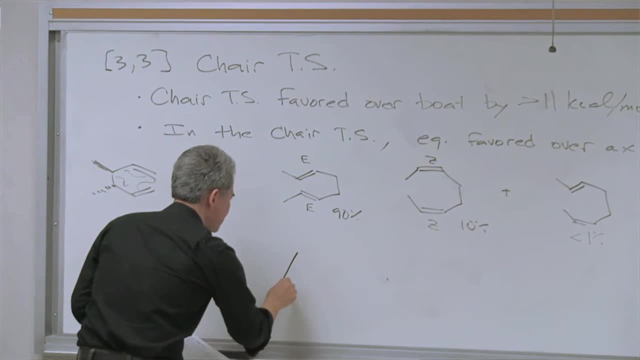 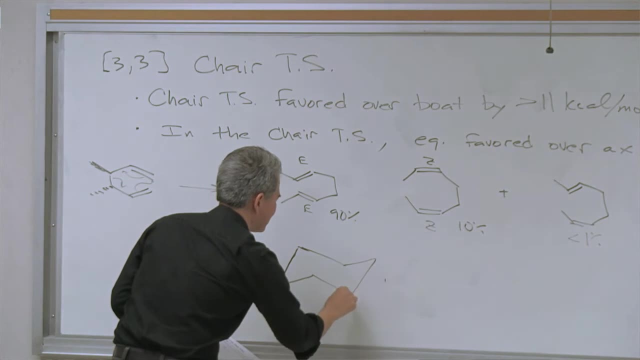 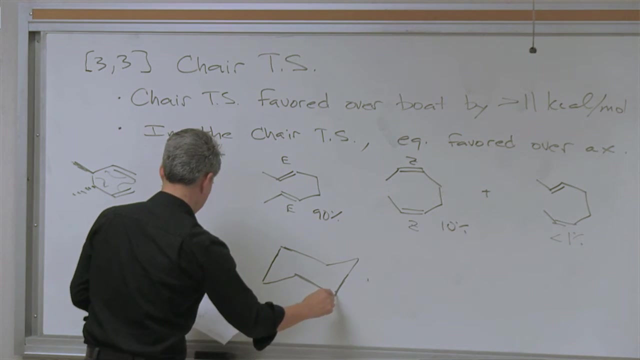 So I'll just sort of lightly sketch a chair, because we're going to erase some bonds here to make them partial bonds. I don't know if I can lightly sketch with a pen here, but you can. These are the bonds that are closer to us. 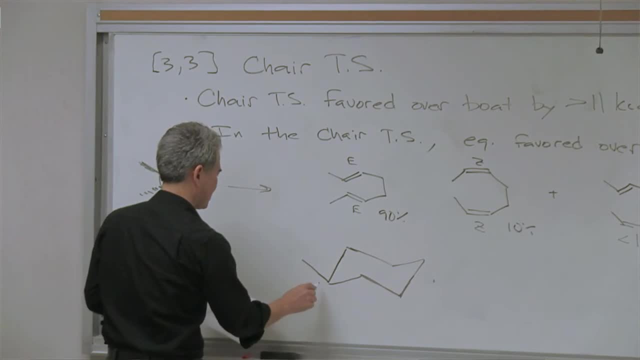 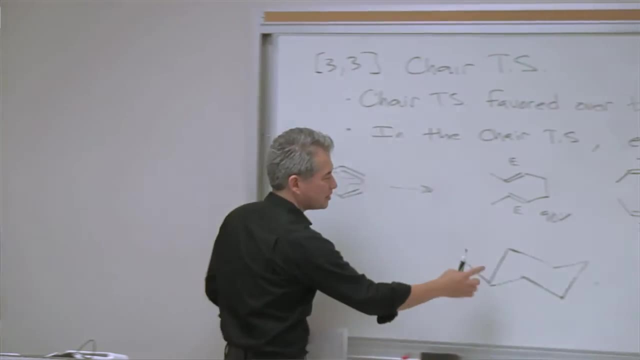 And I want to really focus on here's where I'm going to put my methyl groups in this transition state. Let me just try to make that a partial bond right there, so you can kind of see where I'm coming from. And here's this other partial bond between these two. 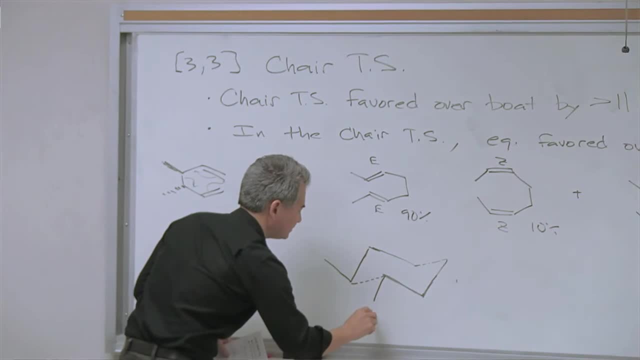 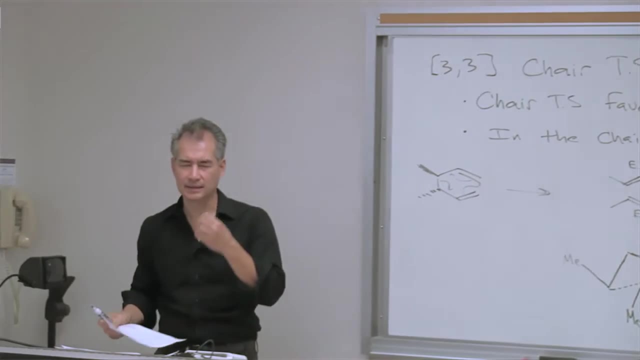 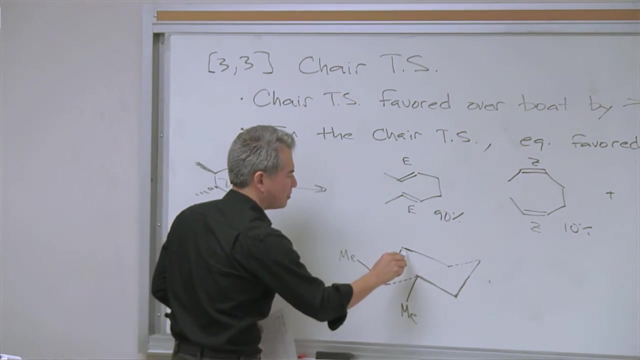 So here's one of the methyl groups, and the other methyl group would be here. Now how do we double check that I've drawn this correctly? Now, if it really is a transition state, I should draw partial bonds here for the pi bonds as I break and form them. 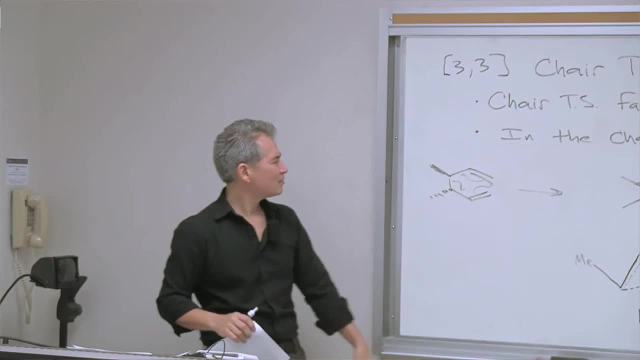 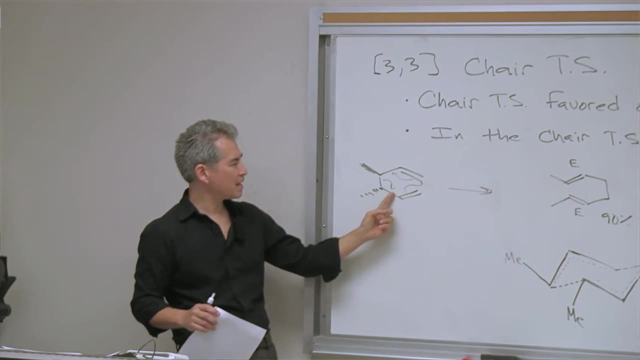 I'm only going to do it for this first transition state because it makes it kind of complex. In the transition state I'm breaking this bond, this pi bond, and I'm forming a pi bond. And in the transition state I'm making a pi bond and breaking this pi bond. 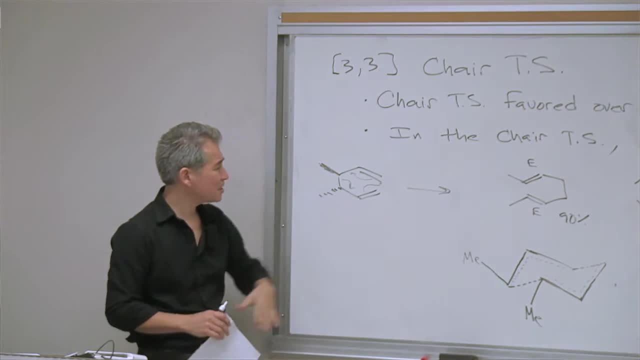 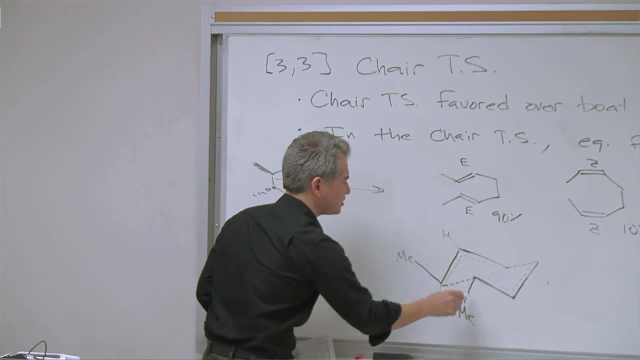 So I can just use dashed lines everywhere. How do I check to make sure I've got the geometry right? What I want to do is I want to focus on the relationship here between these H's to make sure I get this right. You can see that one methyl group on the chair is up the other methyl group on the chair. 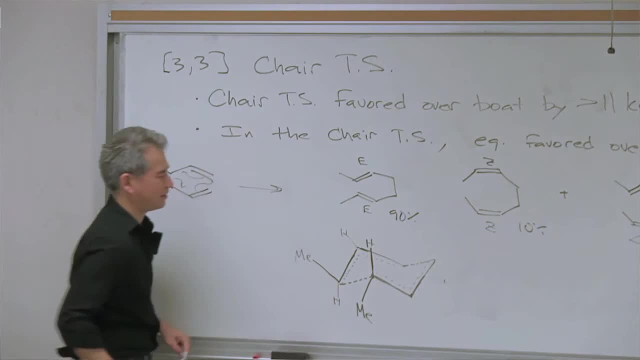 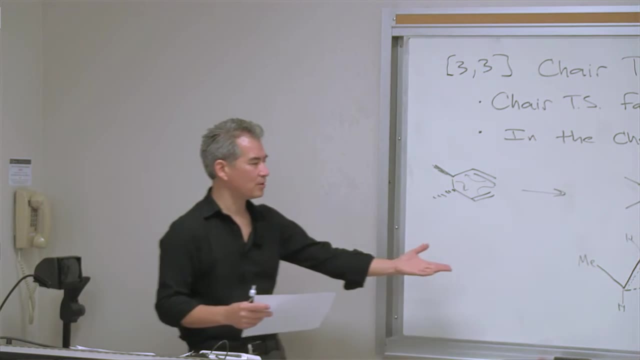 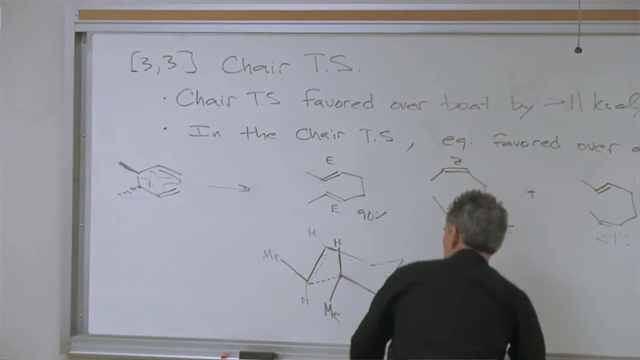 is down And sorry I have to make this H bond long, But in this transition state this looks pretty good. Both of my methyl groups have equatorial dispositions here in this chair-like transition state. But there's another chair-like transition state that I can draw. 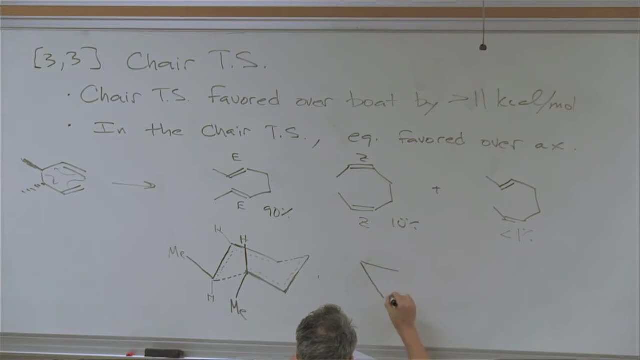 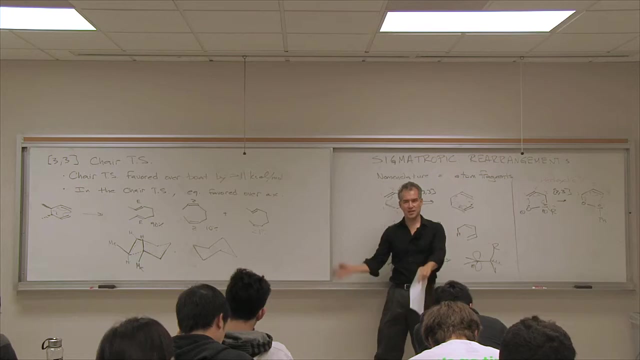 I'm going to draw the ring-flipped chair, And so you might want to sketch this lightly so you can erase one of the bonds. So I flip right. you've got to draw the other flipped version of the chair here in order to make it match what I'm drawing. 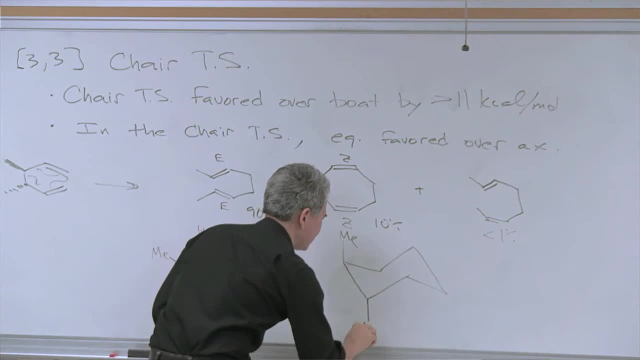 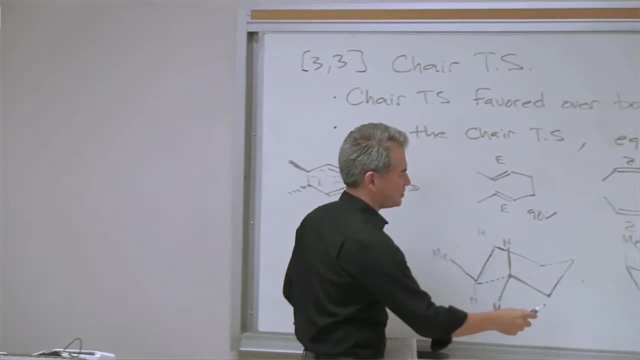 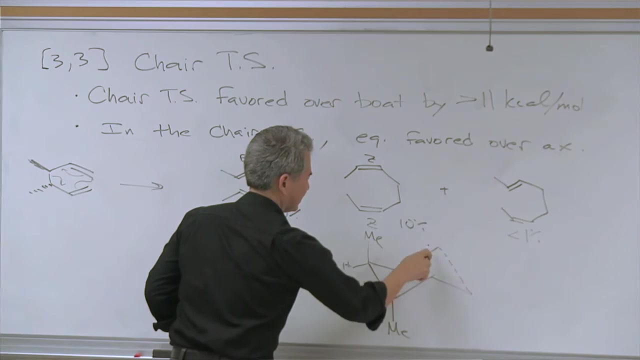 And I'm going to draw both of these methyl groups axial in this transition state. I don't think I need to go into much detail. You should know that axial groups on six-membered rings are disfavored, And here's the partial bond that I'm forming there. 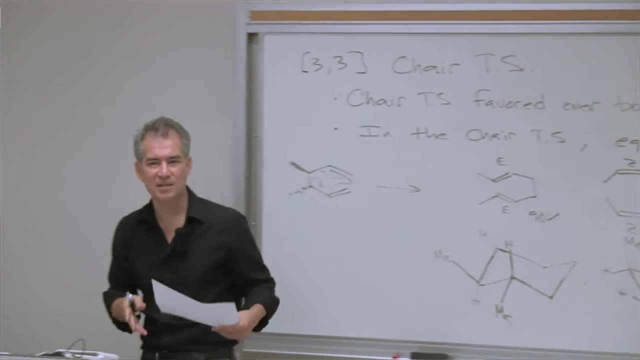 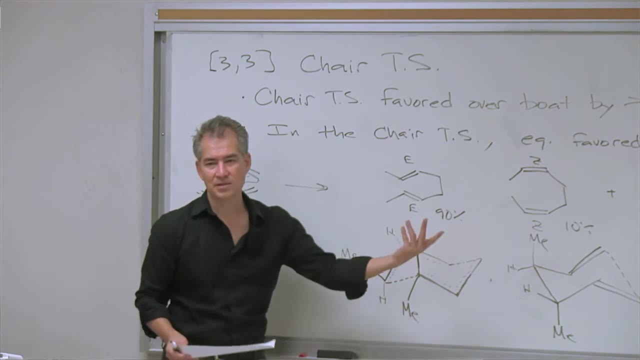 And I'm not going to draw all partial bonds. I'm just going to kind of draw the starting material and show a dashed line where I'm forming a bond here. But this would be the alternative transition. Okay, Okay, Transition state confirmation. that looks like a chair. 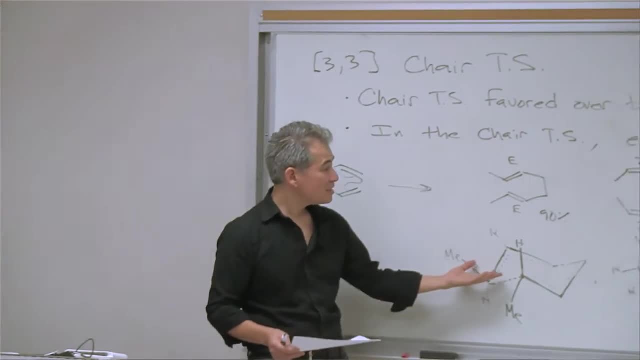 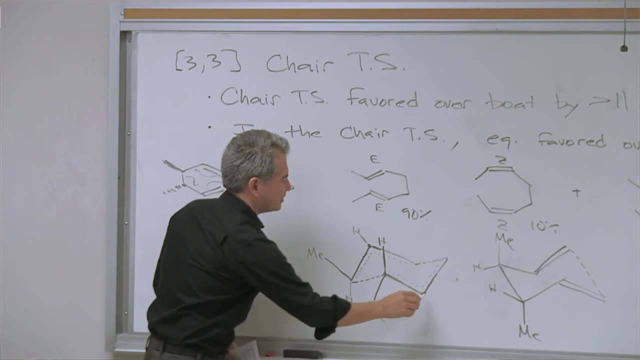 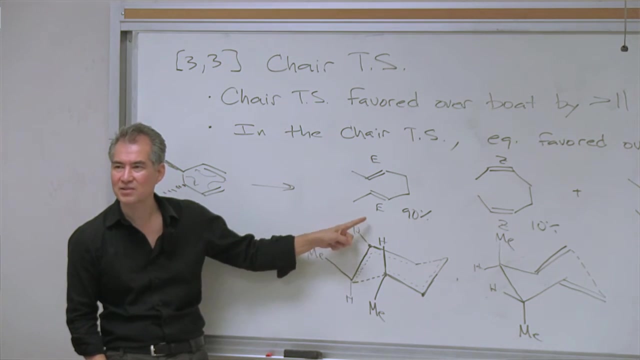 So I've got two chair possibilities And I hope you can see that this is way better Now. I just want to point at this atom right here and this atom right there. This is not really a chair. It's not a chair because there is no pure axial substituent at this position. 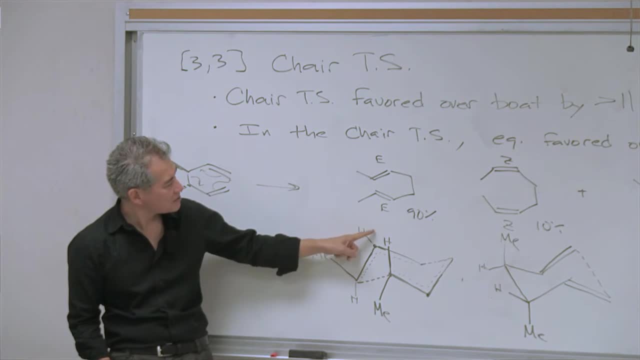 And there's no pure equatorial substituent, And if there's no perfectly axial substituent, because this is sp2 instead of sp3, that means it's not as painful to have axial substituents. It's a 90-10 ratio. 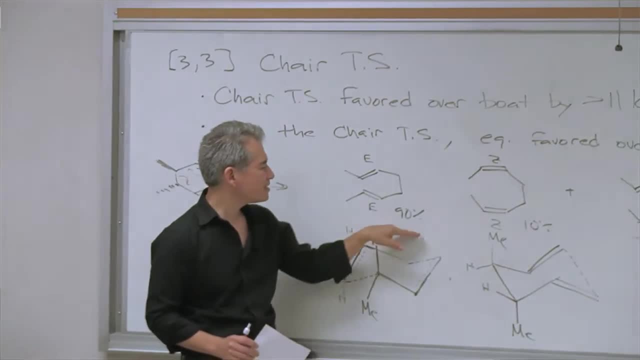 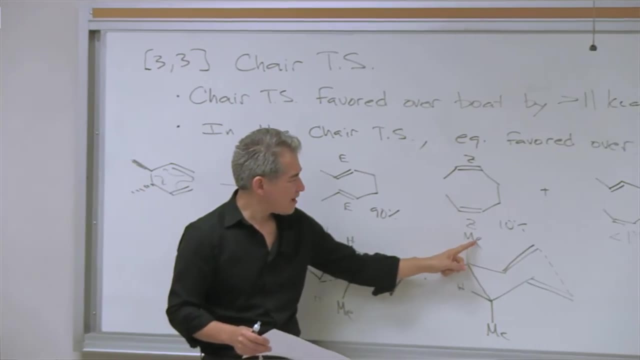 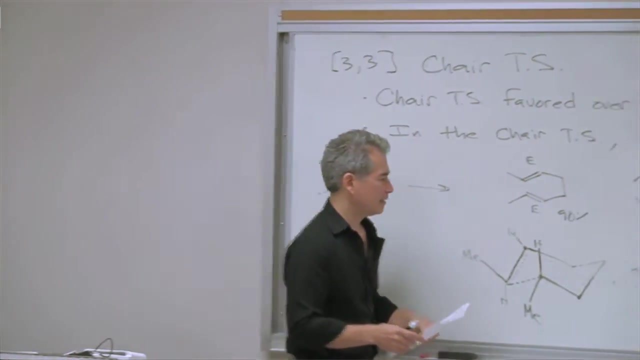 It's not 99 to 1. So you don't get. you know, having axial groups here is not quite as painful as it would be on a perfect cyclohexane where everything is sp3. But it's still pretty painful. 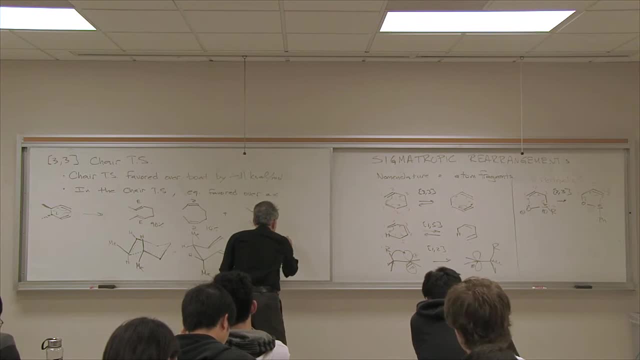 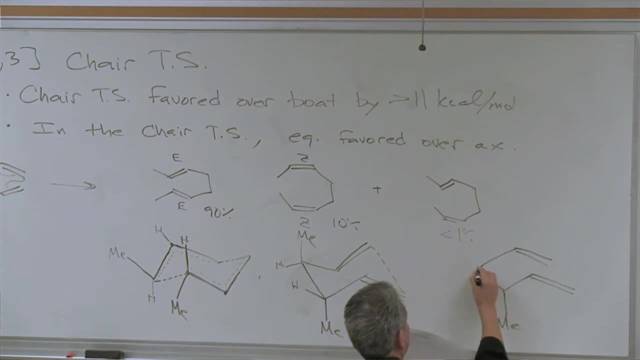 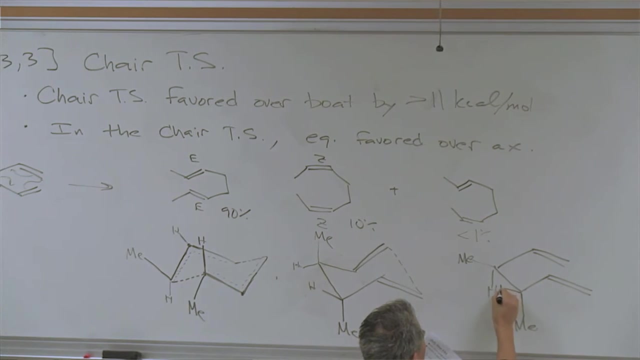 Okay, And then the last possible transition state is just a total non-starter. here I'm going to draw this boat-like transition state And one of these methyl groups gets to be kind of pseudo-equatorial. The other methyl group has to be axial. 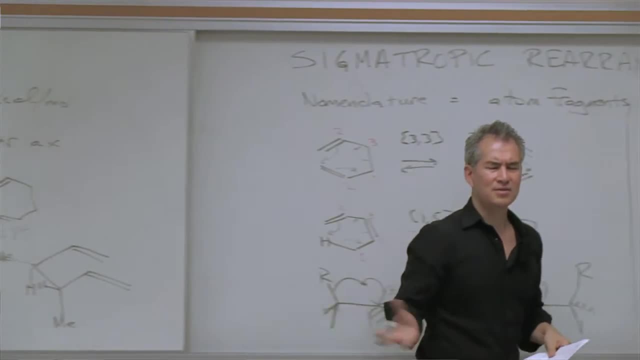 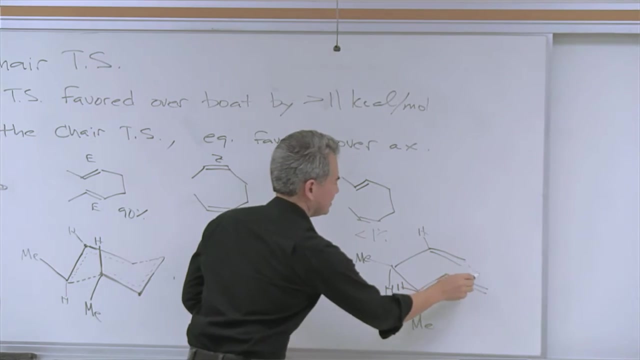 But that's not the problem. The problem is that it's boat-like, And so you see almost none of the product from the boat-like transition state. And so if you look at this here, this transition state, this boat-like transition state, see. 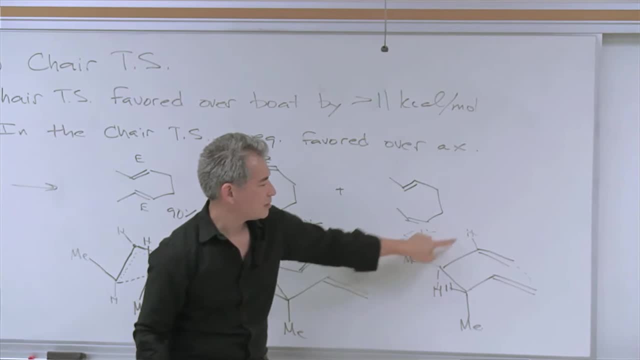 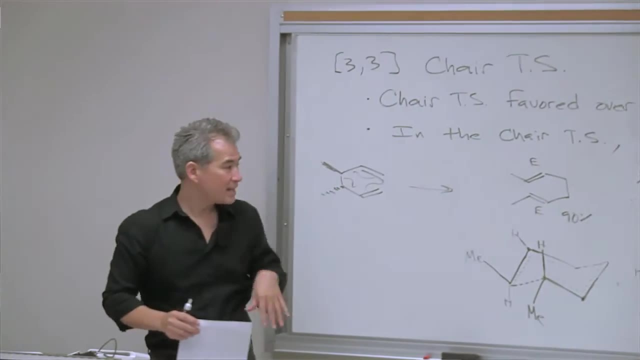 the two H's. They're anti. That's going to give you a trans double bond there. If you look at the two H's over here, They're cis. That's going to lead to the cis double bond. Sometimes, if you can't keep track of whether you're drawing the right isomers, look at. 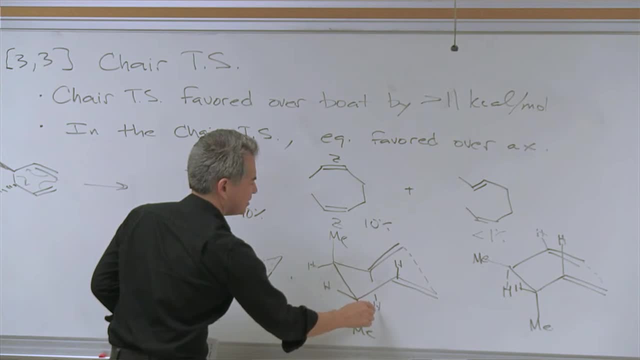 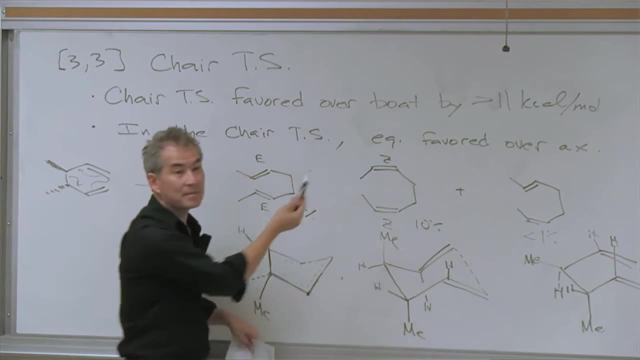 the relative substituents. So let me come down here. These two H's are cis And they're cis in the product. These two H's are cis to each other in the transition state. They better be cis in the product. So sometimes drawing the H's which aren't drawn for you will help you make sure you're. 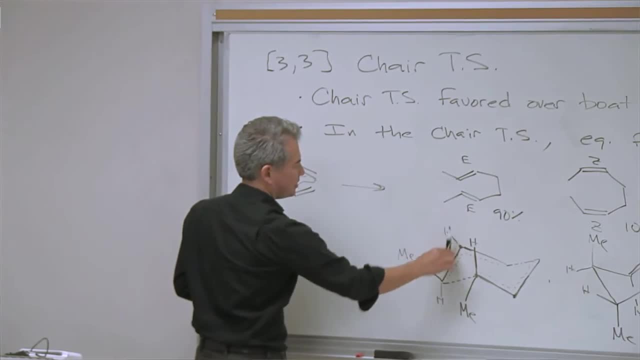 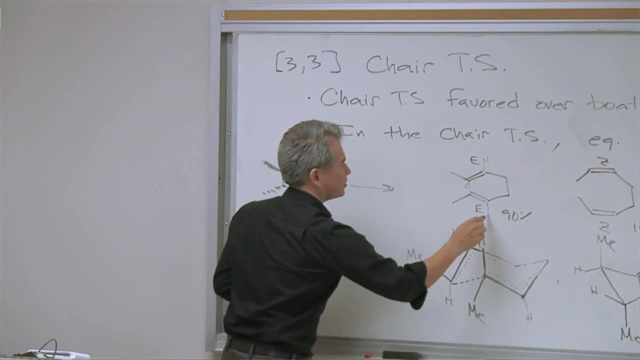 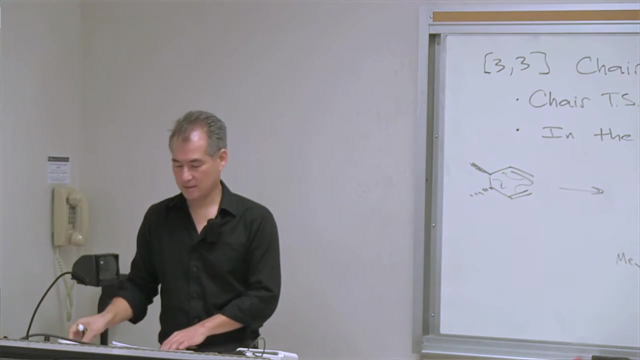 keeping track of the geometry. And again, in this transition state the two H's are trans And here they're trans in the product. These two H's are trans to each other And they're trans in the product. So that's kind of one of the big issues with these 3-3 rearrangements is keeping track. 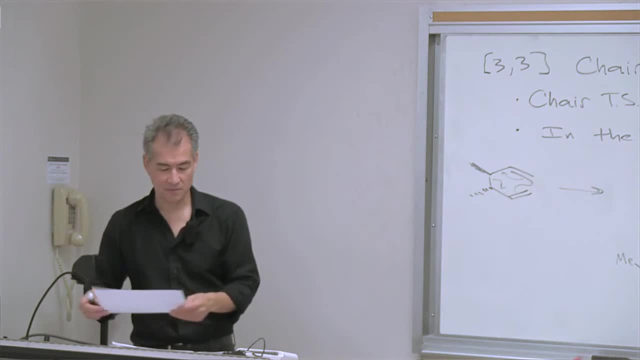 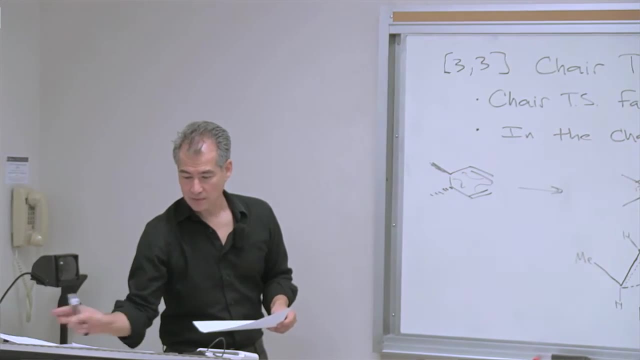 of double bond geometry and seeing how that correlates as you go from starting material to product. OK, Let's look at the orbitals that are involved in this transition state. OK, Let's look at the orbitals that are involved in this transition state. 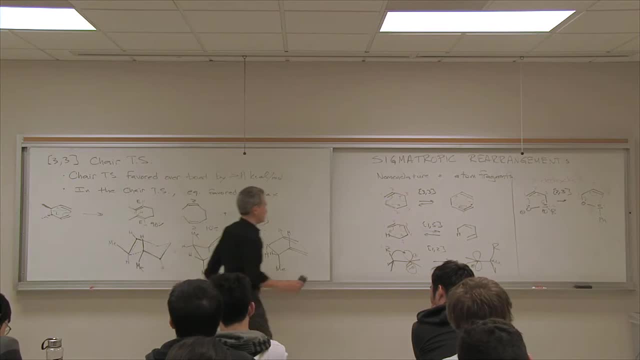 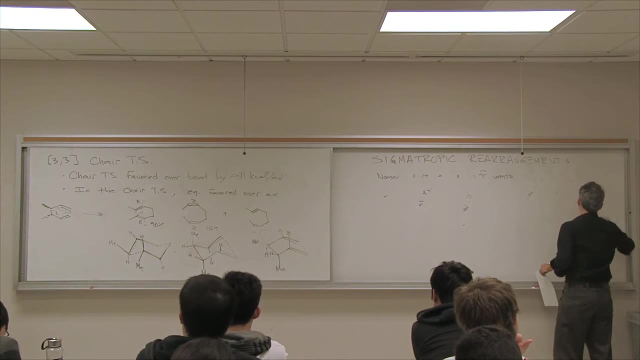 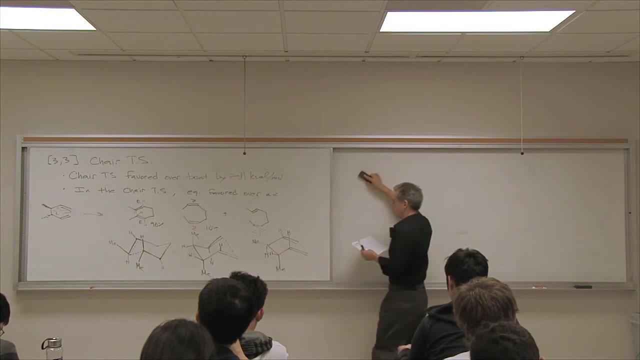 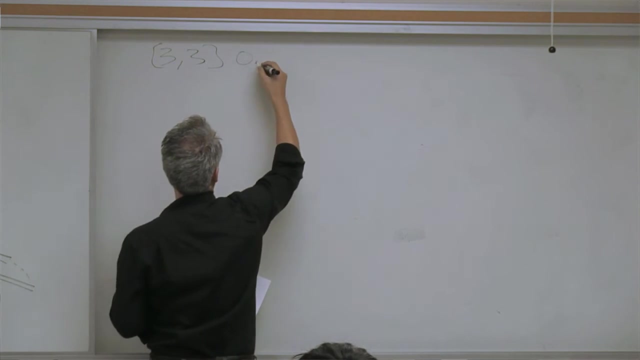 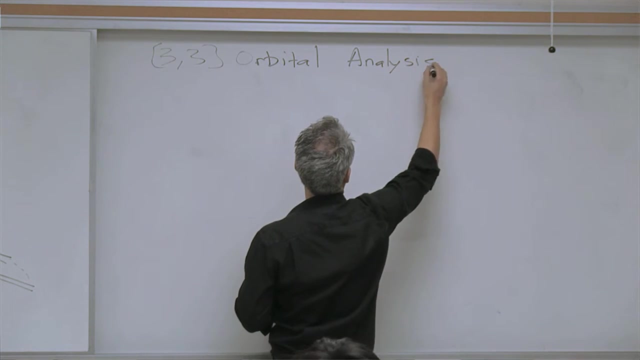 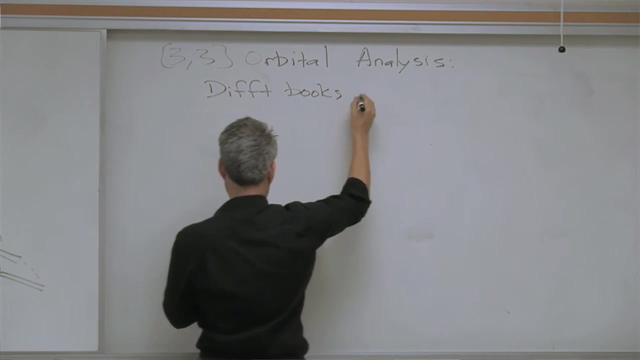 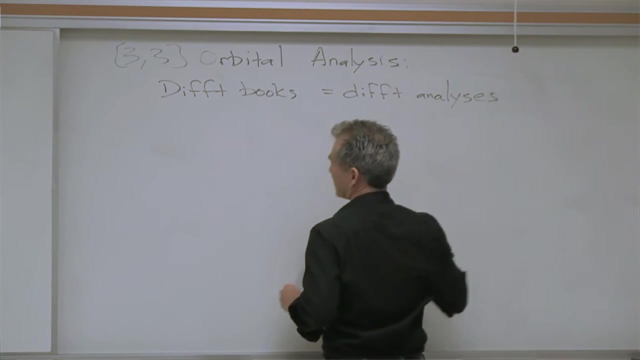 OK, Let's look at the orbitals that are involved in this transition state. OK, So here's this simple 3-3 sigmatropic rearrangement. So this is all of theacement- the right arrow, right node- And it's aggravating because, as you look at one book versus another, they analyze the orbitals. 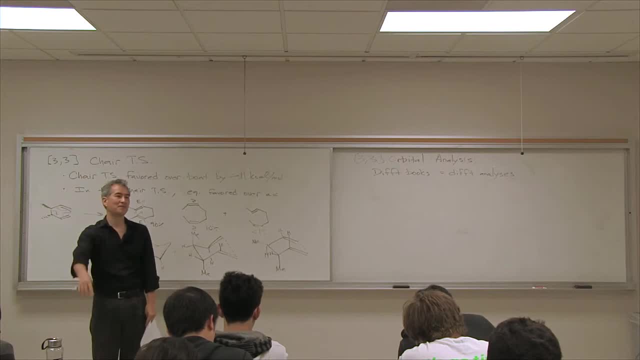 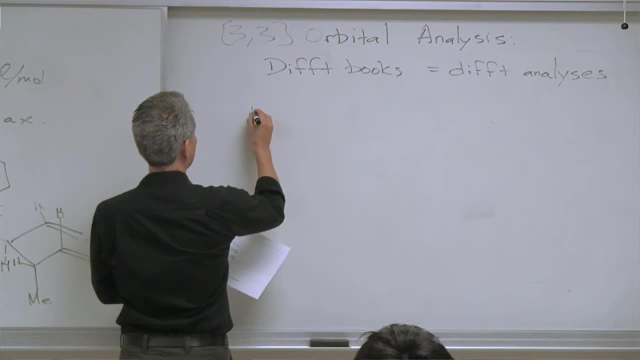 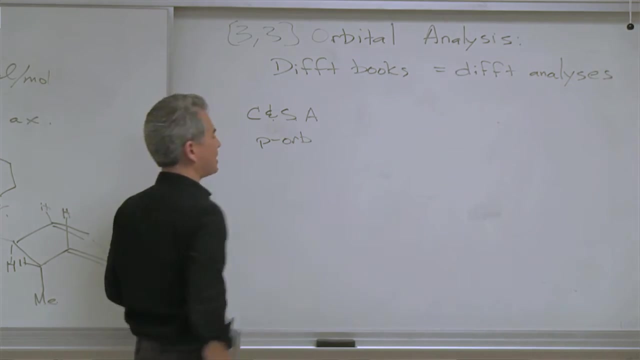 in different ways. It's so aggravating and it's going to confuse you. Let me try to resolve that confusion so we can try to see what's going on with this different type of orbital analysis. So if you look in the Carrion-Sundberg book, the analysis is based on p-orbital interactions. 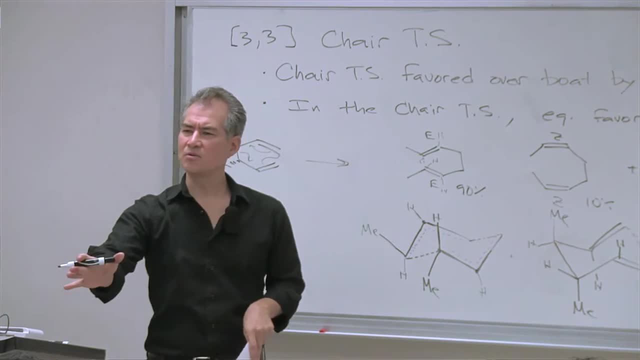 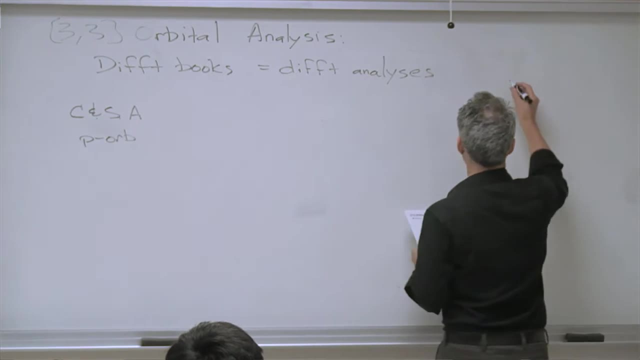 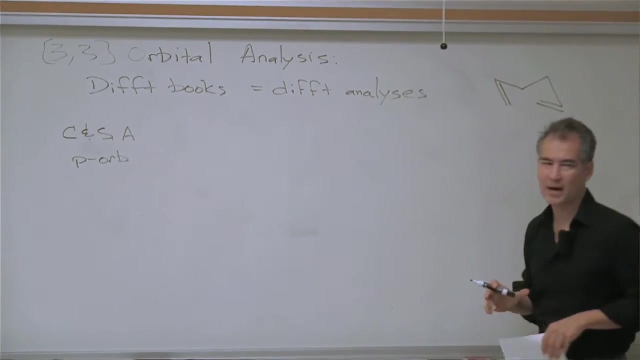 You take every single bond that's involved in the transition state and you try to break it down to look like a p-orbital. So let me go ahead and draw out the, just the simple reaction, without any orbitals. Let's just envision that we're talking about a 3, 3-sigmatropic rearrangement and in that 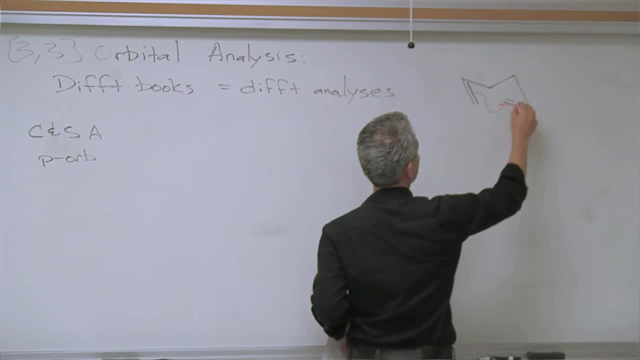 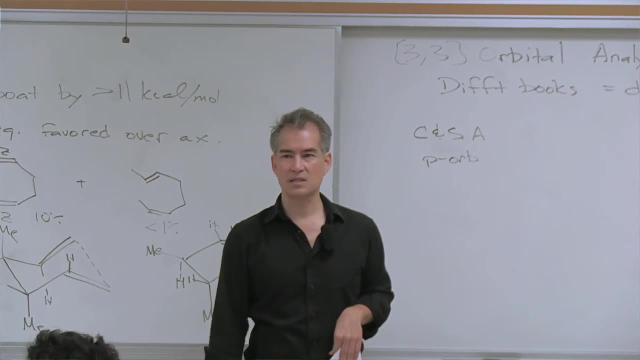 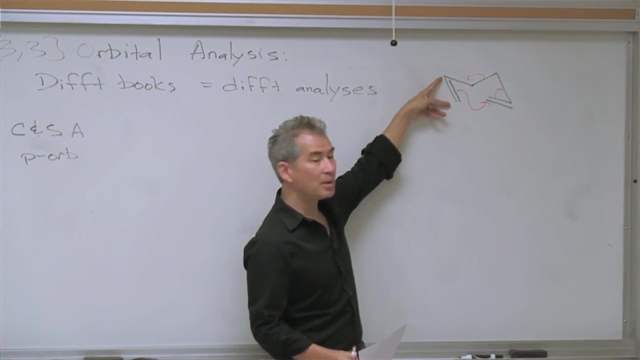 arrangement. this pi bond is attacking this other pi bond. This is giving its electrons over here and you're breaking a sigma bond in the process. Three curved arrows, it's a six electron process, But you can try to imagine that this pi bond that's breaking here is actually composed. 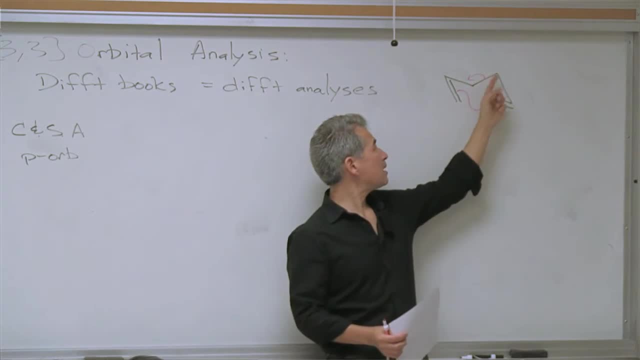 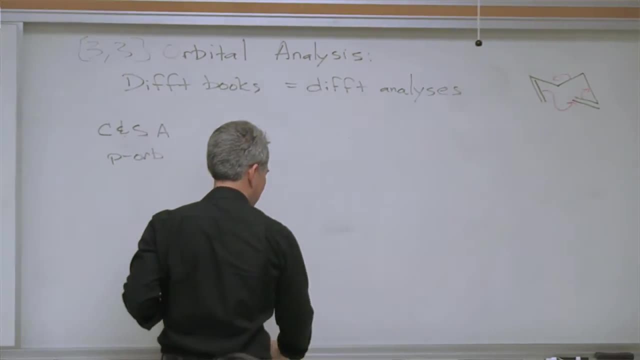 of two p orbitals. You can imagine that this sigma bond is an interaction of two p-like orbitals that are poking end-to-end, and so let's break those bonds down to look like that. That's what Carrion-Sundberg does. 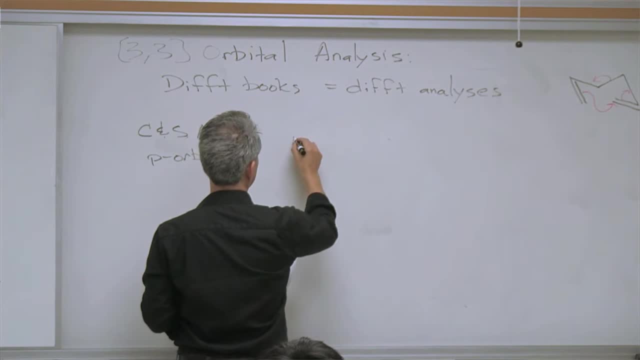 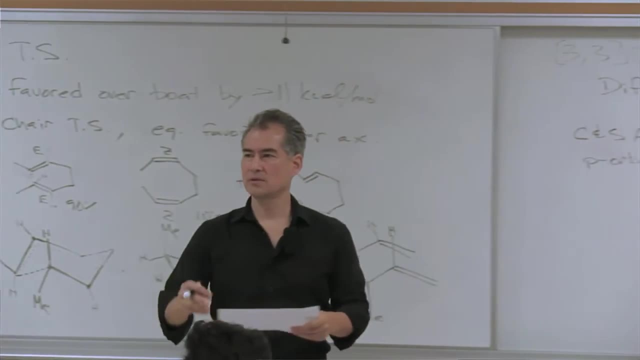 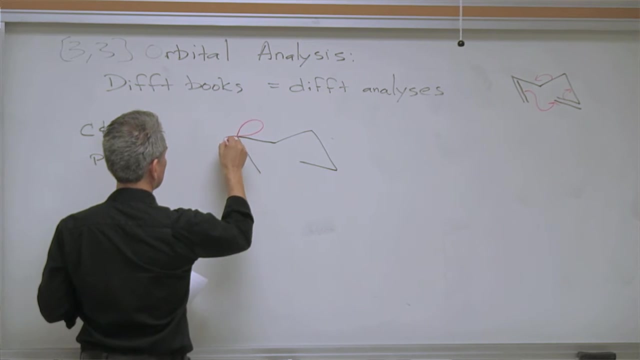 and other books. Let me go ahead and redraw that, that same transition state here, And I'm going to draw those p-like orbitals that are involved in the transition state. So over here I'm going to take this, that pi bond, and I'm going to draw two p-like orbitals and phase them so that they look like a. 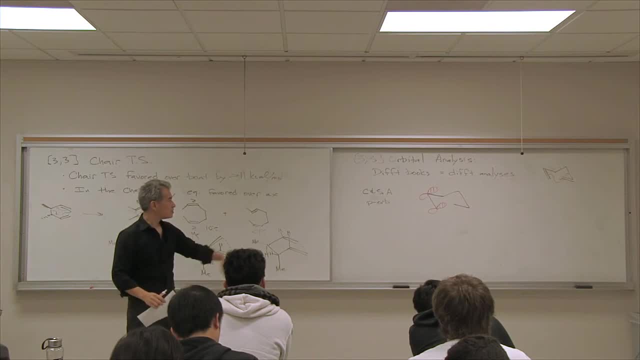 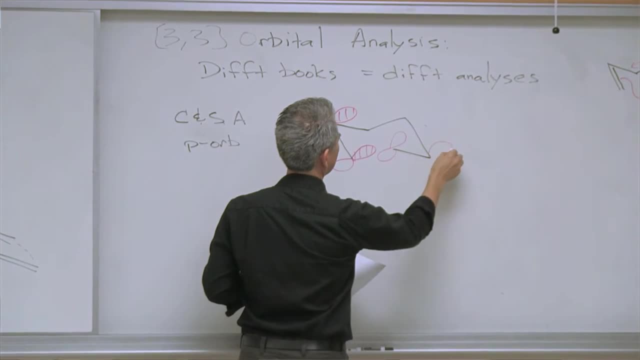 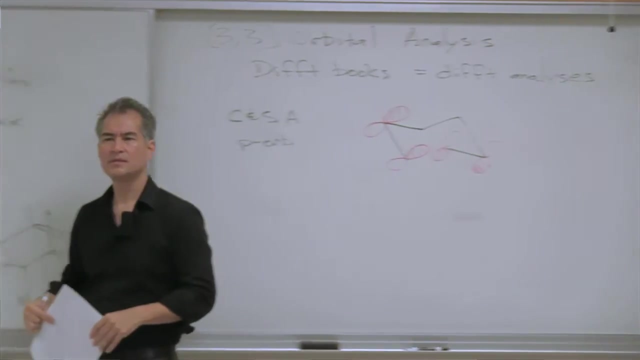 pi bond. Right, If those two p orbitals with that phasing interact, you'll end up with a pi bond. And then over here I'll take this other pi bond and do the same thing On this one. I'll hash the bottom parts of these orbitals And then the last. 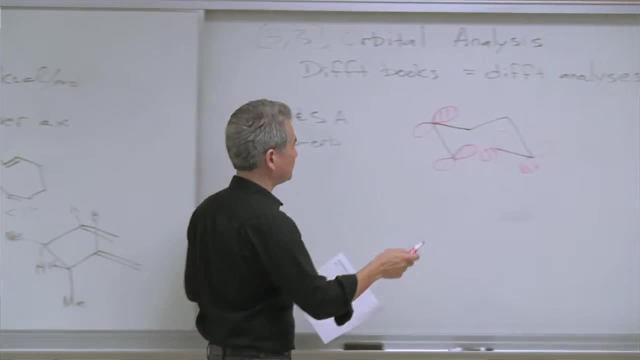 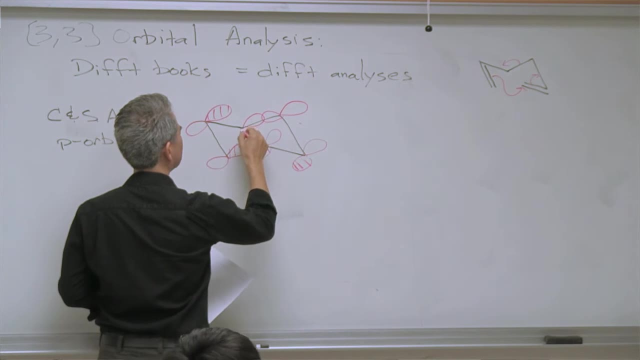 bond is the sigma bond, And so how do I phase, how do I draw the p orbitals to make it look like a sigma bond? I'll put them end to end. That's kind of like the sigma bond there, And I'm going to hash the. 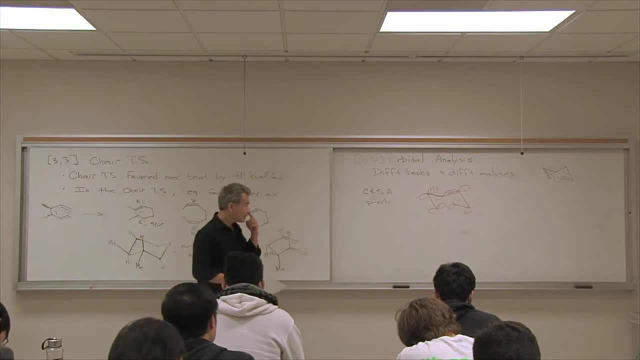 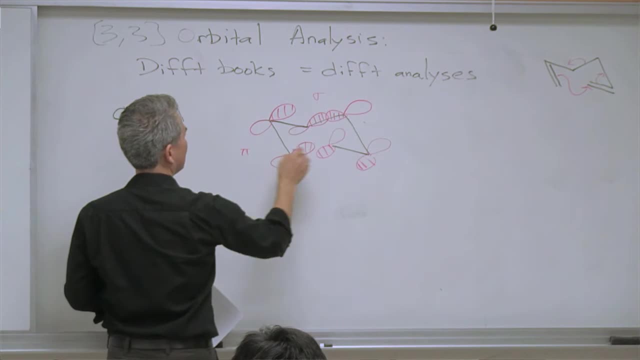 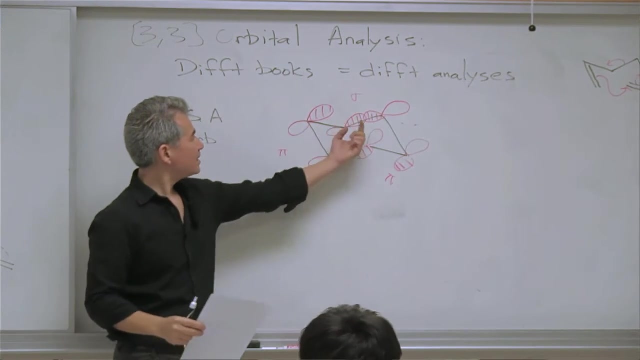 inside in between. so the phasing. And now, if I look at this, you know if I've drawn, if I've correctly drawn these things so that they look like a sigma bond and a pi bond, whoops, and down here a pi bond, I can arrange these so that there's a continuous 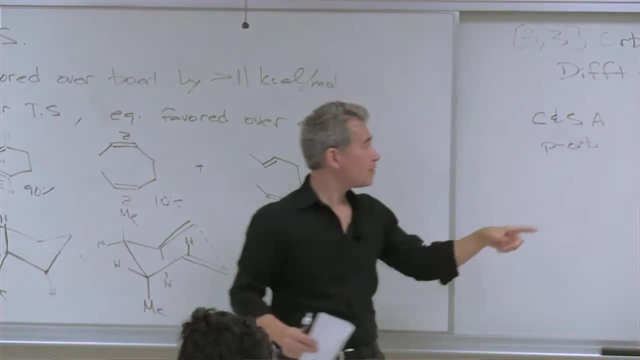 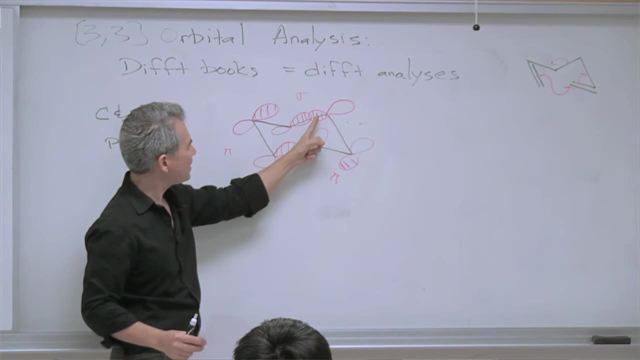 overlap of like phased orbitals. See how all the hashed ones here interact Top face, top face, top face of the yellow fragment And over here on the bottom face I've got this sort of hashed, hashed, hashed. It works out beautifully. The orbital symmetry is perfect and 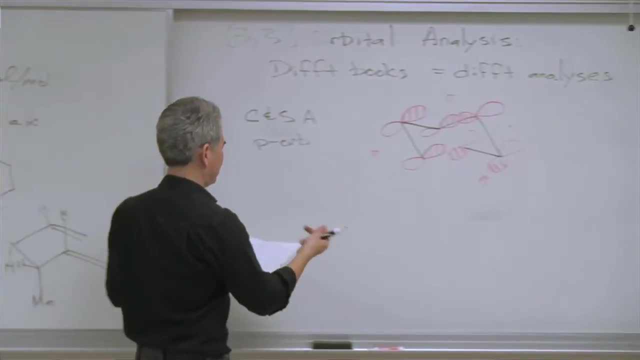 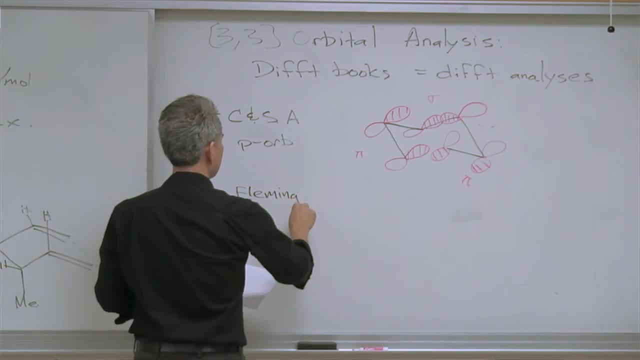 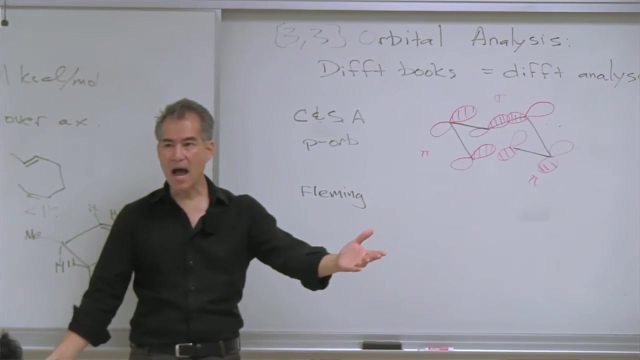 that's why you can rearrange through these kinds of transition states in a 3-3.. So if you look at the Fleming book, of course Fleming is all about frontier orbitals and canonical frontier molecular orbitals, Sigma pi, p orbitals, lone pairs, sigma star, stuff like that. 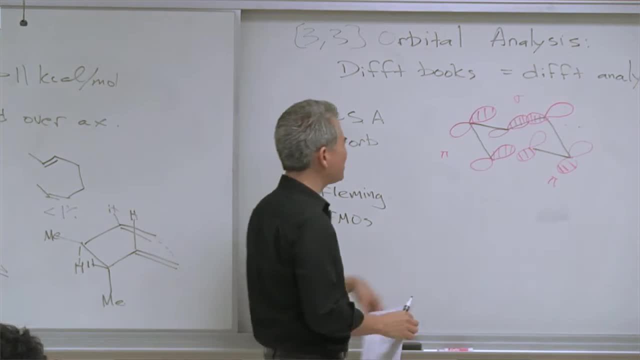 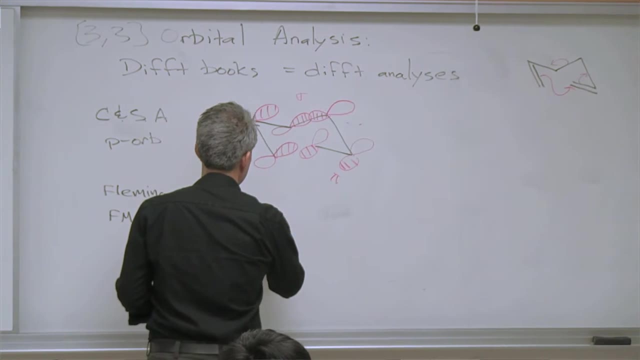 And so Fleming says: well, look, I'm not going to draw p orbitals. I know it's a pi bond, so why don't I just draw the pi bond? So if you look at the analysis in the Fleming book, you draw the same. 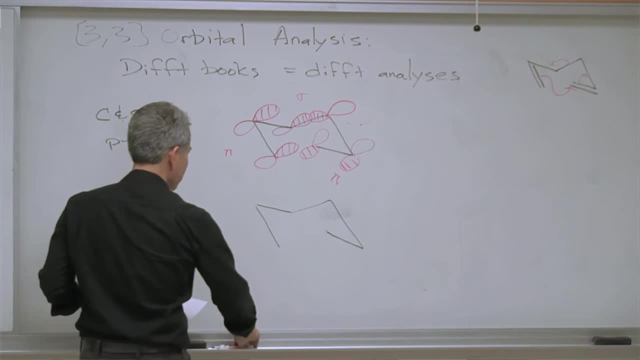 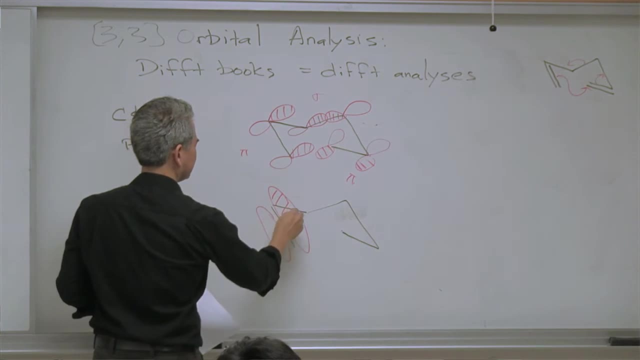 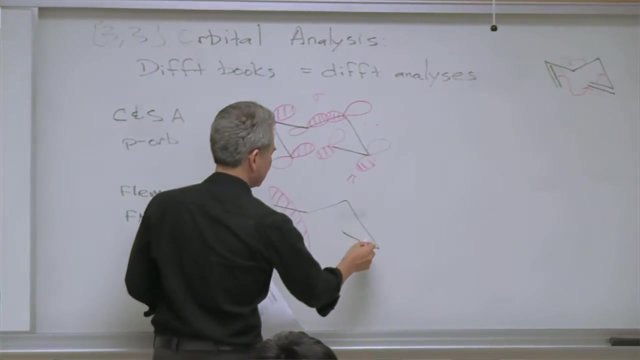 chair, that doesn't change, and then we'll just sketch out a pi-like orbital. Let me sketch it out. Here's a pi-like orbital. If two p orbitals combine together, you'll get a pi-like orbital out of that And over here on my on the other side. 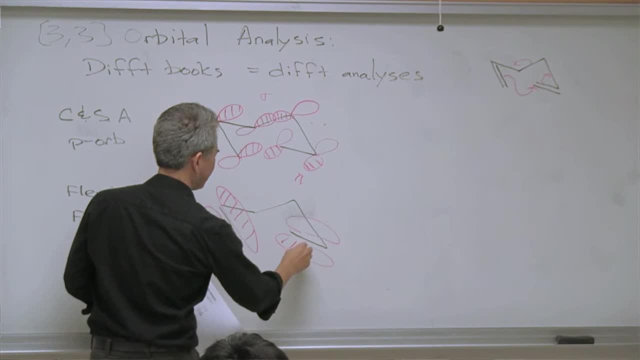 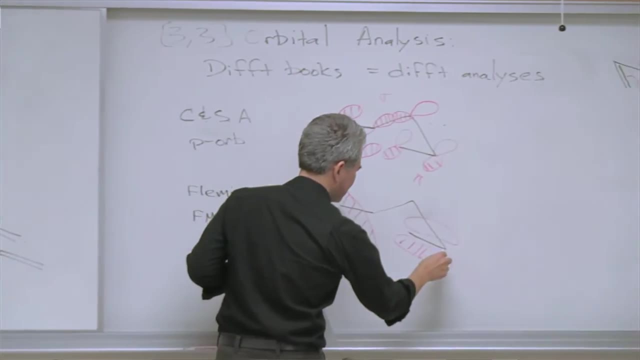 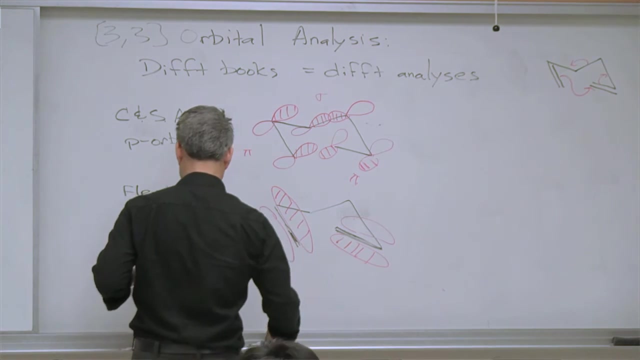 I'm going to draw a pi-like orbital. This time I'm going to phase the bottom. Let me try to make this three-dimensional by showing that this bond is closer to us. There we go. That looks kind of like it's getting closer to us. 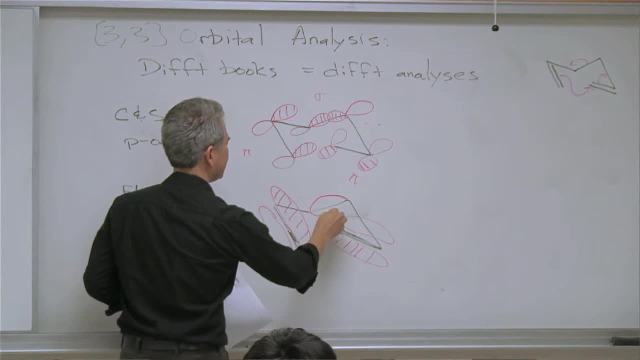 Okay, and then finally the sigma, the sigma bond, you've got electron density in between the two carbons, and then you've got unlike phasing on the back end here. Oh wait, let me, uh, let me change that so it's hashed in the middle. 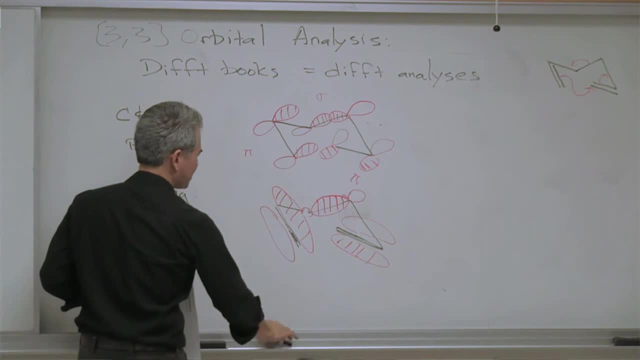 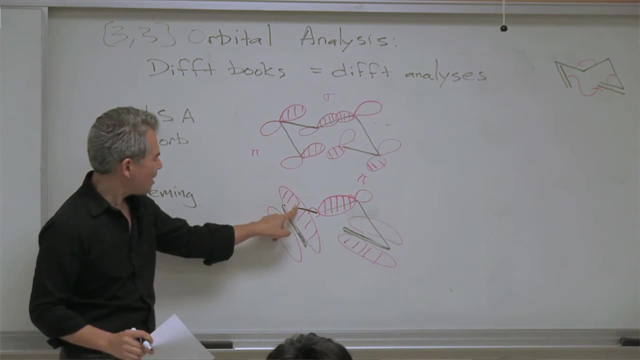 Okay, so now let's focus on this pi-like, this three carbon fragment here, this aloe fragment there, I don't know it's it's probably not so obvious here. Let me hide that behind there. So I've got this pi-like orbital here. 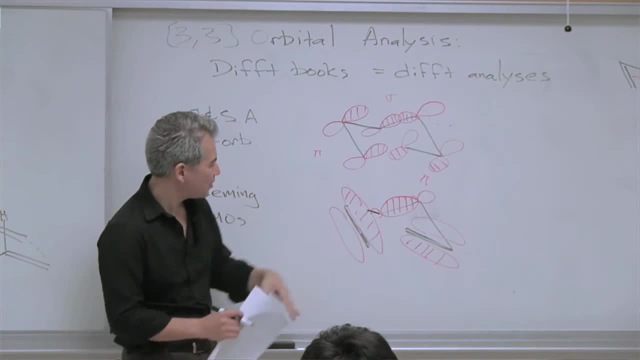 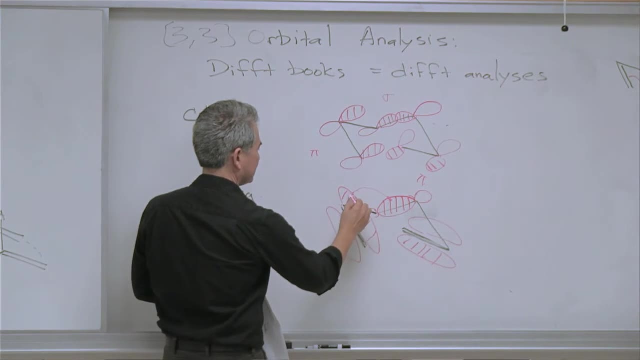 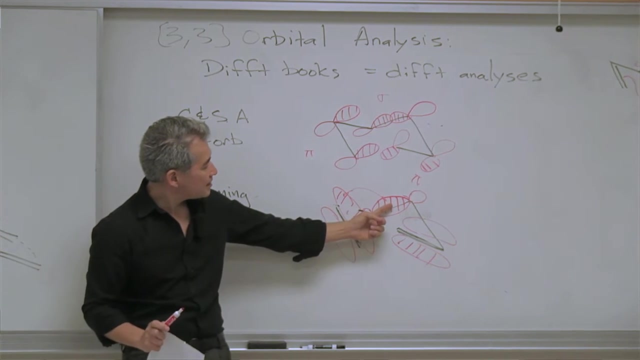 like the pi bond and it's got the same phasing as this sigma bond. It can overlap on the top face of this aloe fragment. Um, I can get a constructive, active interaction between the top of this pi-like orbital and that sigma bond And this. 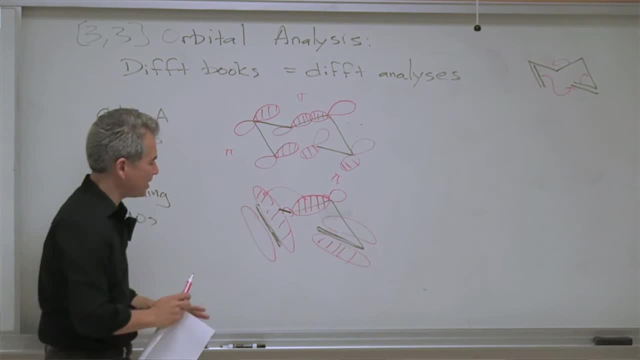 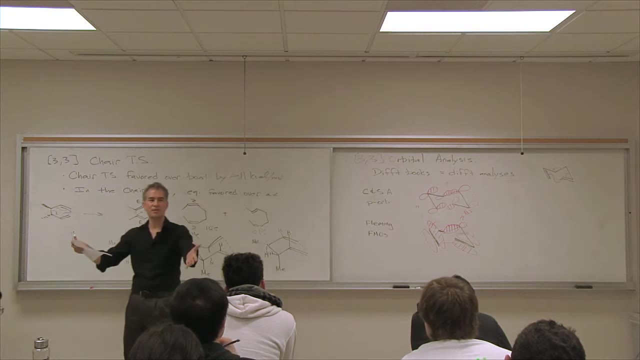 sigma bond can interact with the bottom face of this pi bond, which can also interact with the top face. There's- I mean there's- a complete network of orbitals here that all have the symmetry matched and it works perfectly. And it works perfectly because, if the analysis 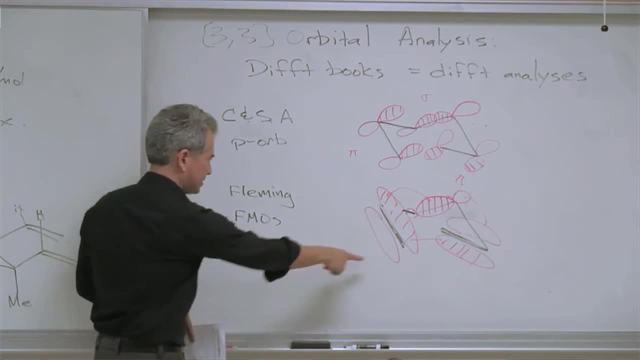 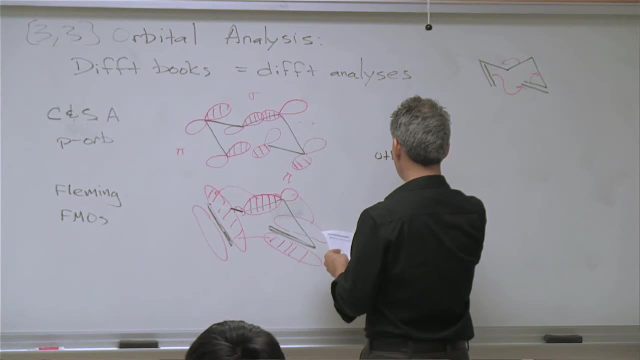 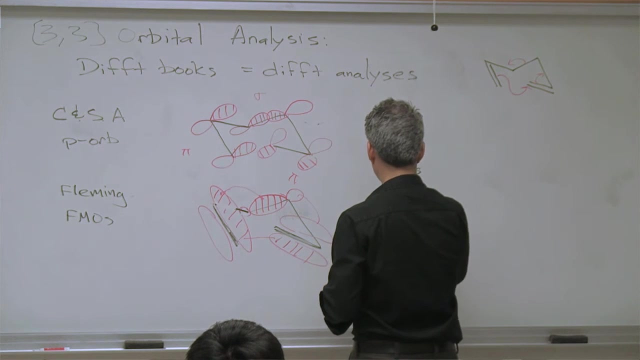 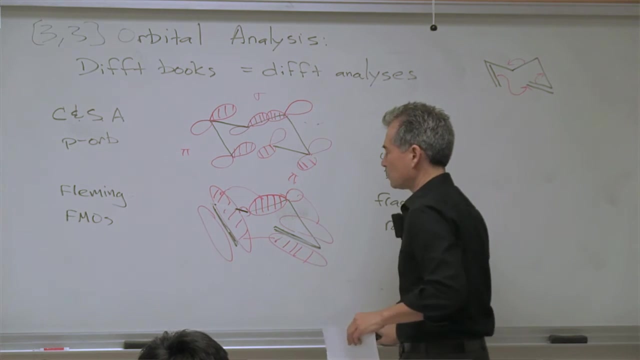 worked here, it has to work there. Okay, there's a last way to analyze these things, and I don't have room underneath here, so I'll try to sketch it over here on the side. So the Fleming book does FMOs, Other books and other websites. break these down into fragment radicals In. 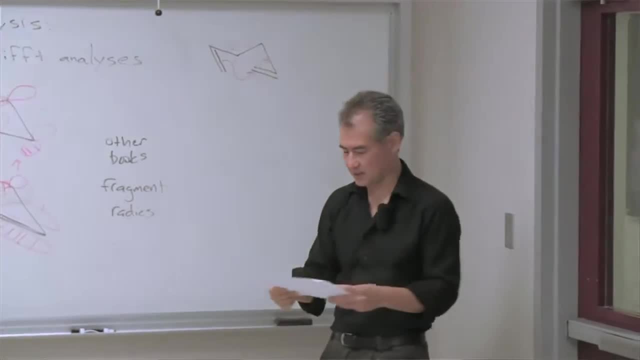 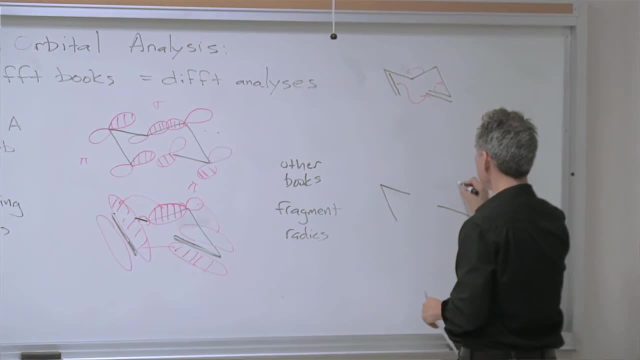 other words, it just fully breaks it down into two, three atom fragments. And so if this really is just two allyl radicals combining together, it's going to be a very, very complicated analysis. Then all you have to do is understand what the orbitals look like for an allyl system. 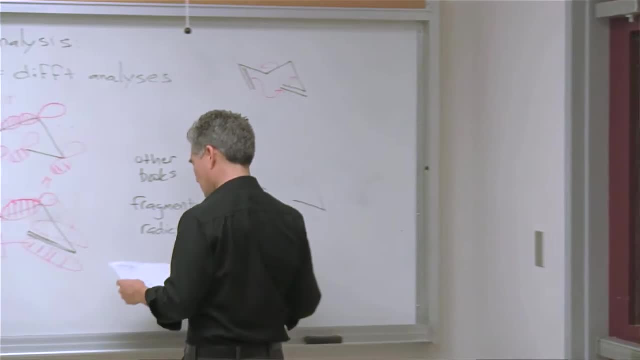 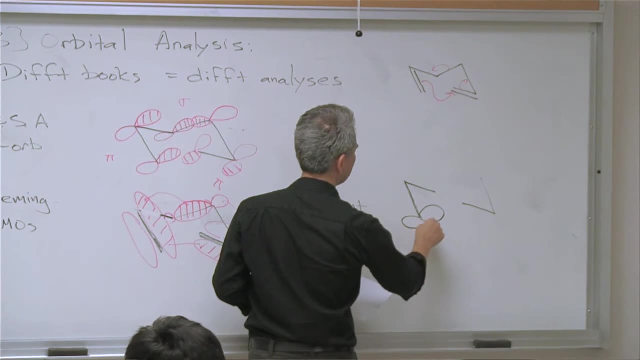 You just need to go back to Hooke's theory and say: what does an allyl, what do the orbitals, what does the pi-like orbital look like for an allyl fragment? So here's one allyl fragment and you'll recall from Hooke's theory that an allyl fragment has this kind of phasing. 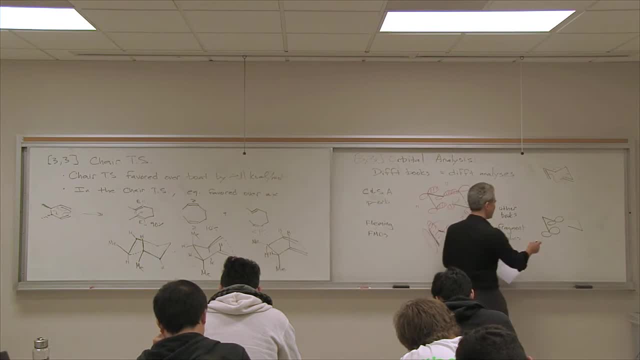 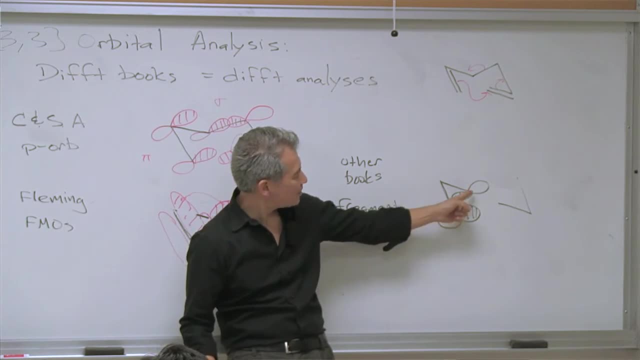 There's a node in the middle and all you really care about is the phasing on the end. is it the same or opposite? Well, it's opposite. So on one carbon atom, it's형- It's a single atom hashed part up. On the other carbon atom, it's hashed part down If we draw the other. 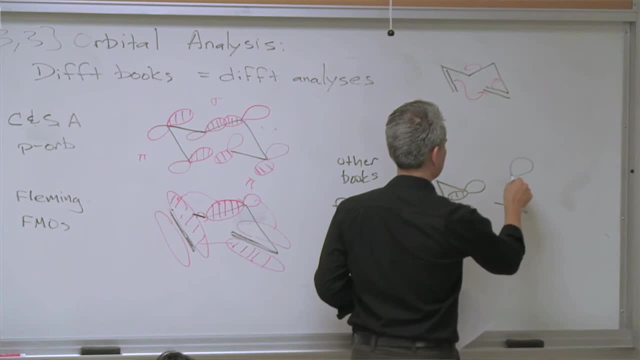 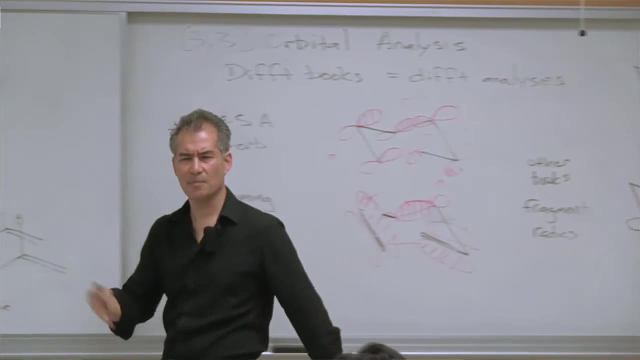 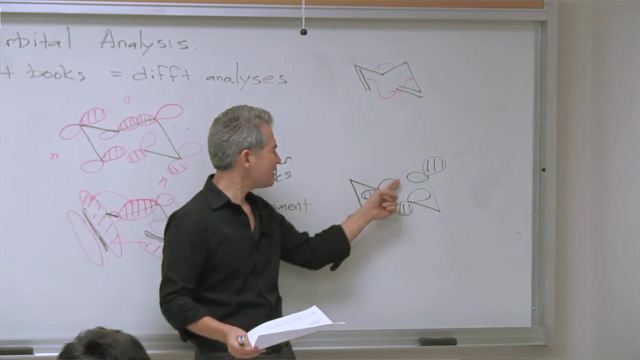 aloe fragment. in the orbital phasing it's got to be the same where hashed part is up on one side and down on the other side And it's arbitrary. but we're going to choose the phasing combination. But I could have reversed this, But I'm going to choose the 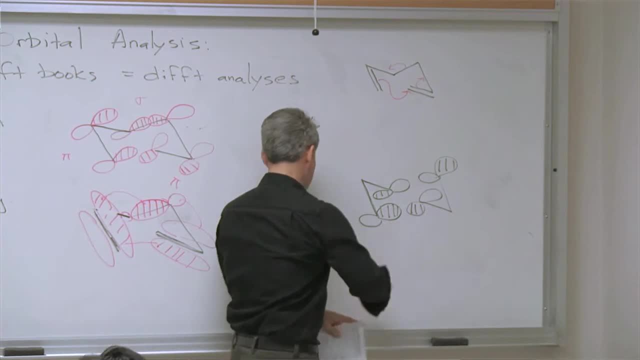 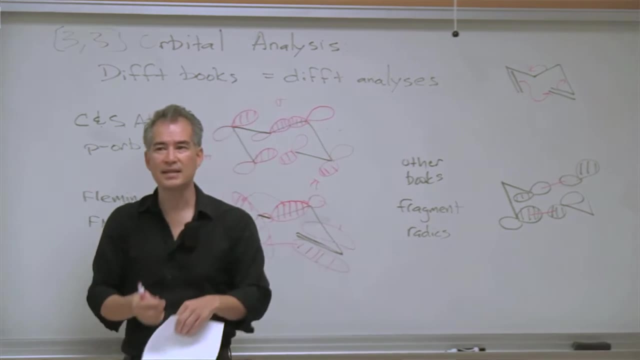 phasing combination where I'm going to have bonding So these can interact. Sorry, I should have used the glorious red color here but I forgot to do that. But you can see that there's a way to combine these so that the bottom face of one interacts with the top. 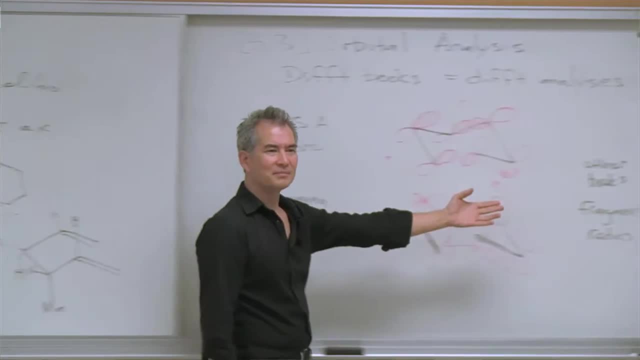 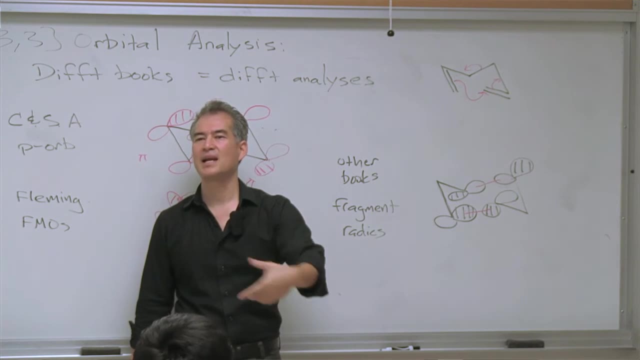 face of the other. I kind of like this depiction because it's simple And because when we talk about rearrangements I'm going to say three, three sigmatropic rearrangement and I want you to focus on what's going on with the faces of those three atom fragments. So I kind of 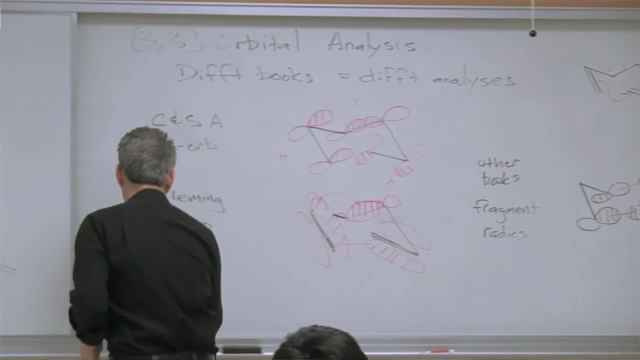 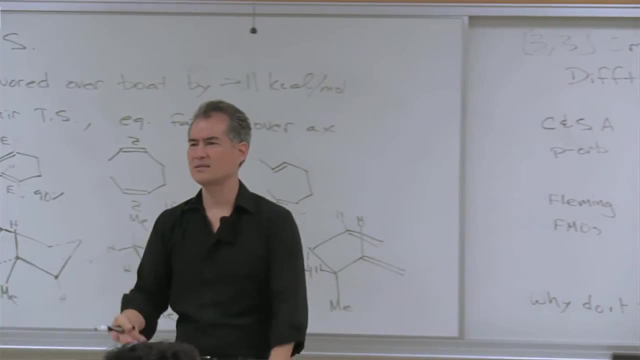 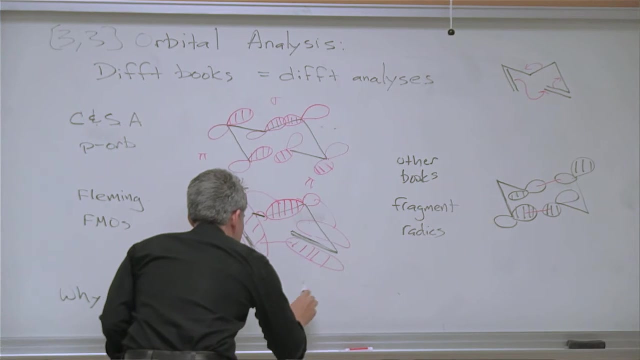 like this. So, overall, why would you do these kinds of things? And the only reason that you're going to analyze these- the orbitals here and the phasing- is because you want to know whether the two fragments are acting anterofacially or suprafacially. 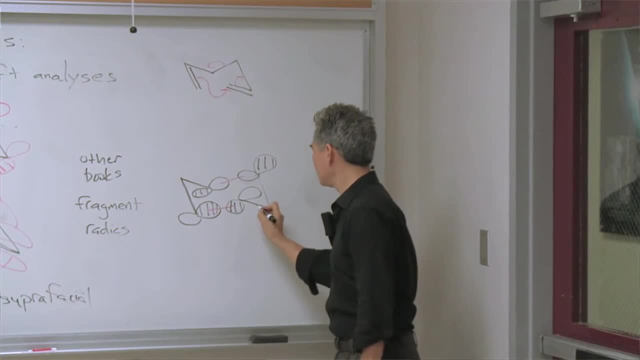 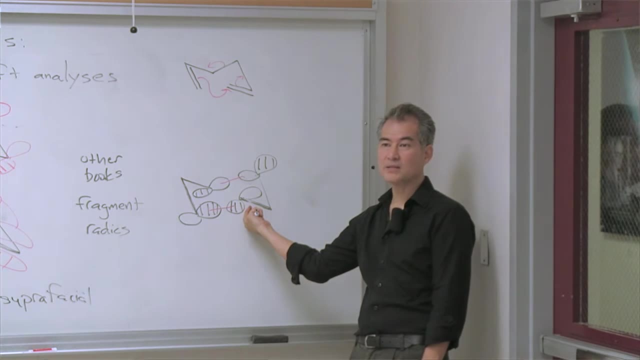 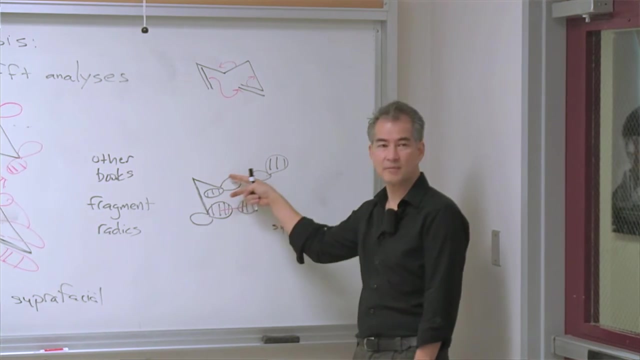 So here, both of my bonds and I- maybe it's- I don't know if that's obvious from my drawing here- but both of the bonds are coming from the bottom face of this aloe fragment And that's suprafacial, And this other fragment. both of the bonds are coming from the top. 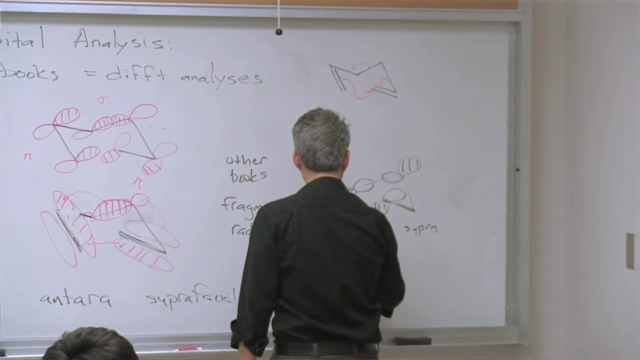 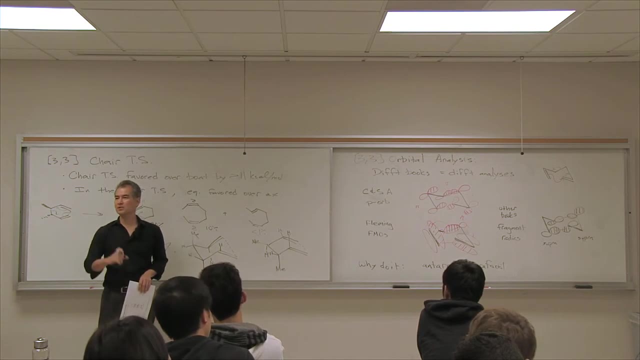 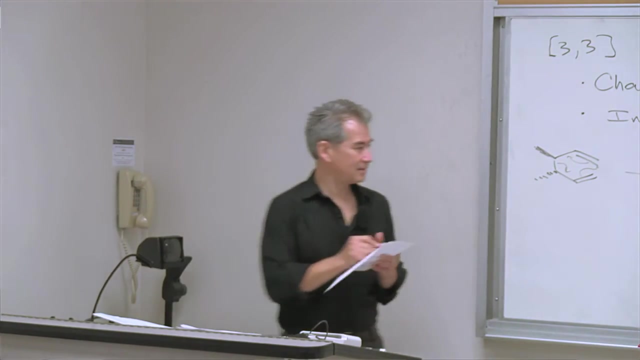 face of that one That's still suprafacial. So this would be a suprafacial, suprafacial process, And that's not always the case. In a minute, I'm going to show you some cases where you'd have to dream up some pretty weird transition states in order to access anterofacial. 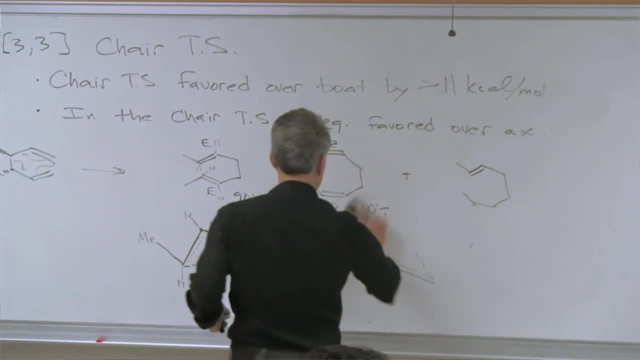 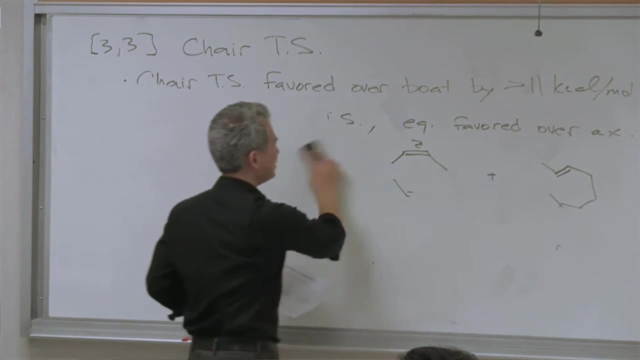 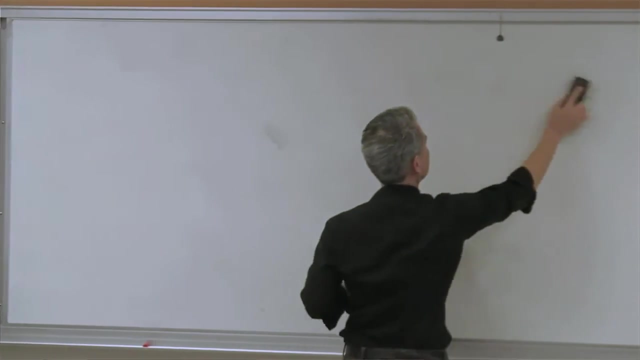 geometries. OK, I kind of like that. third, because it seems simple, There's less stuff we have to draw on the paper, Right? If it's a 3,, 3 sigmatropic rearrangement, well, let me just draw a 3 carbon aloe fragment. OK, The utility of this suprafacial, anterofacial business. 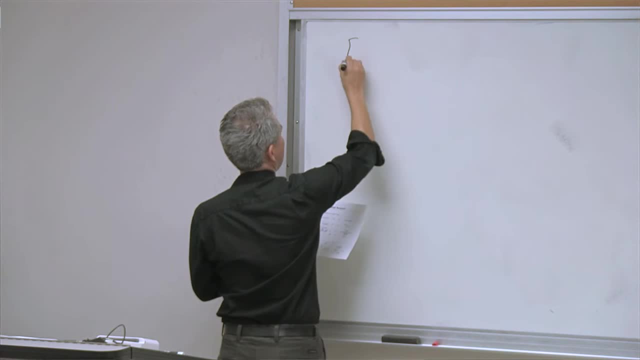 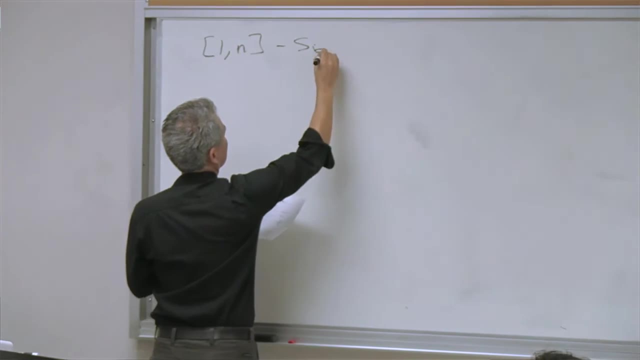 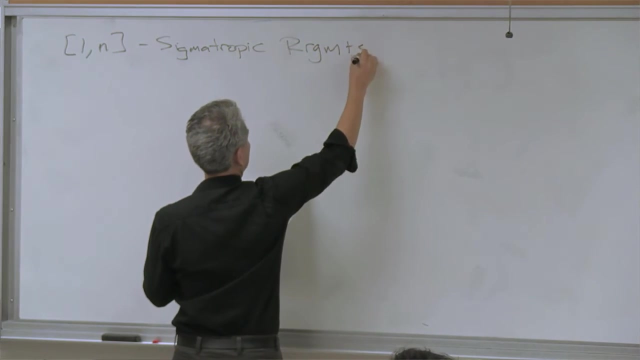 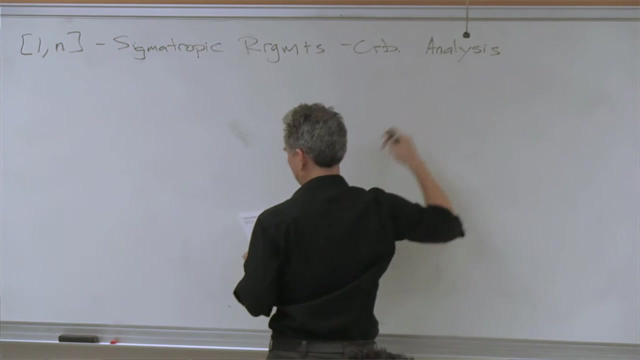 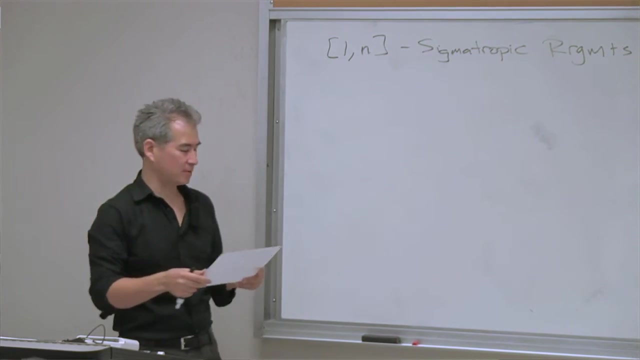 I think it'll help if we draw out some, oh some, 1N shifts. I'm just going to use that little integer number or whole number. So 1, 2 shifts, 1, 3, 1, 4, 1, 5, 1, 6.. Let's talk about those. 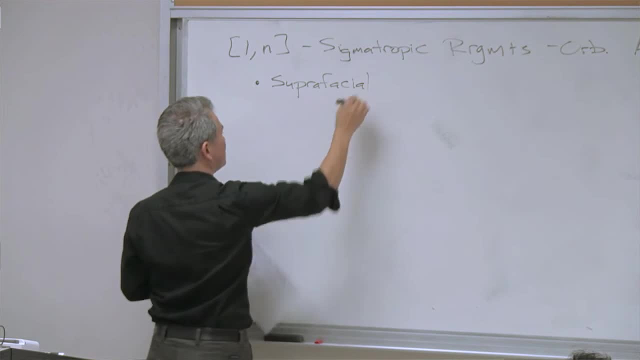 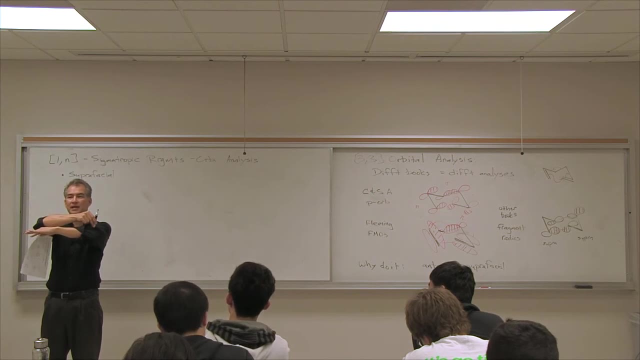 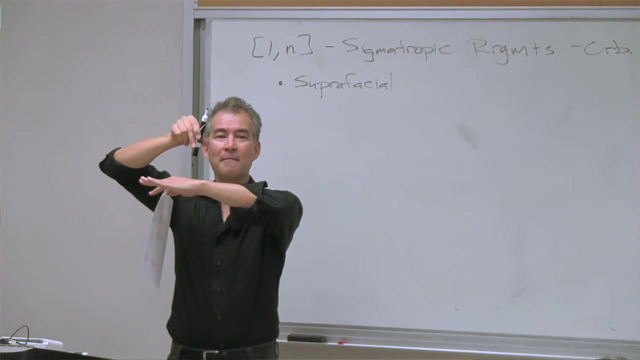 Everything is easy to envision when you talk about super-facial processes. I've got some sort of substituent on the top face and it just moves to a different atom on the same face. that's easy. It's much harder to envision some process where a group is sticking up and then magically 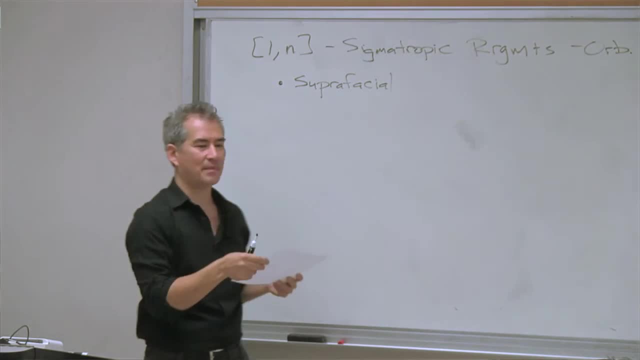 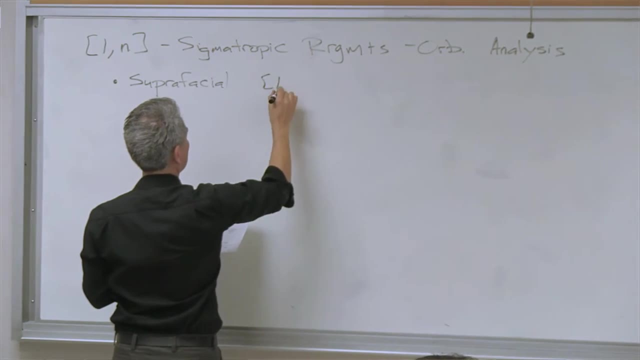 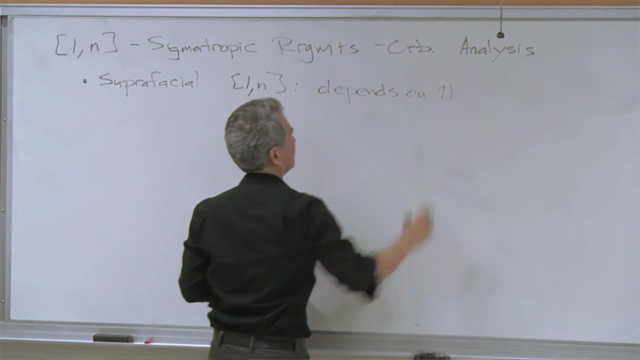 or, mystically, it somehow ends up on the bottom face. That's a lot harder to imagine. it's not impossible. Actually, super-facial ought to be easy. but what you'll find is it depends on whether it's 1, 2,, 1, 3, or 1, 4,, 1, 5,, et cetera. 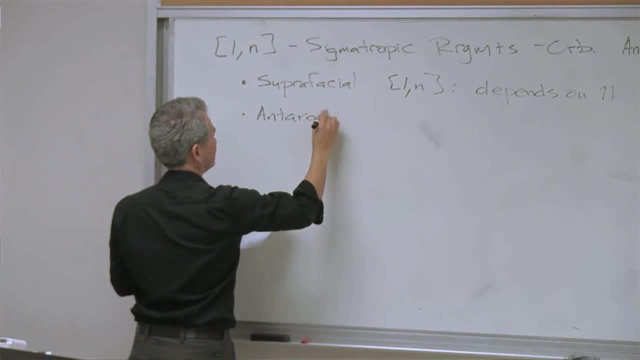 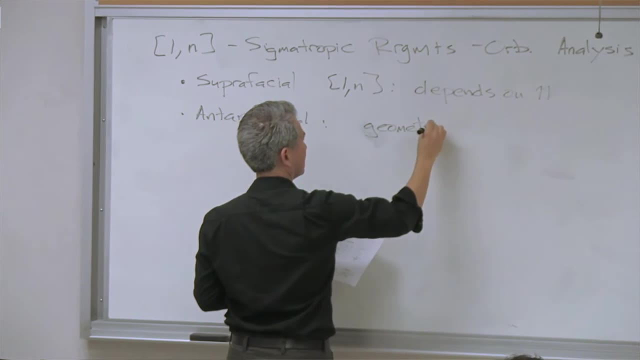 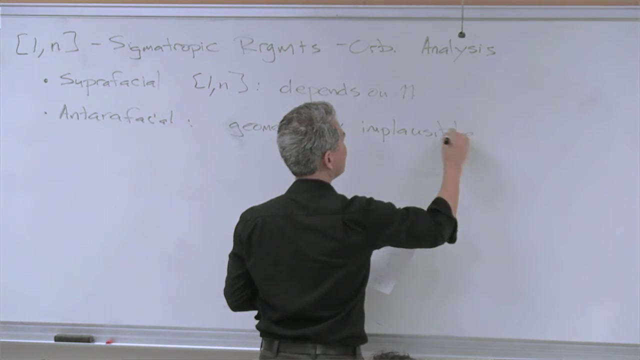 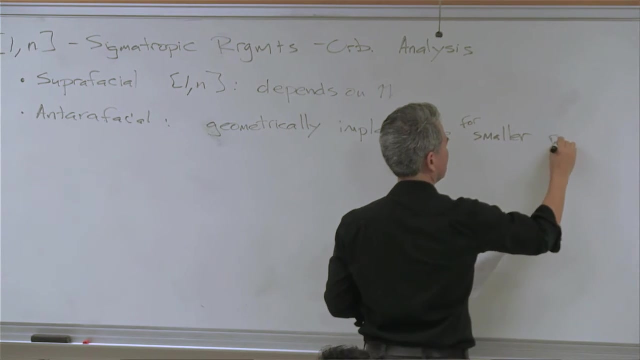 And tera-facial conceptually. Okay, let's go back to the first one, Okay. Okay, It ought to be implausible for typical ring sizes- I'll call them smaller rings, but are generally implausible if you talk about normal ring sizes like five-member transition states. 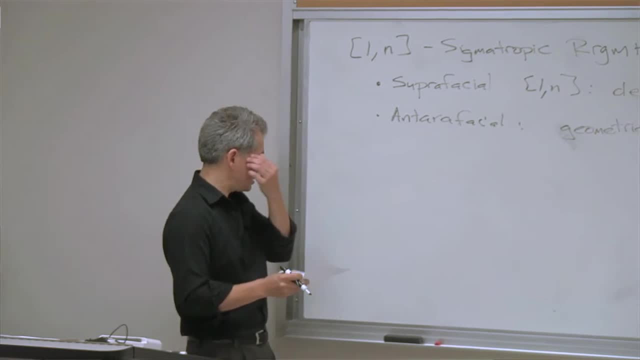 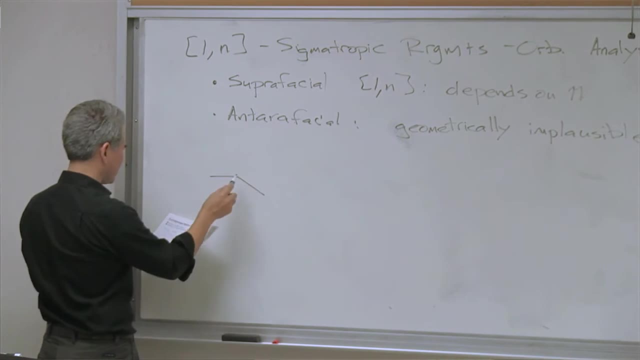 or six-membered ring transition states or four-membered ring transition states. Let's try to take a look at some shifts. I'm going to draw a kind of edge on. I'm going to try to draw a kind of edge on. I'm going to try to draw just propene, just so I can envision. 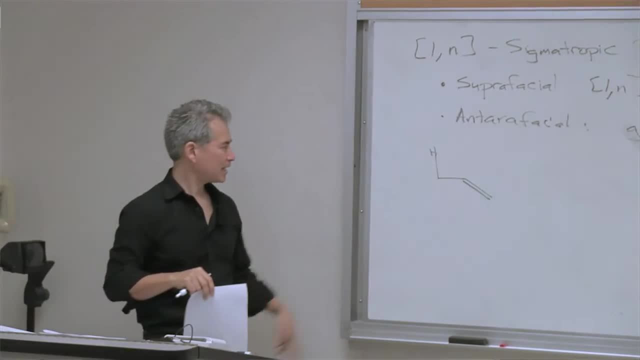 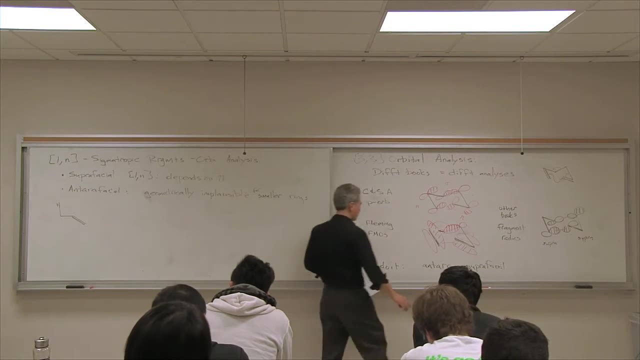 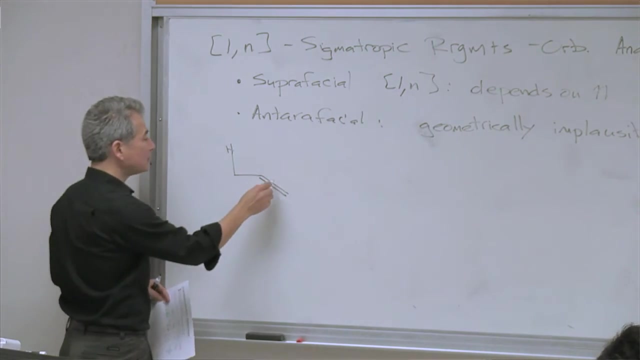 that there's two faces to this propene molecule And I've got a carbon-hydrogen bond here, And so what's the chance for this carbon-hydrogen bond to simply skip over and tautomerize, right? It doesn't matter whether this is carbon-carbon or carbon-oxygen, right? 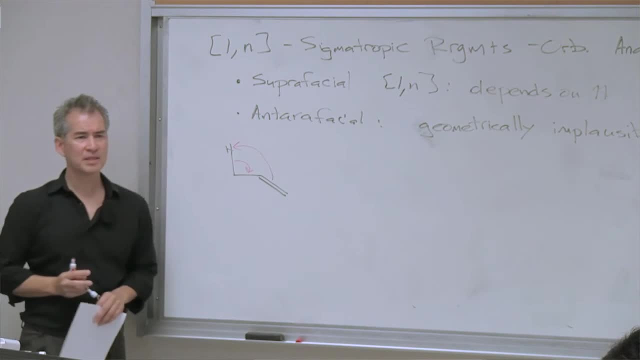 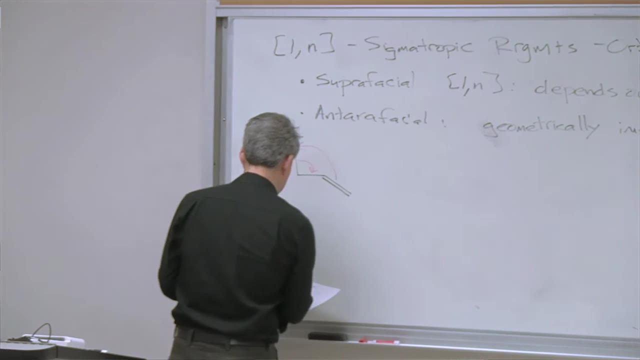 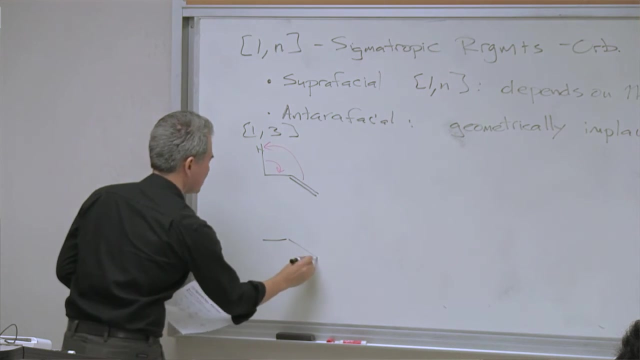 If I put an oxygen atom there, is this possible for me to tautomerize keto to enol in one step? Let me go ahead and draw the orbital analysis here. So this would be a 1, 3 shift. And if I draw the orbitals for an allofragment, for the three-atom fragment? here's the orbital. 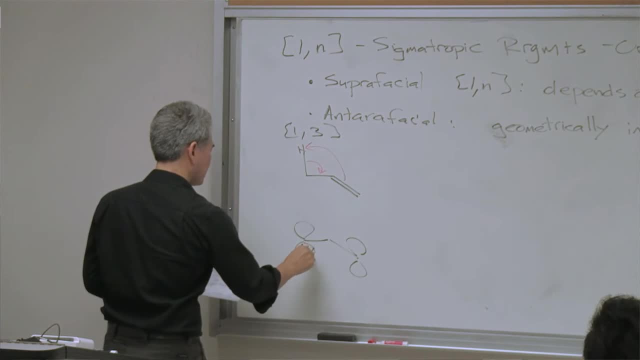 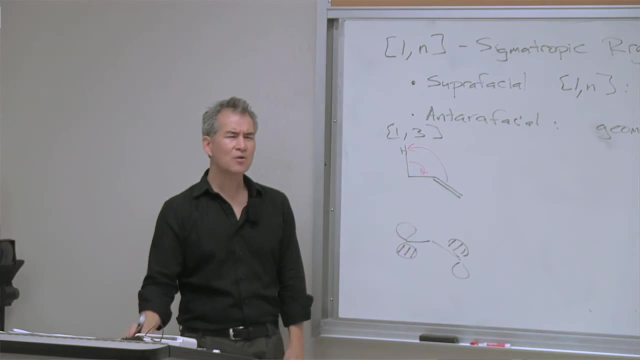 analysis for a three-atom fragment. Remember, there's a node in the middle. One end has got the hash on the bottom, The other end has the hash on the top. What does the orbital look like for a hydrogen atom? Well, remember. 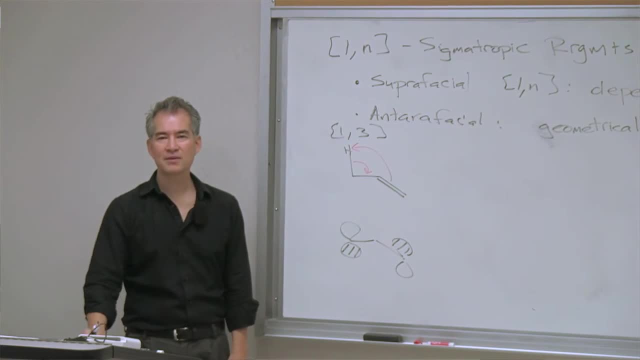 There's no p orbital. There's no p orbital. There's no p orbital. You have to draw orbitals with a hydrogen atom. Hydrogen atom is a first row, It's just S You've got like a 1S orbital. 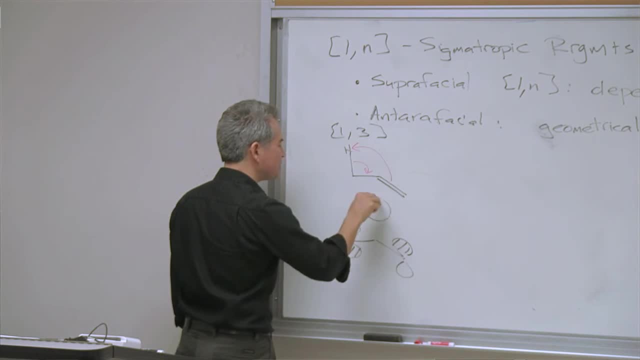 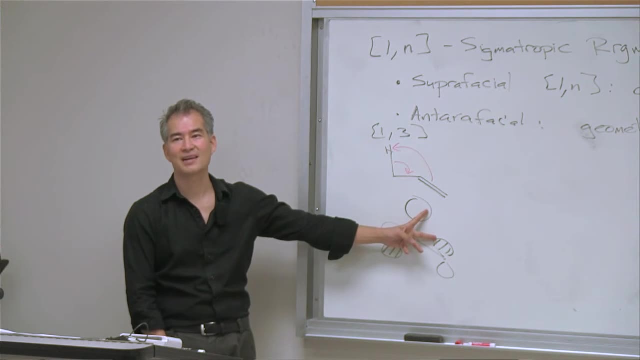 So let me draw a 1S orbital. It's not SP3 or SP2.. That's all I get. So, yeah, you can have a bonding interaction here, but you cannot simultaneously have a bonding interaction with the top face of an allofragment. It violates principles of orbital symmetry. There is no way you can simultaneously have bonding on the top face here and on the top face on the other end. That's why, whether it's propene or a carbonyl compound, you can't have 1,, 3 superfacial shifts with protons. 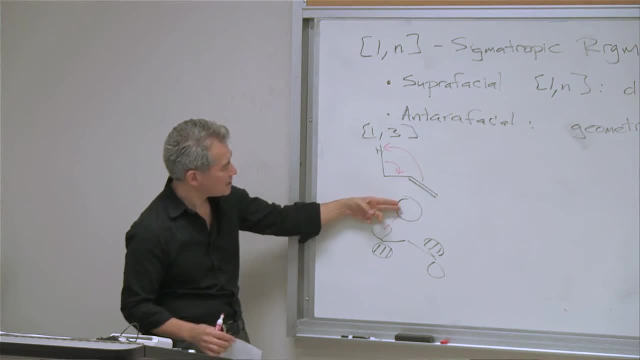 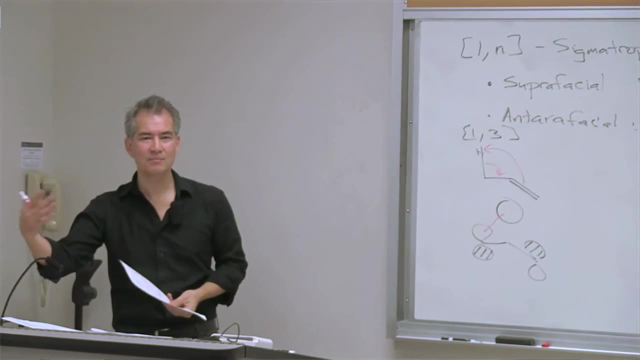 You'd have to. the only way you could have some sort of 1, 3 shift that's paracyclic is if it is, if the proton started on the top face and somehow ended up on the bottom And quantum mechanically. maybe there's some tunneling argument. 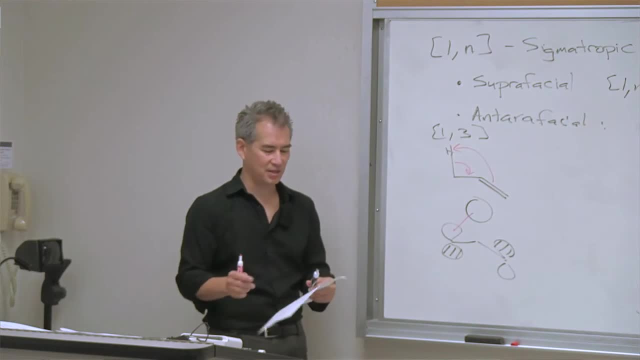 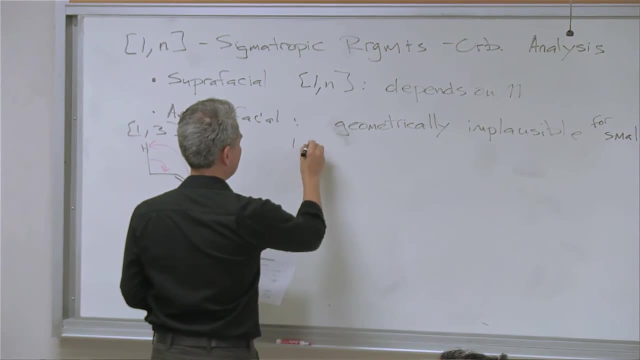 why that might be possible, but that's just not plausible. to draw 1, 3 shifts of protons, That's completely implausible. OK, let's take a look at another example, at a 1, 5 shift. So now I'm going to struggle here. 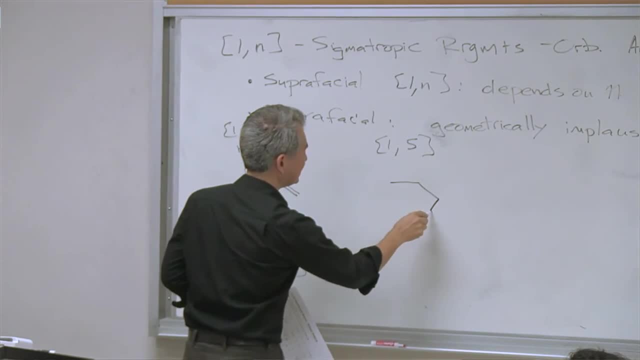 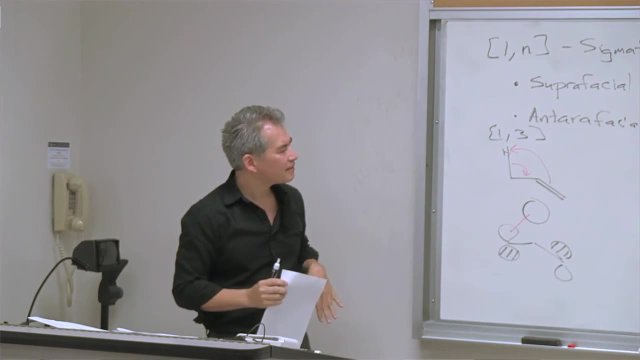 to draw a pentadienyl system, kind of like a bit part of a benzene ring edge on, because I want to be able to see the different phases of that And I want to be. I've got a 5 carbon system and I want 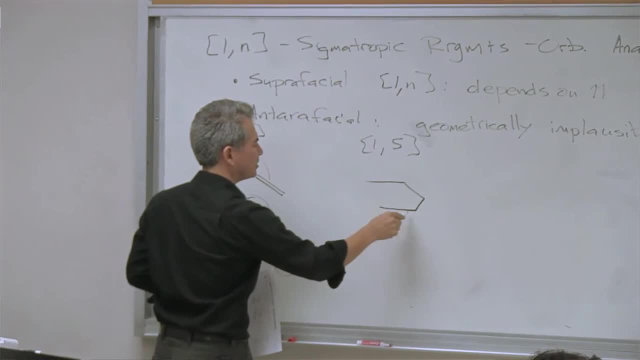 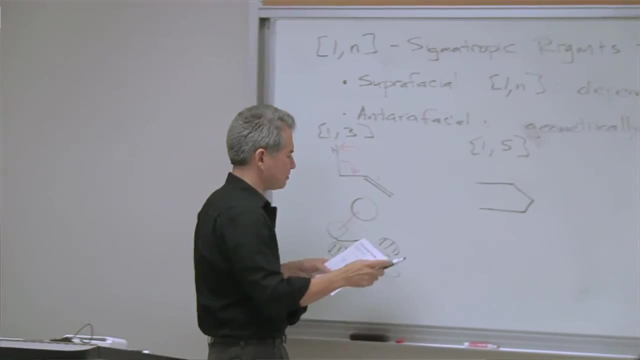 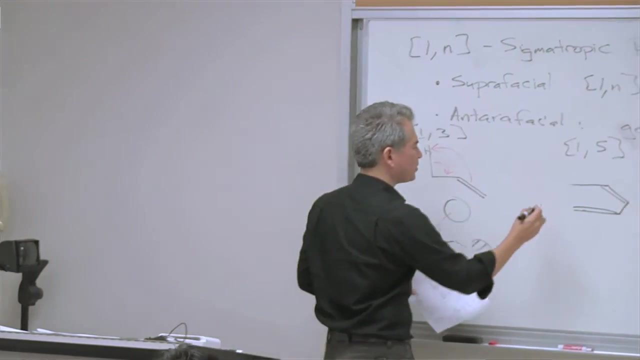 to try to envision. maybe if I make these bonds longer it'll make it more, more three-dimensional. OK, So there's a 5 carbon And let me add some double bonds so it looks like a pi system here. And then, on this last carbon, I'm going. 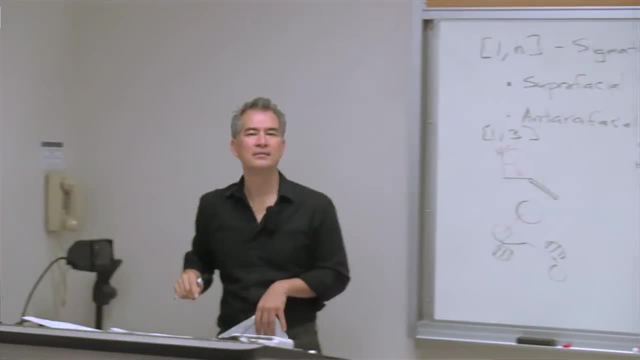 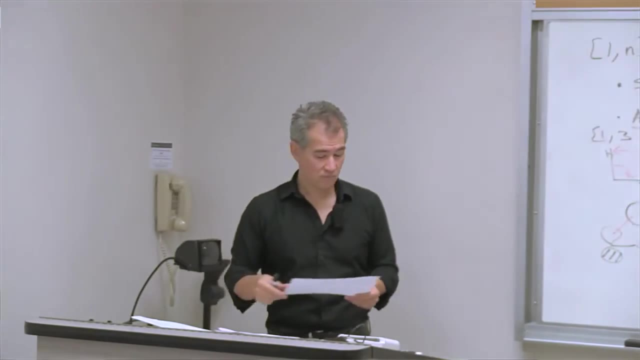 to have a hydrogen atom poking onto the top face, And so let's try to imagine: is it possible for the H to jump over here onto this other carbon atom? And so maybe what I- I mean I could draw the arrows, That's, that's no problem. 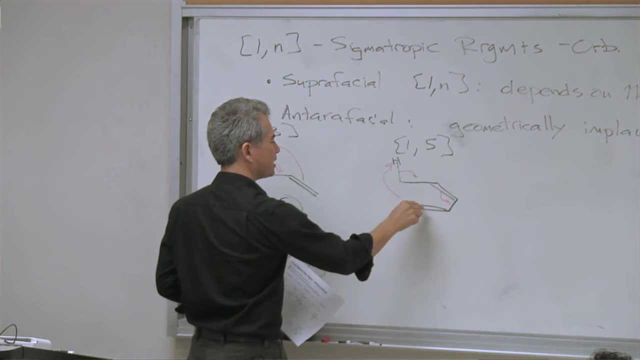 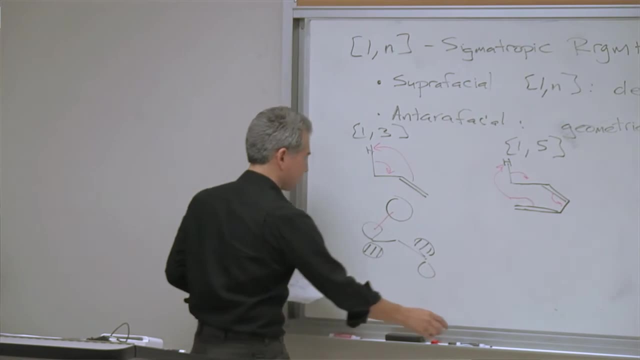 It's easy to draw arrows to make it look like: right, I'm going to protonate this, this double bond here, Double bond on the end. It's always easy to draw the arrows. The question is: does, does the orbital symmetry work out? 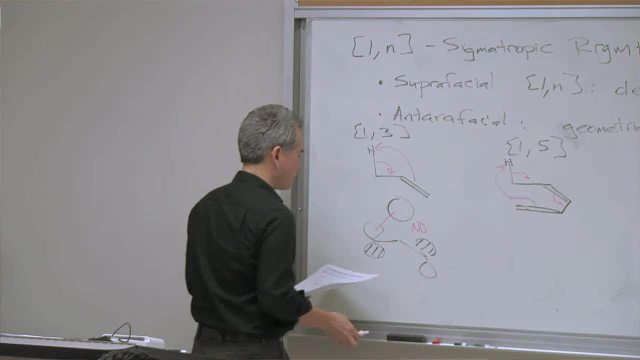 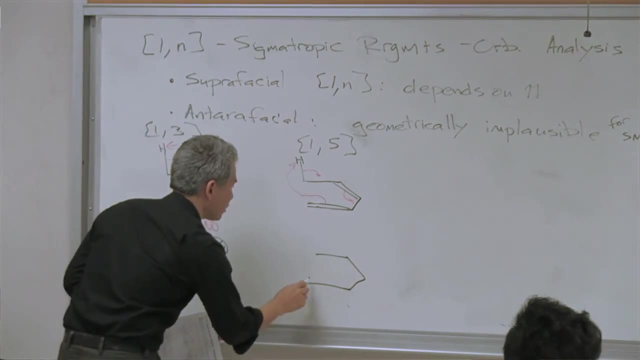 I'm going to just write no here. Right, The the 1, 3 shift we we agreed was just no way that was going to happen. Let me try to sketch out the orbitals for a right, this is just hookle theory again. 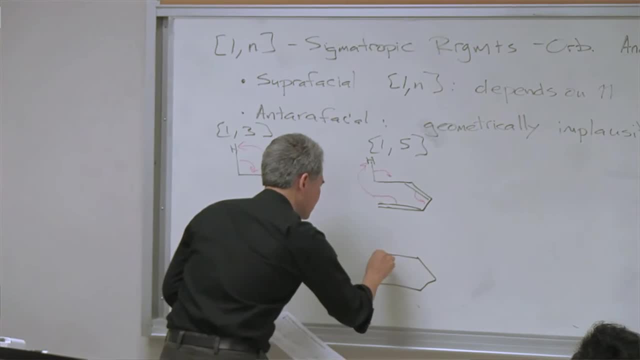 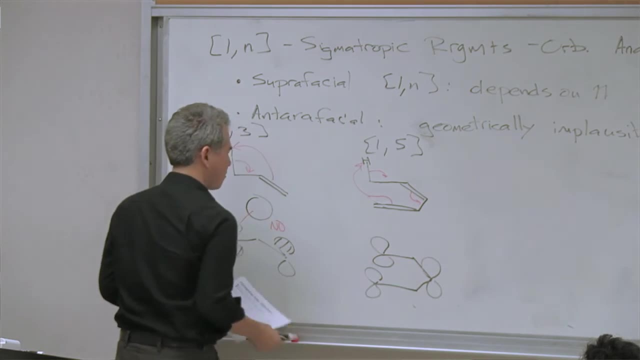 What does a pentadienyl system look like? Well, it looks like this. If I draw the orbitals for a pentadienyl system, there's two nodes here: at carbon 3. At carbons 2 and 4.. 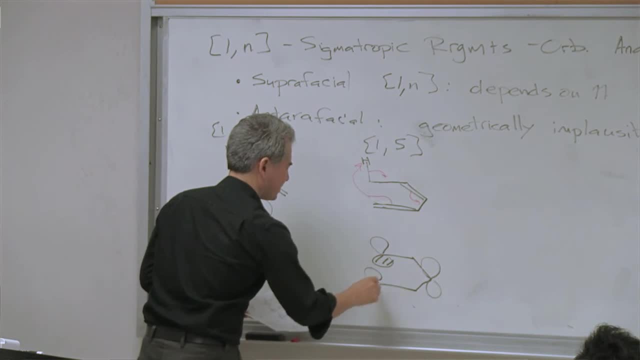 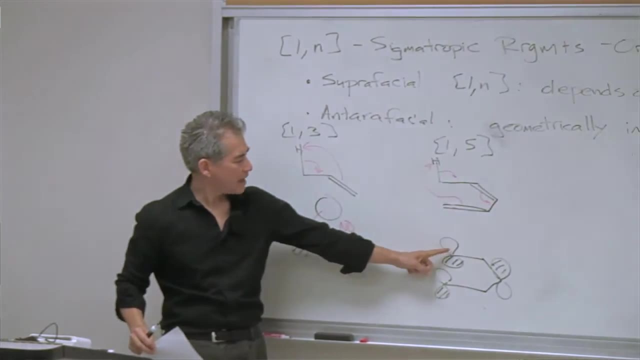 And if I look at the phasing for a pentadienyl system, the phasing on the two end carbons- and that's the ones we really care about- is the same. Hashed on the bottom, hashed on the bottom. 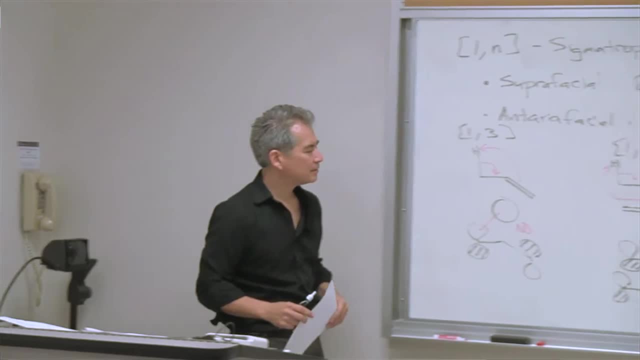 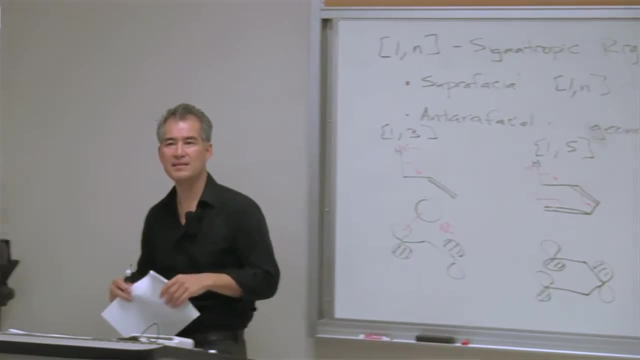 Or you could arbitrarily draw it the other way, hashed on top. So with a pentadienyl system with a 5 carbon pi system, the two end carbons have the same phasing on the top, And that means if I draw some sort of a hydrogen atom. 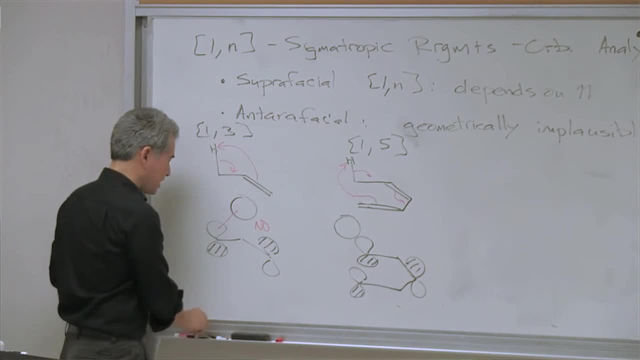 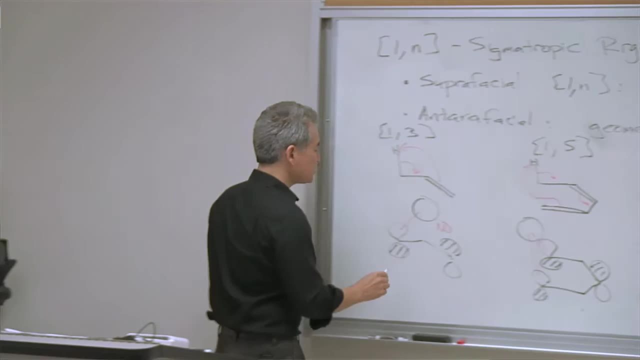 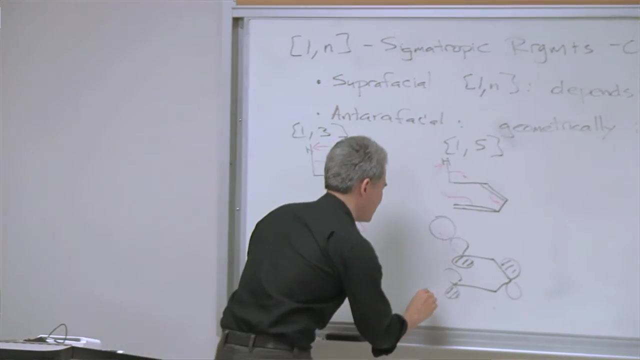 there's a 1s orbital Right, I can simultaneously have bonding between both of the end carbons on the same face. So the super facial shift for a 1, 3, totally implausible. But a super facial 1, 5 shift on the same face, no problem. 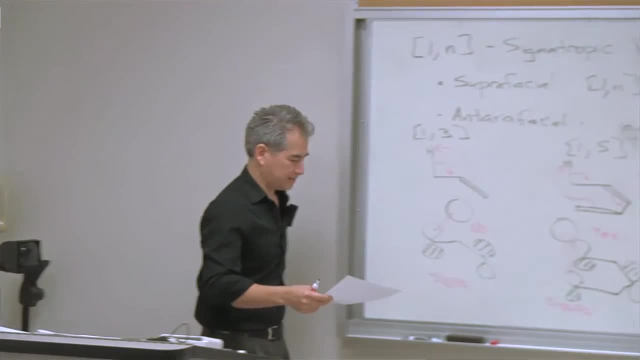 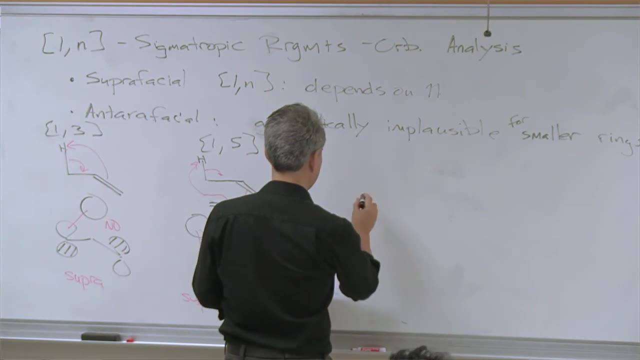 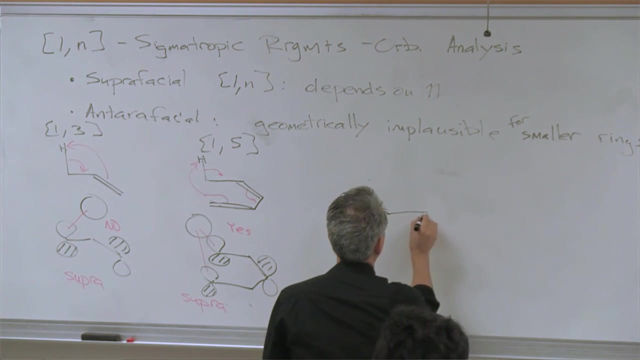 1, 5 shifts are very common in organic chemistry. OK, Let's keep going, And I'm going to have to. now you have to try to draw a stop sign here. I think is the easiest way. I'm going to try to figure out how to draw edge on. 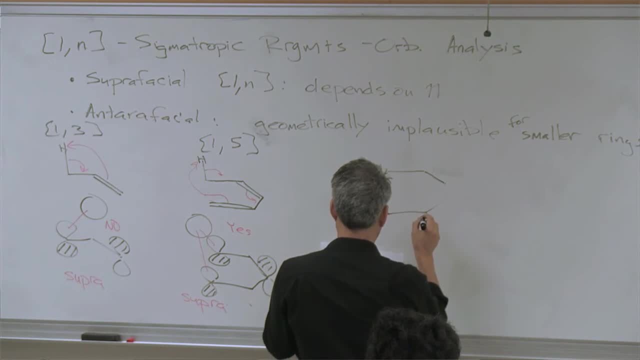 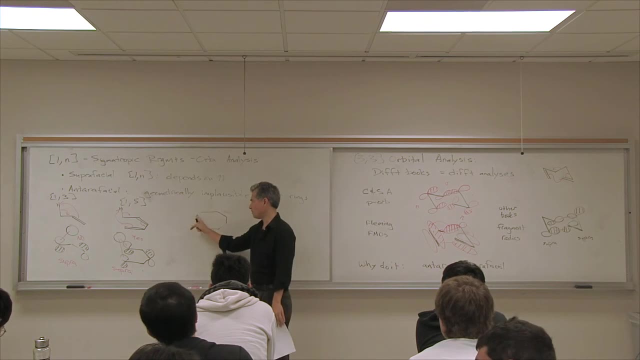 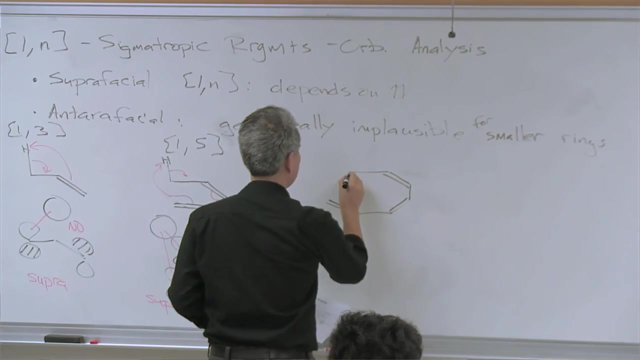 Now do I do this? I'm going to try to draw 7 carbons. It's like an 8 membered ring. I'm just going to leave off one of these carbons, OK, And then, once again, I'm going to have this H atom jutting. 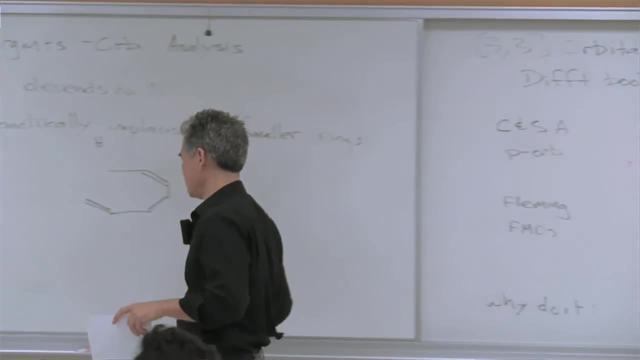 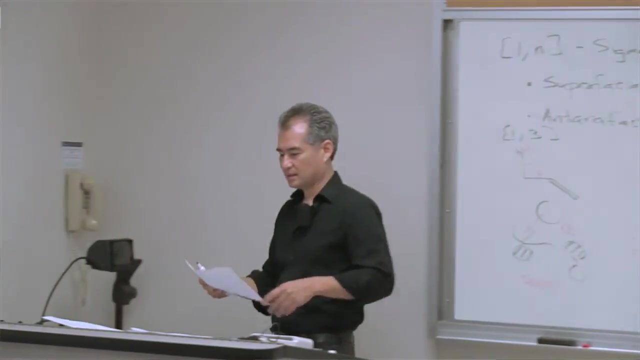 up on the top face so we can try to envision. is it possible? right The arrow? it's easy to draw arrows here. Look at this, just as easy as it was before. But the question is: is that allowed by principles of orbital symmetry? 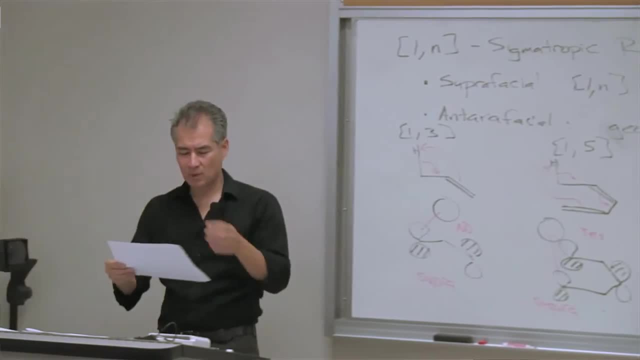 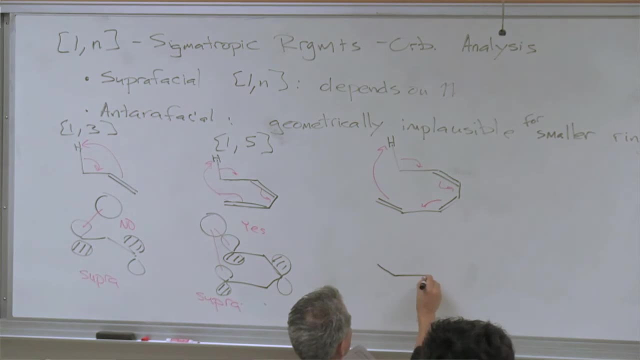 So let's, we've got a 7 carbon system here, And what do the orbitals look like for a 7 carbon system? We haven't spent a lot of time talking about that, So I'm going to try to draw a 7 carbon system. 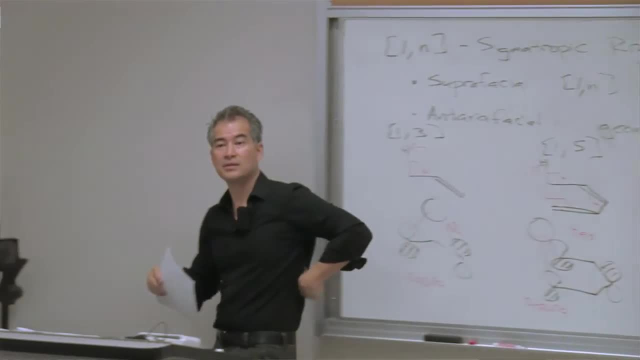 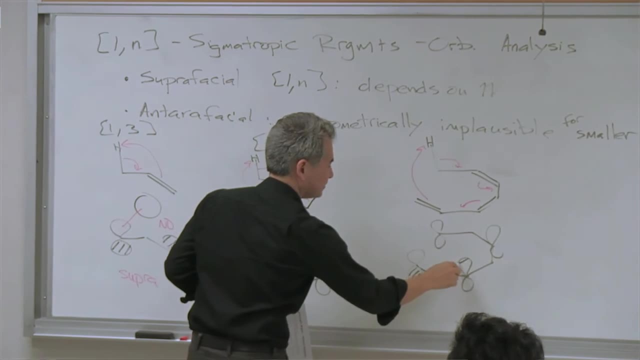 So there's 2 nodes over here with the 5 carbon system, There's 3 nodes with the 7 carbon system And if I draw this orbital phasing, it has to flip. There's 1 node, it has to flip again. 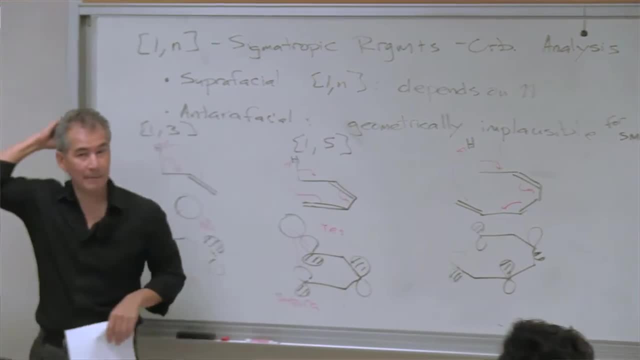 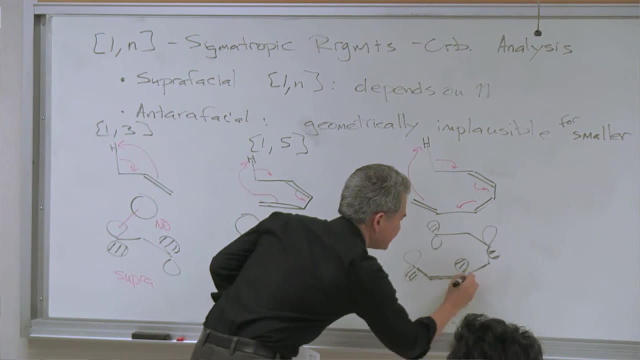 Now the hashing is on the bottom, it has to flip again, And now the hashing is on the top. Let me try to make this sort of look 3 dimensional here, Because again I'm trying to get this idea of faces across. 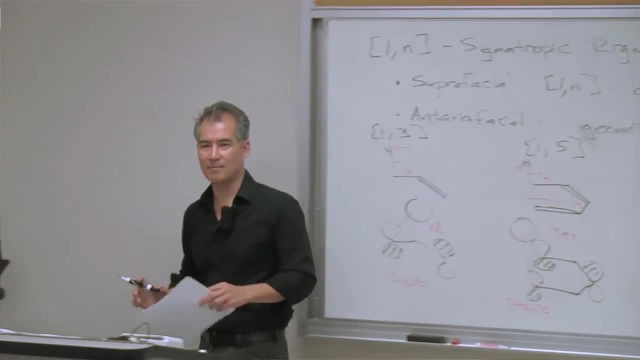 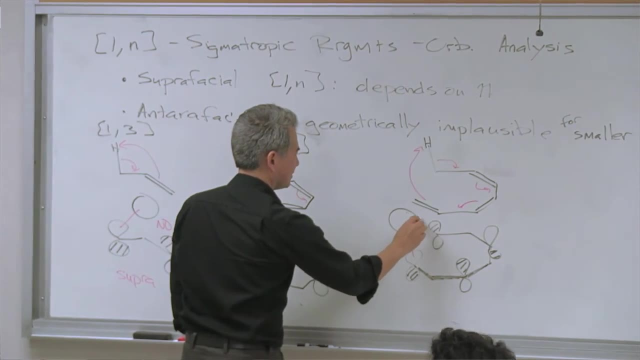 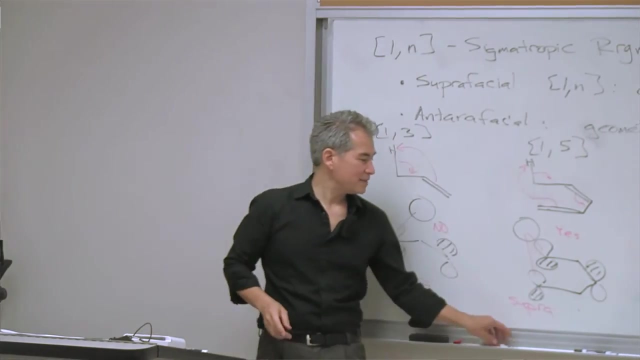 So if I draw a hydrogen atom here, right, you can see the problem. If my hydrogen atom has bonding interactions over here, you can't. I'll just write: no, you can't have a superfacial shift. There's no such thing as a superfacial 1, 7 shift. 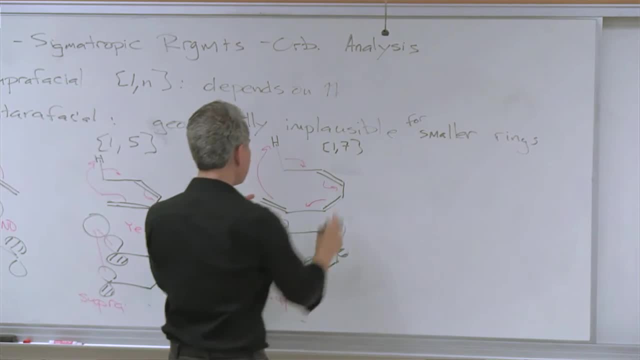 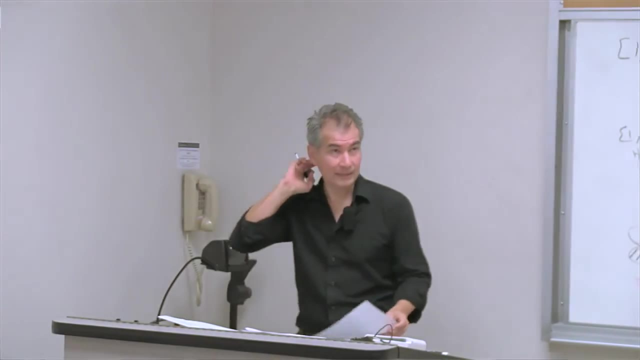 That's totally implausible. But that's not to say that you couldn't shift this, like maybe there's some way to shift this to the bottom face And we'll talk about that shortly. Actually, let me give you some examples now of how. what are the practical implications of this? 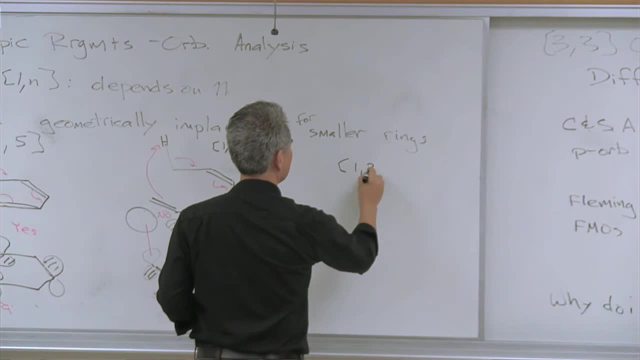 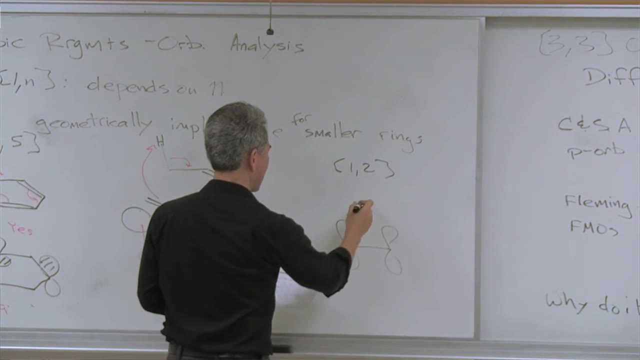 I guess I'll just mention a 1, 2 shift is allowed by orbital symmetry, the carbocation shift. And how do I draw a carbocation shifting? So if I draw a carbocation shift or a methyl group shifts, I would draw the 2-carbon system like a pi bond. 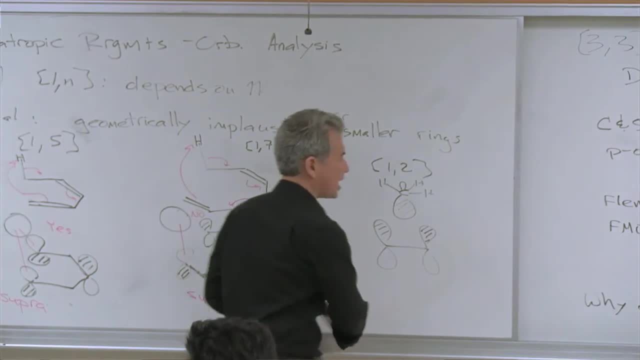 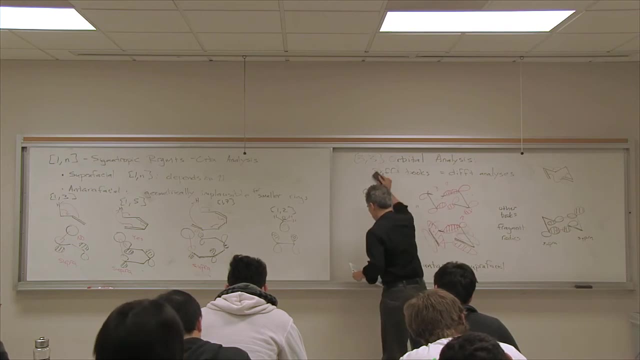 A 1, 2 shift is allowed by orbital symmetry. It doesn't matter whether it's a hydride shift or an alkyl group shifting. the orbital phasing works out for a 1, 2 shift. Okay, so what's? what are the implications of this? 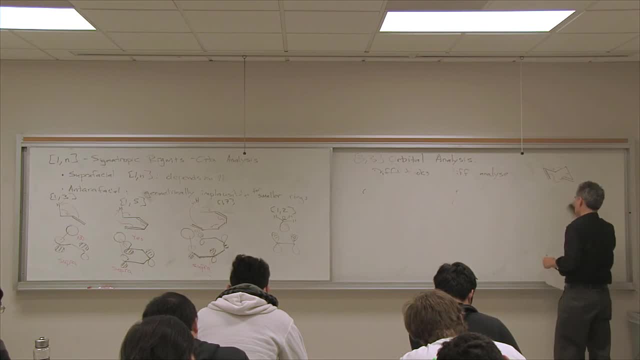 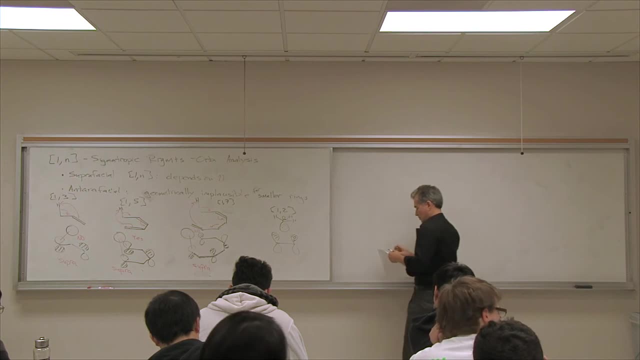 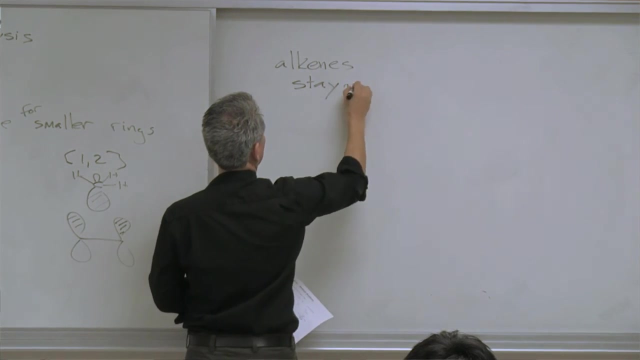 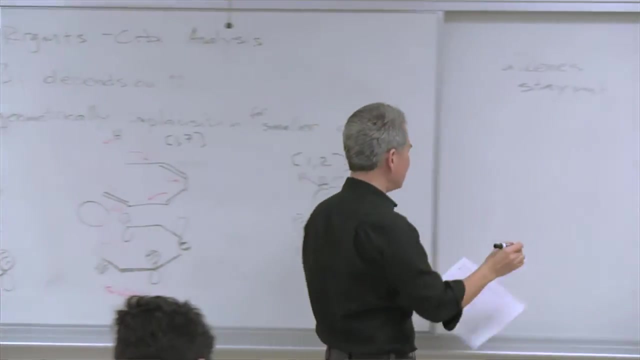 of this allowed Versus not allowed, or we would say symmetry allowed Versus symmetry, disallowed or forbidden. Okay, so here's one very simple implication: Thank God 1, 3 shifts are not allowed super facially. 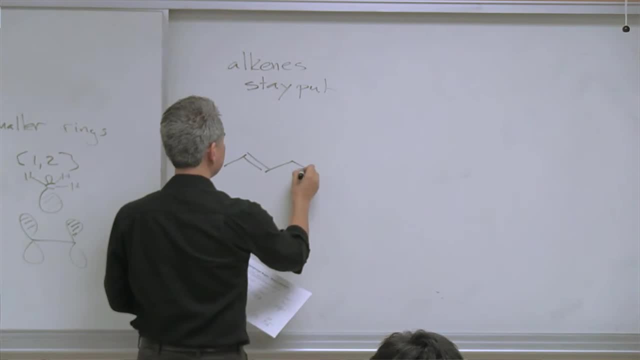 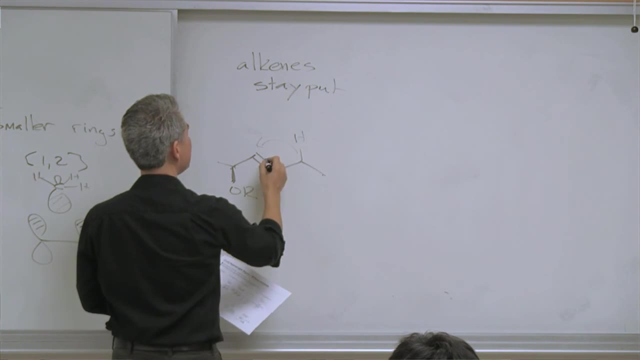 So if you go into the lab and you synthesize some sort of an alkene Like this, you do not have to worry that these H's are going to dance around on your on your substrate and shift the bonds around. Alkenes stay put. 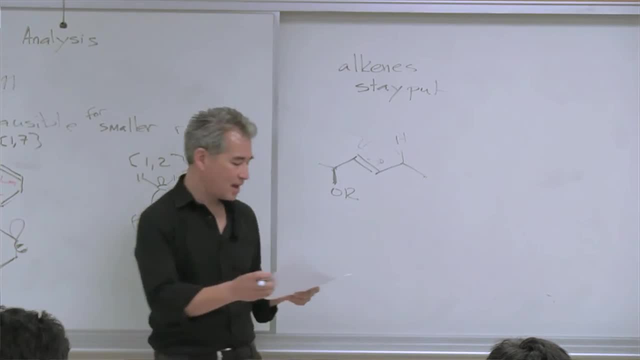 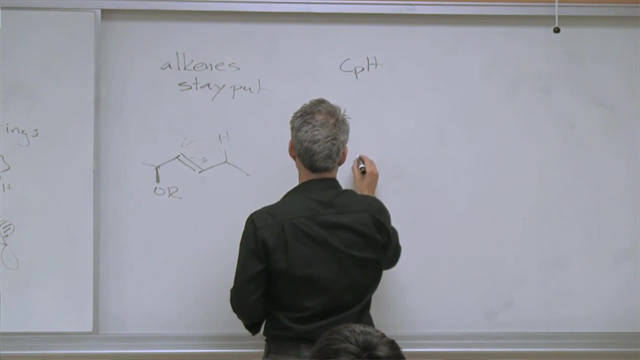 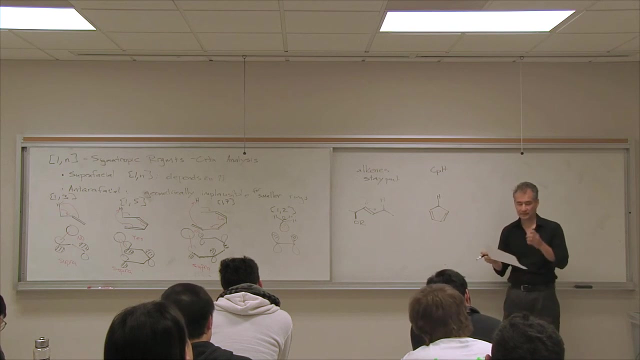 They don't just float around because of 1, 3 shifts. That's totally implausible. The alternative is that cyclopentadienyl systems with H's on them are extremely sensitive to isomerization, And so if you, you know, you're going to have to, you know. 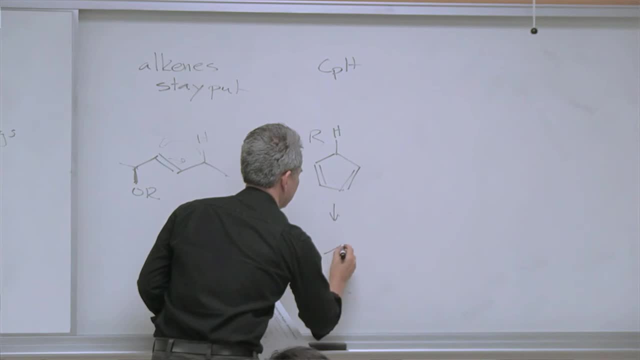 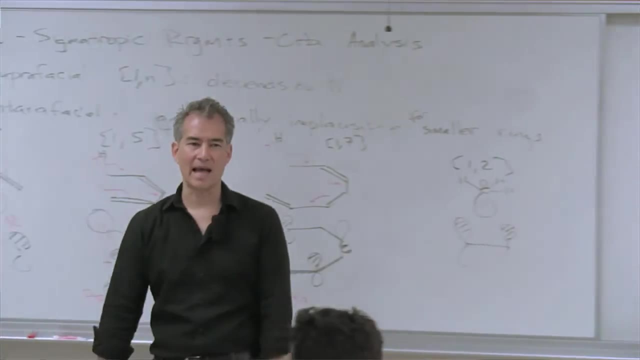 you have some sort of an alkyl group there, you'll find that what happens is that that alkyl group will seem to move to different positions. It's not the alkyl group that's moving, it's the proton. Now it's possible that, if your conditions are basic enough, 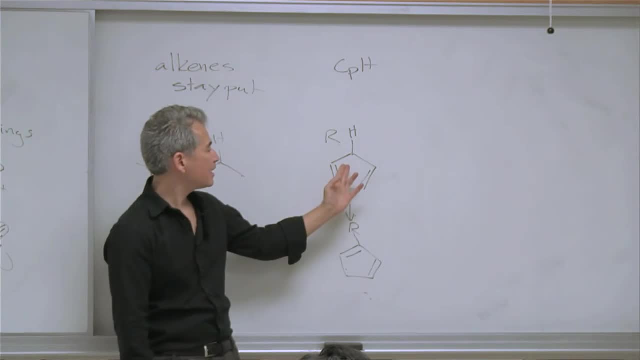 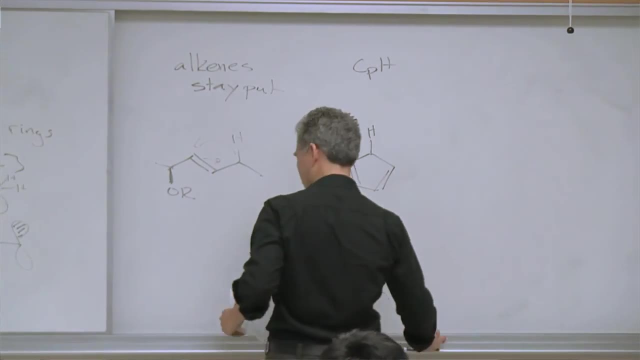 you're deprotonating and reprotonating. This is very acidic, But even if you take all the base out, the H's will still migrate around through 1, 5 shifts And I'll draw the arrow pushing there. So it's very tricky. 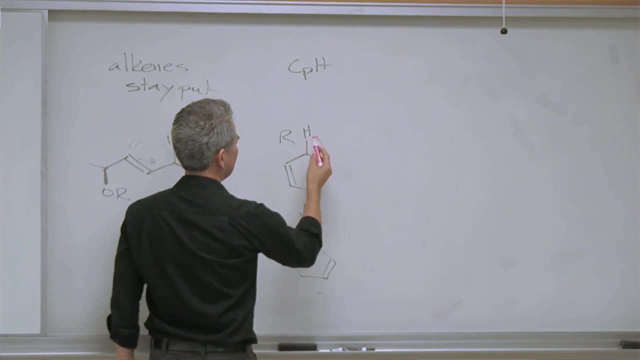 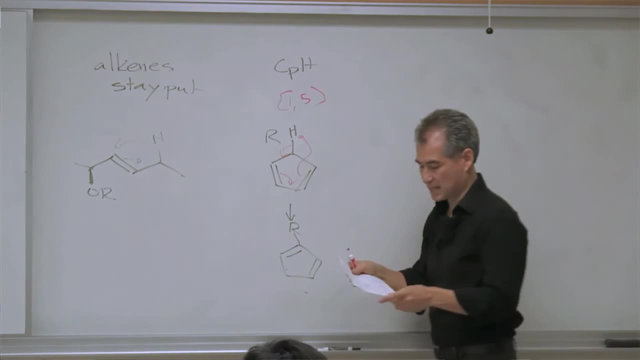 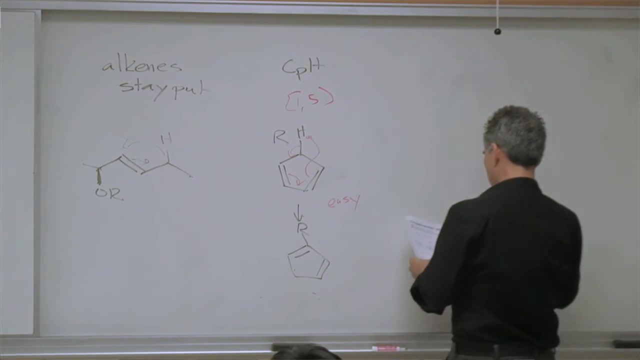 It's tricky to work with cyclo substituted cyclopentadienyls because they undergo 1, 5 shifts with great facility. So that's very easy. I'll just write easy here. I don't have a, I'm going to struggle here to draw. 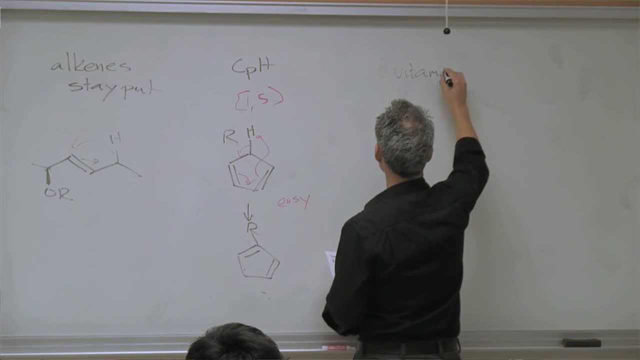 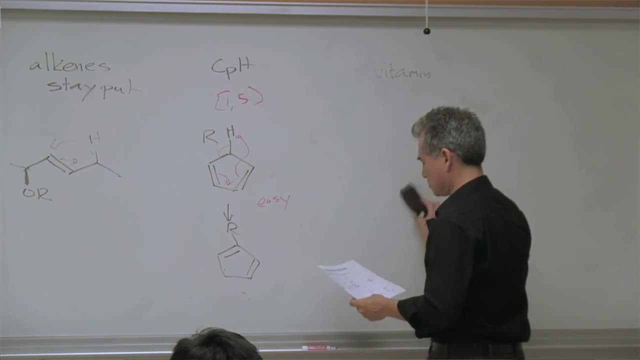 And I'm going to try to draw. let me you know, the easiest way to do this is to draw an eight-membered ring. So let me just draw an eight-membered ring And I'm going to erase one of the bonds in my eight-membered ring. 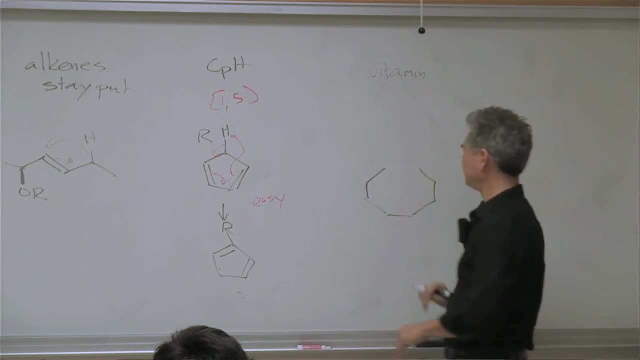 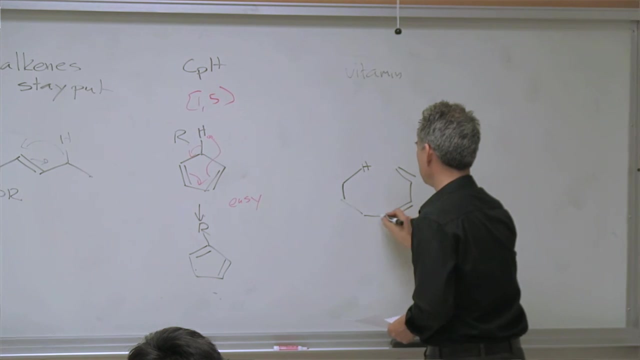 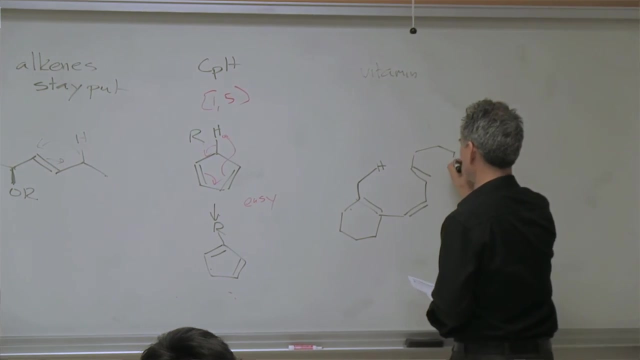 And here's the bond I'm going to erase up on top here. So vitamin D biosynthesis involves this kind of a 1, 7 shift And I'm not going to draw all the rest of the stuff here, but it's part of a steroid-like. 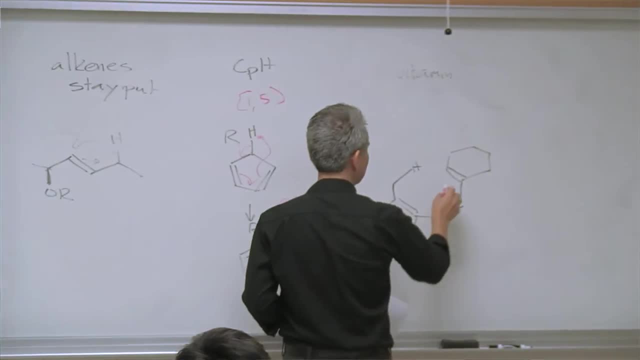 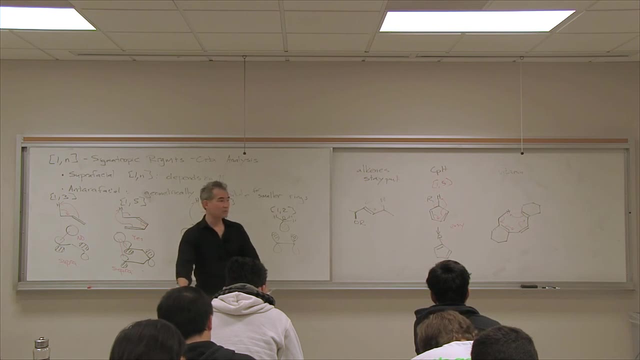 system And if this is really going through a 1-7 shift, it can't be suprafacial. We all agreed that it cannot be a suprafacial shift. This is facile at room temperature. this is happening in your body, even in the dark. 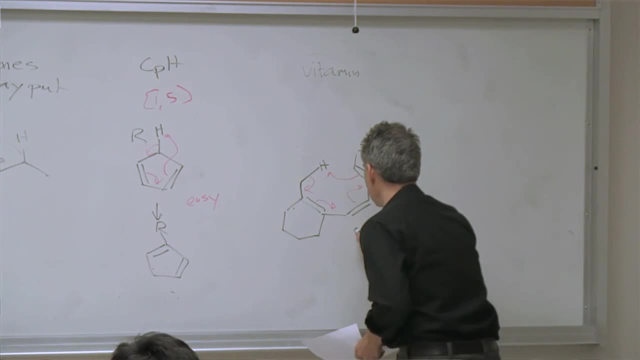 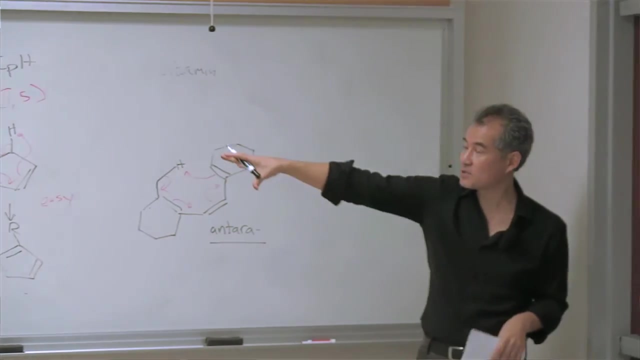 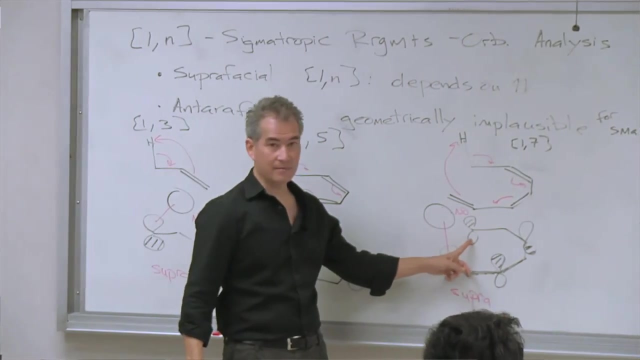 And what I'm going to try to do is try to draw what's happening here. This has to be anterofacial Because the 1-7 suprafacial shift is not allowed. If you want this H to start on the top, face over here, it has to end up on the bottom. 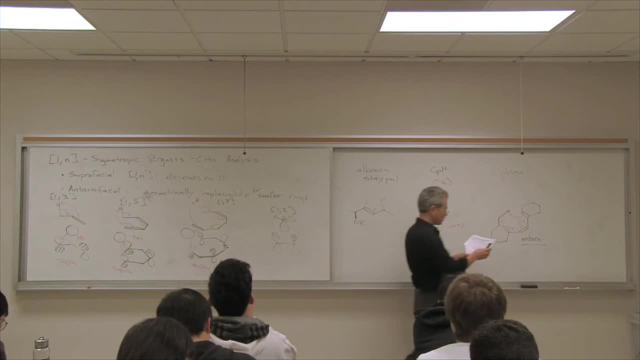 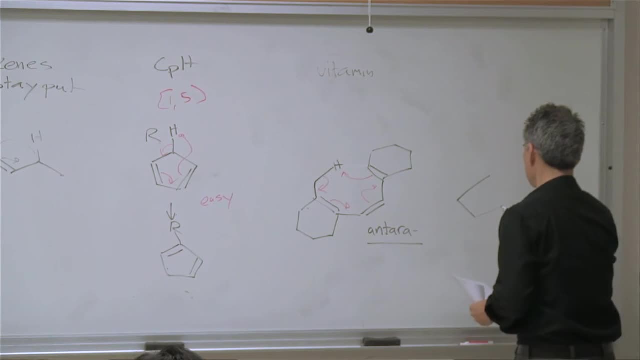 face when it's done, And so you have to try to imagine some sort of a helical type. gee, how do I do this? Let me try to draw this here. I'm going to draw this like allofragmater And I'll have two atoms going up. 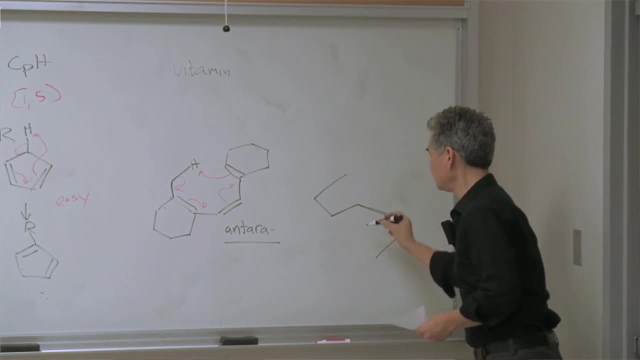 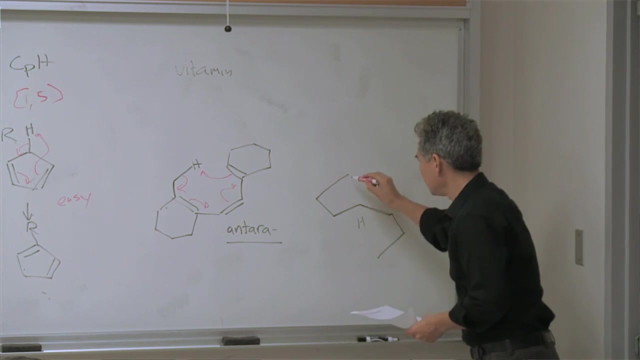 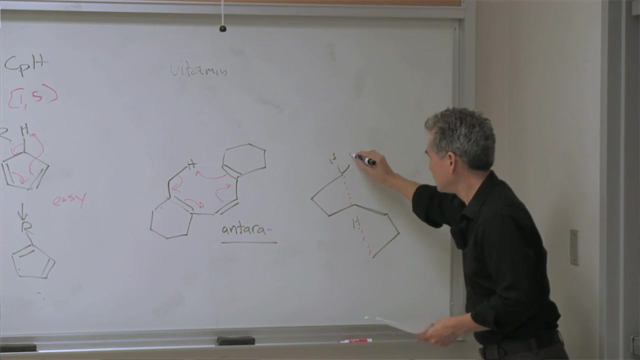 One up here, Two atoms going down there. So that's my seven atom system, And then I'll try to imagine some sort of an H atom in between here, And in the transition state it starts on the bottom face of one of these carbons and 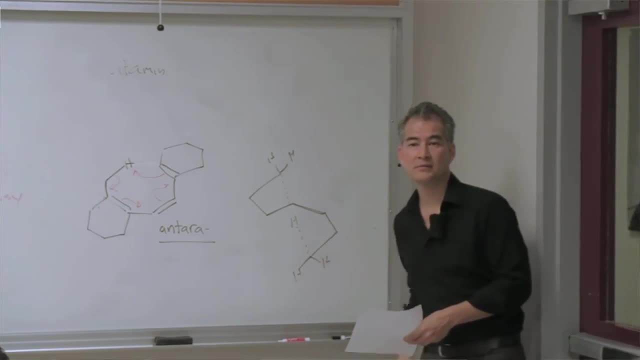 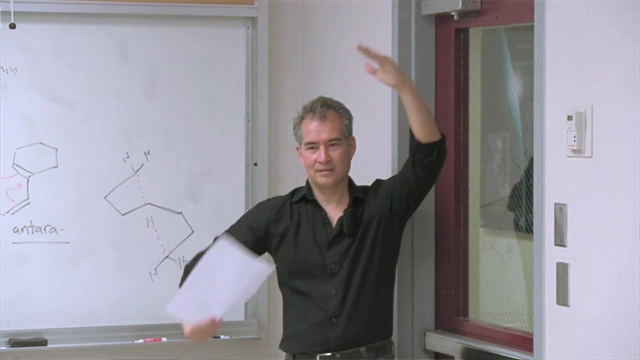 it has to end up on the top face And that's possible. So there's this sort of helical structure in which the bottom face of this and the top face of this- So 1,7 shifts- are allowed, but it's got to be inter-facial. It's possible you could have larger shifts, but as you get to larger ring sizes- 1,9, 1,8, it's just entropically hard to bring those ends together. This is kind of 1,7 is kind of unusual. 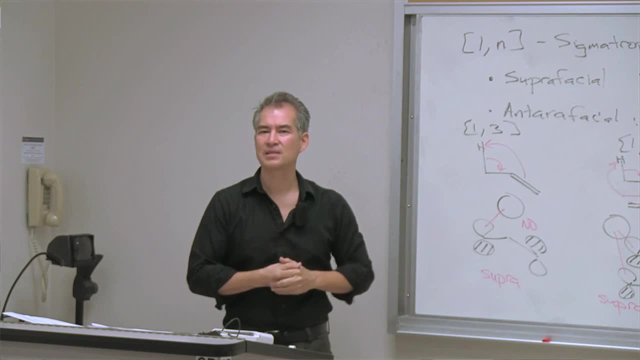 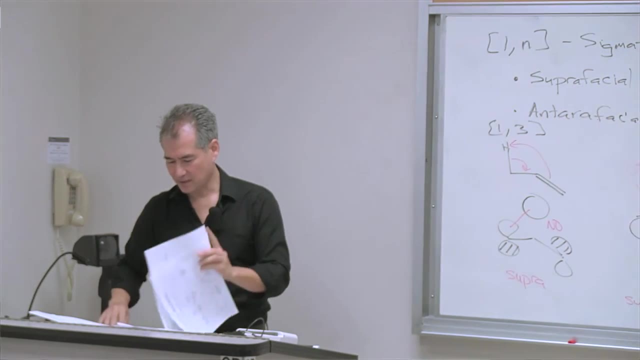 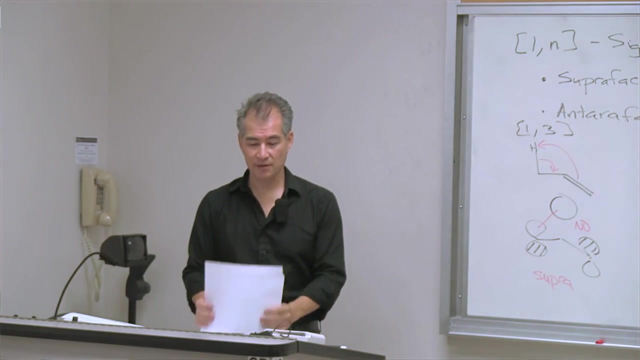 because you typically don't have the ends of one of seven carbon systems poised close to each other. OK, so we'll try to finish up the sigmatropic stuff on Friday And our exam will cover through sigmatropic, through all the paracyclic reactions. 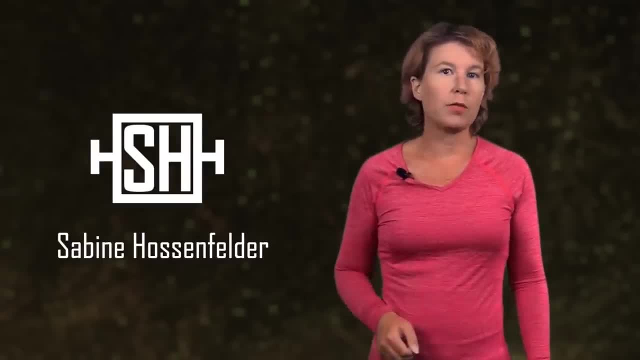 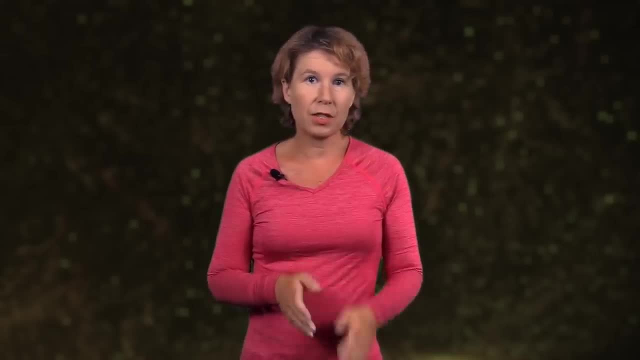 In the past months, we've talked a lot about topics that receive more attention than they deserve. Today, I want to talk about a topic that doesn't receive the attention it deserves. That's a twenty years old anomaly in neutrino physics, which has been above the discovery. 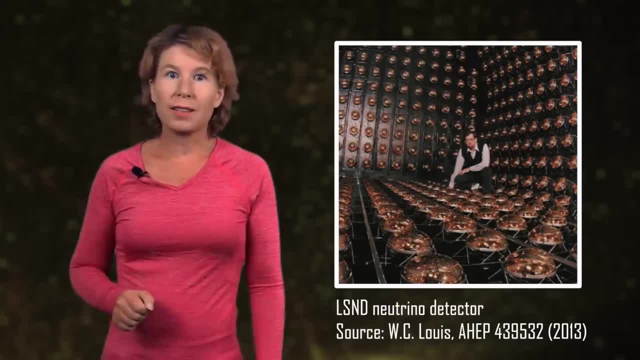 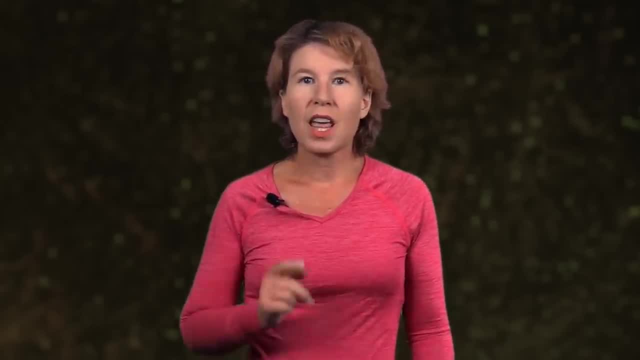 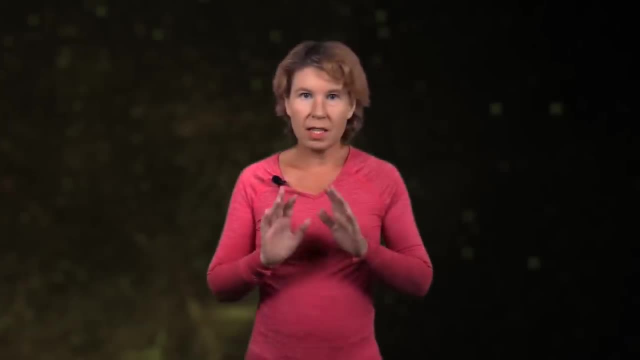 threshold since 2018, but chances are you've never even heard of it. So what are neutrinos? what's going on with them and what does it mean? That's what we'll talk about today. I really don't understand why some science results make headlines and others don't. For example, we've seen loads of headlines about the anomaly in the measurement of the muon g-2 and the lepton anomaly at the large hadron collider. In both of these cases the observations don't agree with the predictions, but neither is statistically significant enough to count.